onslaught of AI started hitting the scene. Thank you for the introduction. We were there maybe four or five, six years ago when the onslaught of AI started hitting the scene. Thank you for the introduction. We were there maybe four or five, six years ago when the onslaught of AI started hitting the scene. 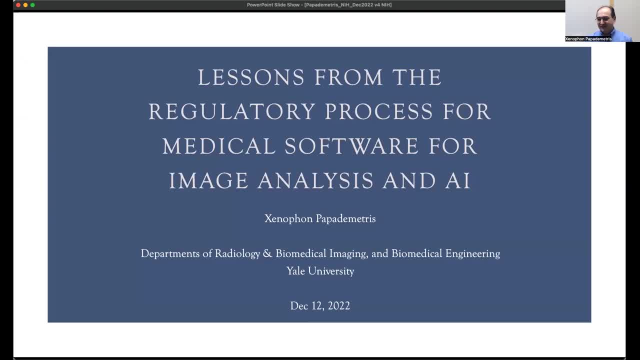 Thank you for the introduction. We were there maybe four or five, six years ago when the onslaught of AI started hitting the scene. I was a big part of the study sections- you know, small Business and business review grants- with Dr Stapler, the SRO, and I was a reviewer. So this is the title for the talk Lessons. 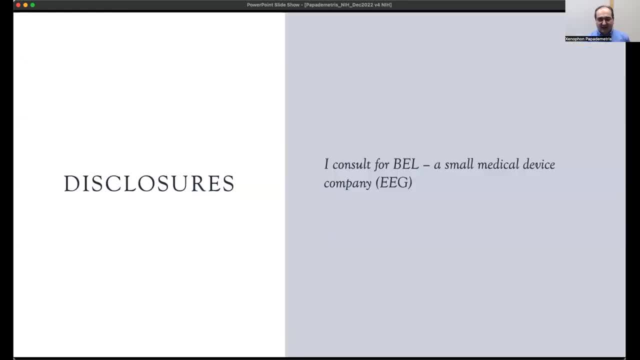 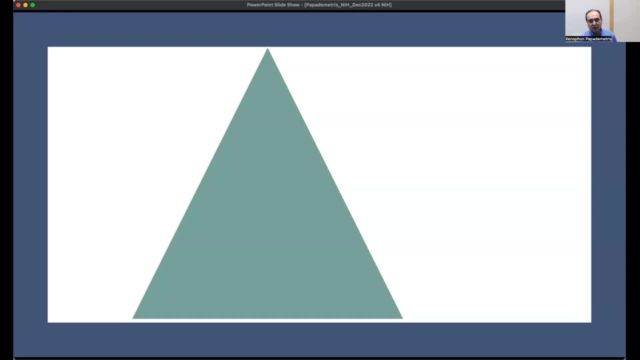 from the regulatory process for medical software for image analysis and AI. This is my disclosures. This doesn't relate to the talk, really, And let me tell you a little bit about what I'm trying to do with this talk. So we have a very sort of highly promising methods in 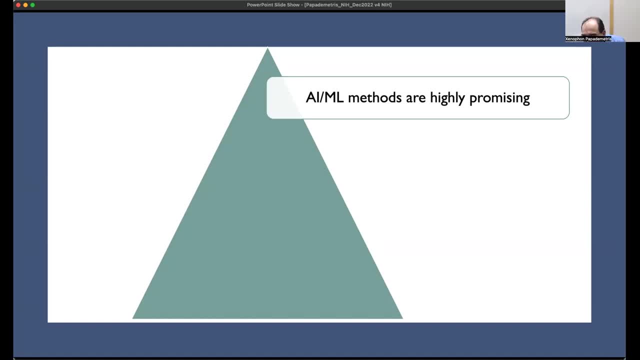 artificial intelligence and machine learning. Some of us have seen results that are better than anything we have seen. Being a scientist is an є performance. That's the whole point, and that's so important. there are some issues that are worrying us- me at least, and others in. 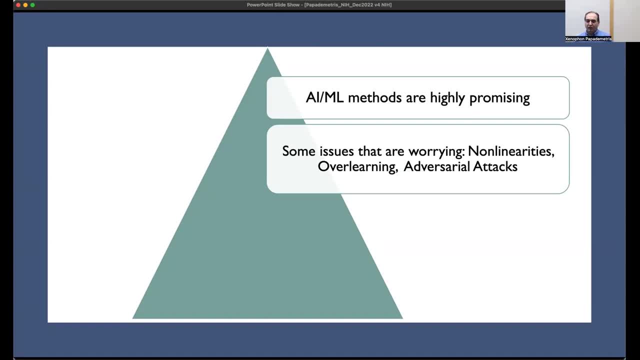 the field when it comes to the use of these methods. things like non-linearity, sober learning, adversarial attacks- all of those are related essentially, and the fundamental question is: how do we learn when to trust these results? we get some really good results, but can we trust? 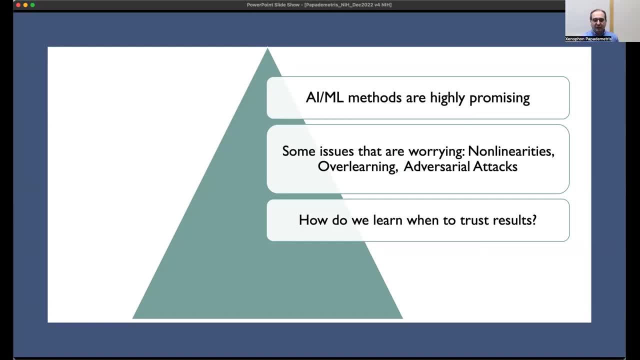 them? are these likely to be still good in a subsequent use? and what i'm going to try to do during this talk is to try to see if we can learn some lessons from the regulatory process for medical devices, medical software, and apply them to ai research and medical image analysis research. 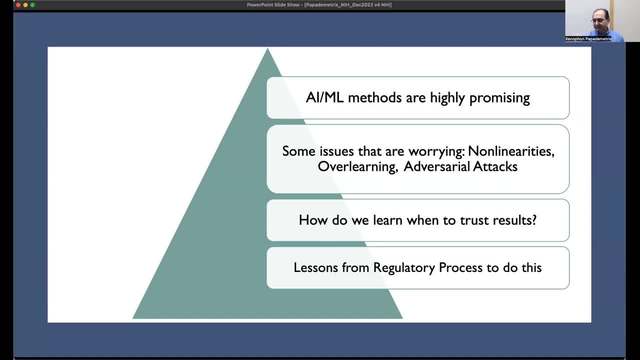 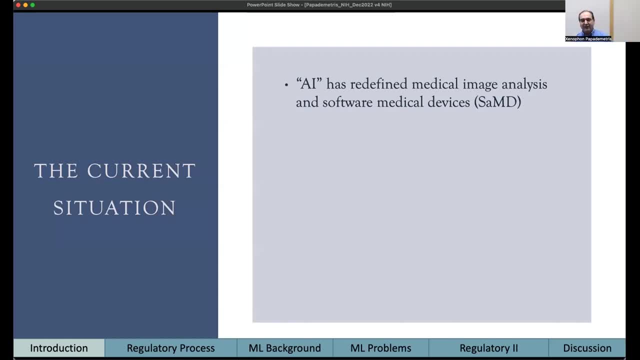 to help us understand how the process works. okay, so here's the current situation we're living in. ai- whatever this is, we'll define it in the next slide- has redefined medical image analysis and what has come to be known as software, medical devices or some. these are regulated software. 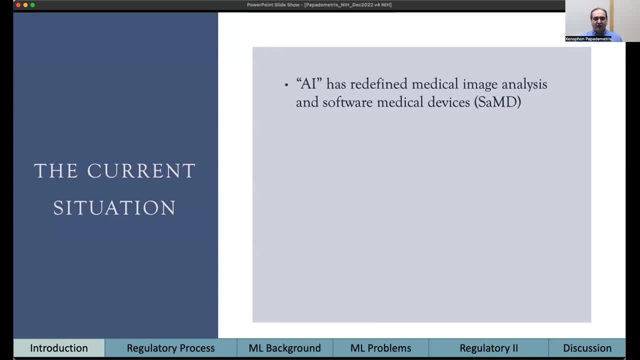 tools through fda and other regulatory agencies for use for diagnosing and treating patients. ai is kind of like gene therapy or stem cells. has created wide interest in the general public and fears and reactions. so by the end of the day, maybe 20-25 years ago, when the whole thing in image analysis was level sets, 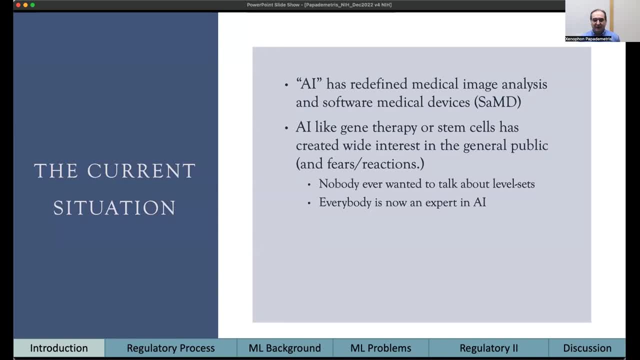 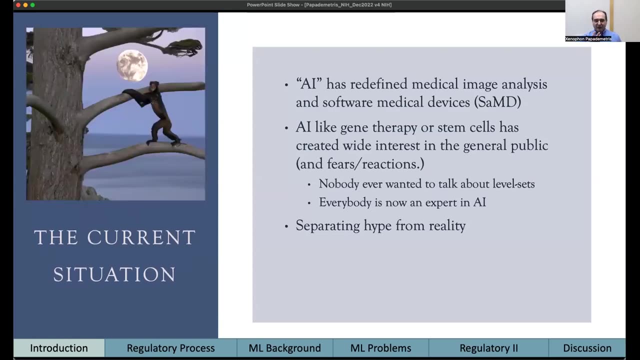 nobody really knew what level sets were or cared about that. everybody's now an expert in ai. if you walk into any medical school, everybody's clearly an expert in ai and i challenge really, when you see results published out there, to separate the height from the reality. and that's really what we're dealing with. so here's a cartoon. 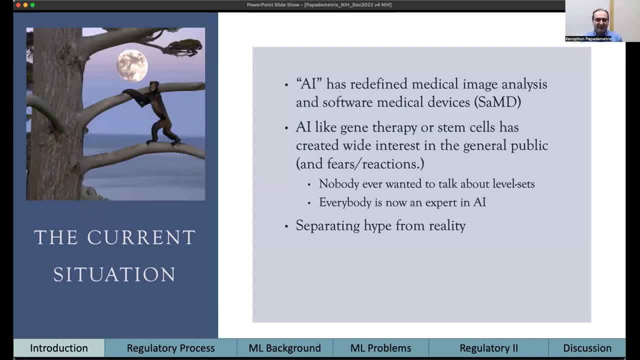 just right to the height, drawn with one of those text to image synthesizers, stable diffusion, and this is a picture of a monkey climbing a tree and the code comes from the 60s. this is geodrey fuso, the early researchers in this field, and he said: you know, there's lots of hype in ai. 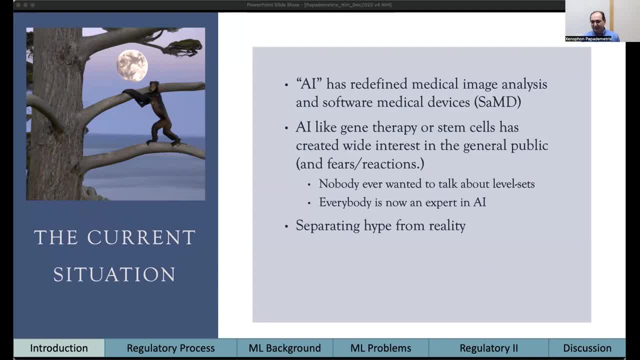 and you know we go back and forth. he said it's like it was like claiming that the first monkey that climbed a tree was making progress was landing on the moon. so yes, we're making progress, but are we asking to getting there or is it just an illusion? so just keep the mind in place. 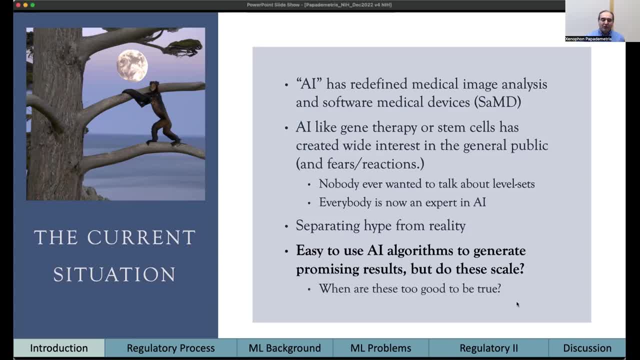 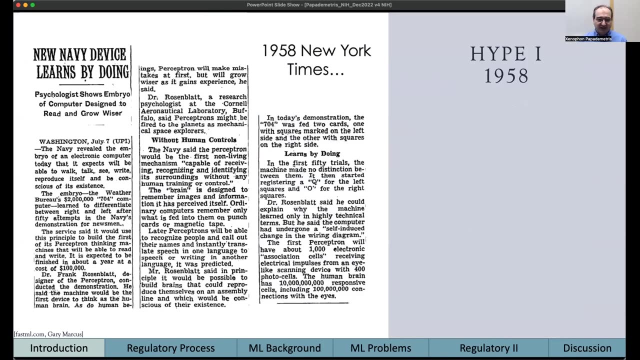 yeah. so with that, it's very easy to use a outcomes to generate promising results. but do these things scale? when are these things too good to be true? so that's where we're dealing with as we speak right now. so that's where we are. so the hype didn't start yesterday. you can go back to 1958. 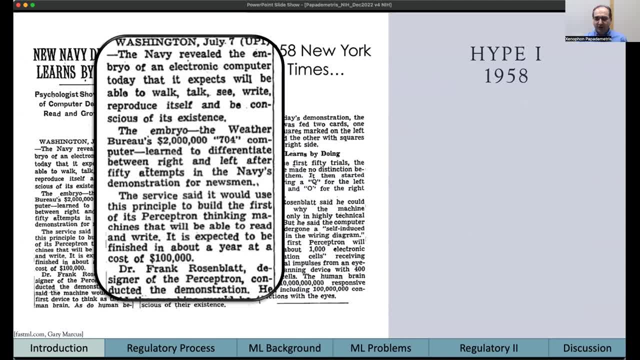 and the new york times, and there's an article about the first percytron. and here we go. the navy revealed that the, the embryo of its, of an electronic computer today the expects- would be able to walk, talk, see right, reproduce itself and be conscious of his existence. the embryo, the 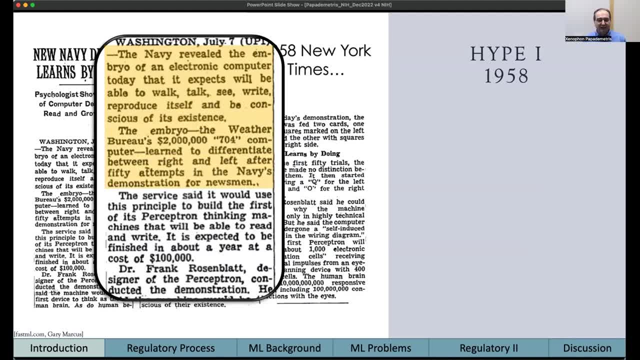 weather bureau's two million dollar 704 computer learned to differentiate between right and left after 50 attempts. in the navy's demonstration for newsmen, the service said that it would use its principle to build the first of its perceptron. thinking machines will be able to read and write. 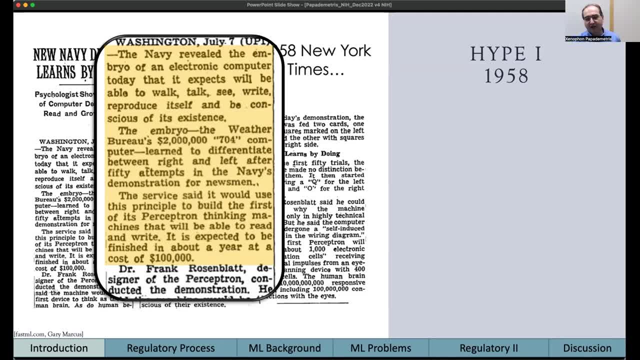 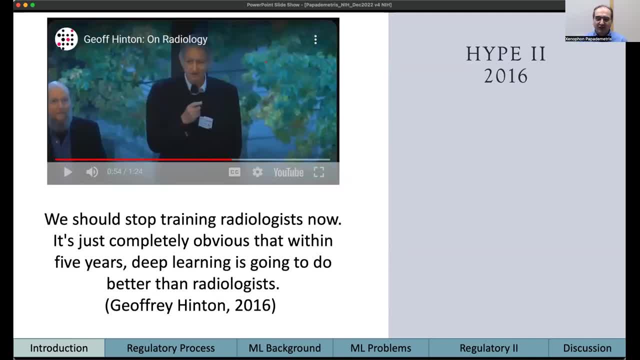 it is expected to be finished in about a year at a cost of a hundred thousand dollars. so this was 1958. clearly, this never happened, right? we know that. here's hype slide number two: this is not. we're not going to play these videos, but this is on youtube, you can find it. this is from jeff. 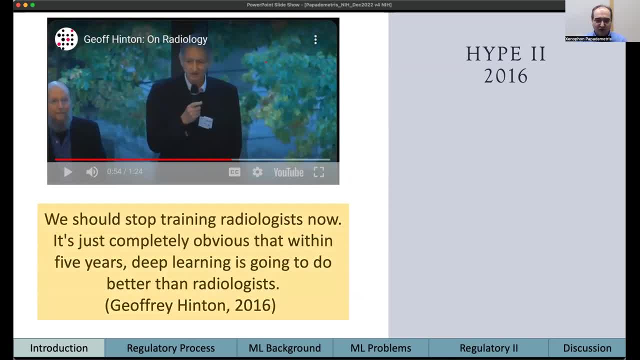 hinton, some of the fathers of deep learning, and this is the comment. we should stop training radiologists now. it is just completely obvious that within five years, deep learning is going to do better than radiologists. now i sit in the radiology department. we have lots of radiologists. 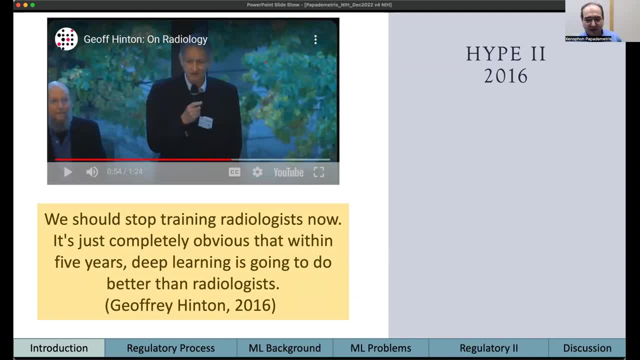 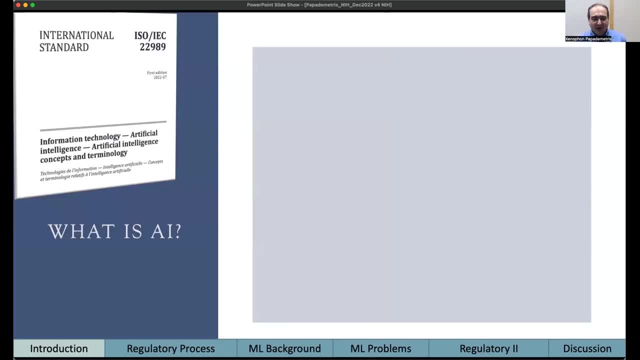 we're having a shortage of radiologists, and deep learning is nowhere near replacing radiologists. so i can tell you this much from my own lived experience here. so what is ai? we've heard the words. let's just get some definitions. it's from one of the international standards, isos 22 1989. 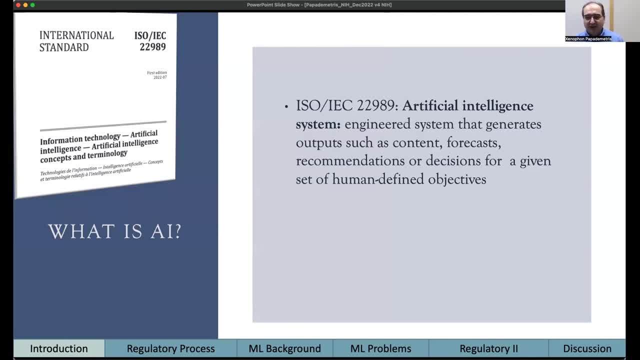 you get this very, very broad definition: an artificial intelligence system. this is an engineered system that generates outputs such as contents, forecasts, recommendations or decisions for a given set of human defined objectives. so this is basically almost everything outside expert circles. my working definition, just talking to people at the medical school here, is that ai is some magic that allows a computer to do something. 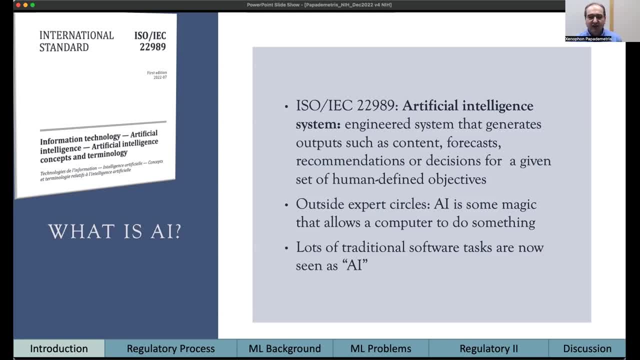 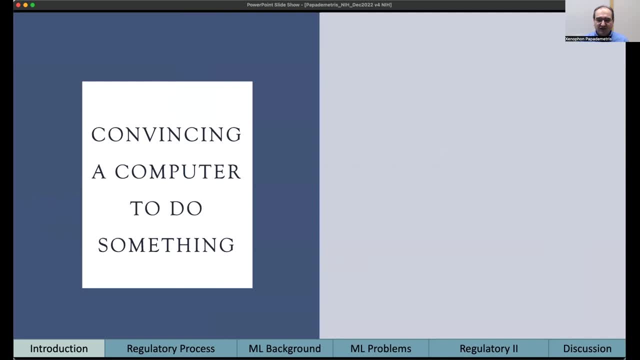 and lots of traditional software tasks are now seen as ai, so people will call ai just about anything. okay, so if it's done by a computer, it's ai. so let's just back up and think a little bit about the taxonomy here. let's: what does it take to convince a computer to do something? 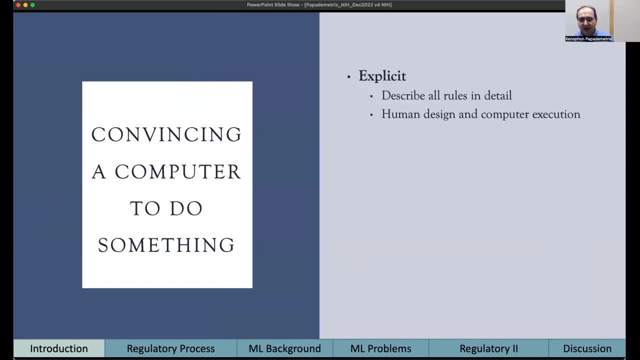 there are sort of two ways to do it. one is to convince a computer to do something. there are two main ways. there's an explicit way where we describe all the rules in detail. this is traditional software programming, and here we have human design to a great level. 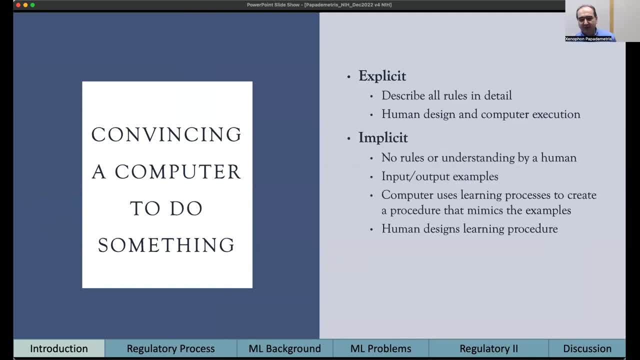 of detail in computer execution. and then we have implicit methods. we have no rules or even understanding, sometimes by human. we have lots of input, output, examples. when i, when you see this, do that type thing, the computer uses learning processes to create a procedure that mimics the examples and you can set the human designs, the learning procedure on the. 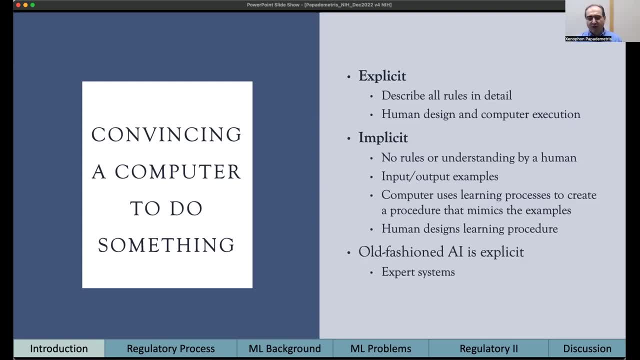 computer then figures out the code. old-fashioned ai is explicit things like your favorite expert systems when you used to call your bank to ask for help and say press two, then press three, then press four. machine learning falls into the category of implicit systems, where we just give it examples and everything from like. 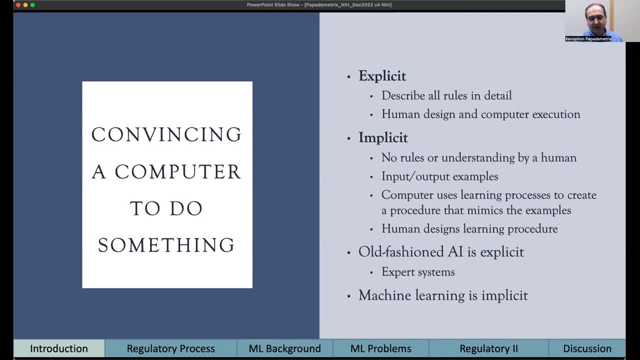 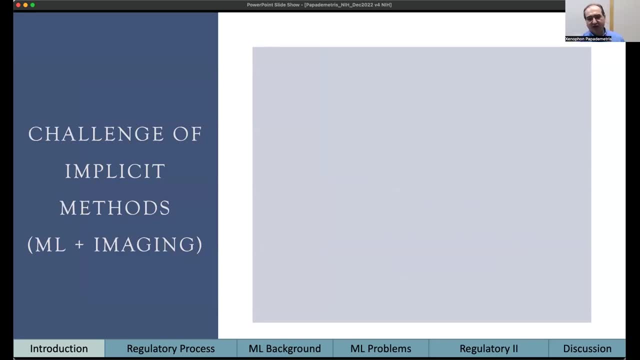 the simplest regression model to a deep neural network comes under that category. here are some of the challenges of using these implicit methods, and this is for primarily, machine learning and imaging, although the same things apply to other things. what we learn is super specific. an algorithm used to classify pediatric brain tumors may be useless. 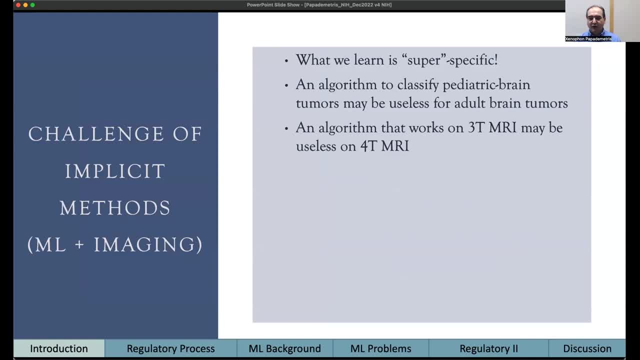 for adult brain tumors. that's just one example. another works on three tesla mri. as a field strength that's the most common in hospitals, may be useless on four tesla mri. an algorithm that works on a particular resolution may be failed partly at a slightly different resolution we have. 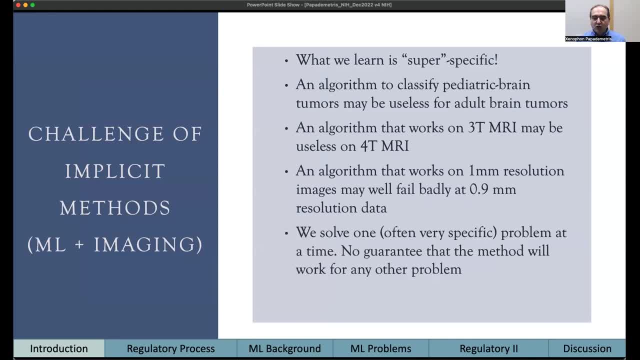 examples of that if you want to see them on day, and what we do is that we solve one very specific problem at a time. there are no guarantees that this method will work for any other problem, and we often do not understand how it works and we're not able to predict how it fails. 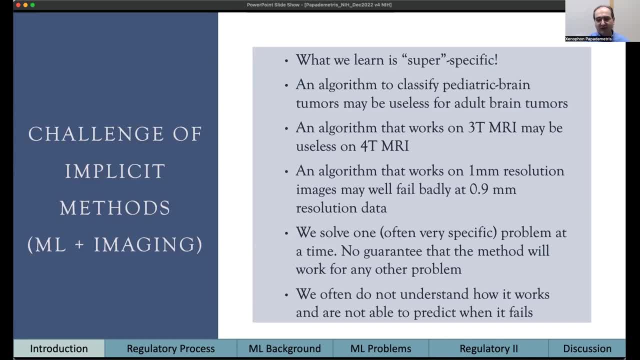 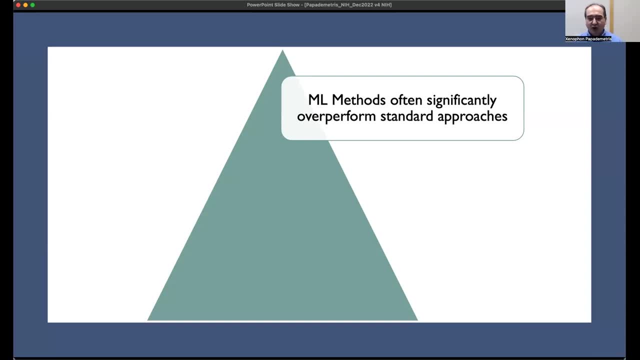 so this is our challenge. something works really well when it does, but it's super specific and we don't know whether it will, how it will fail, and this is what's the such a stage for the talk. we have these methods that often, significantly, will outperform or perform standard approaches. 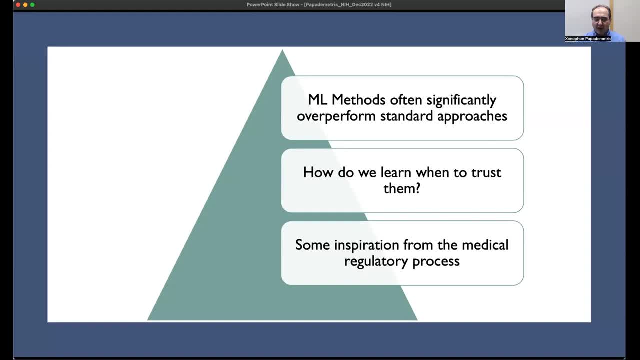 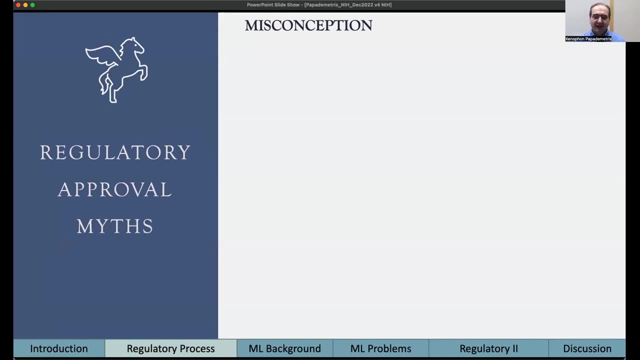 how do we learn when to trust them? this is a fundamental question, and what i'm going to do is i'm going to look at the medical regulatory process for software to get some inspiration, for some ideas as to how to go about that. so, for those of you who are not super familiar with the regulatory process for medical devices, 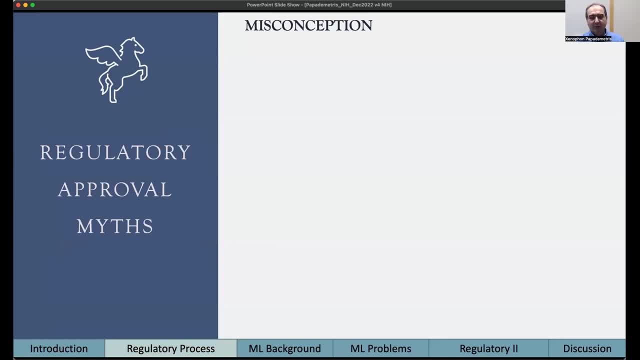 medical software. here's a common misconception. this is how i thought things worked 10 years ago. maybe you code your software however you like. at the end you perform a validation study, you submit the results to the fda and if the results are good enough, you get approval and then you're. 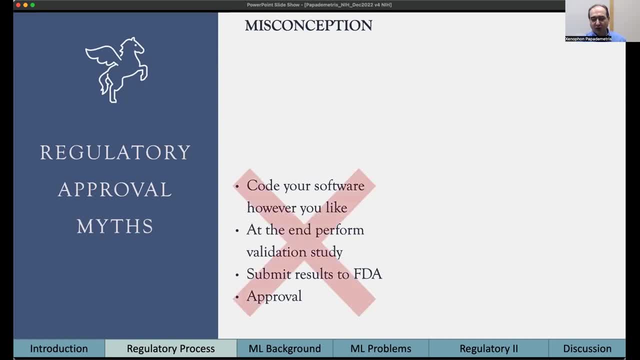 free to sell and make money and make your fortune. this is not hard work, so the way it works is that you start out in your company and you establish a quality process for creating software. you have a lot of rules in place for who can code, what training they need, what, how. 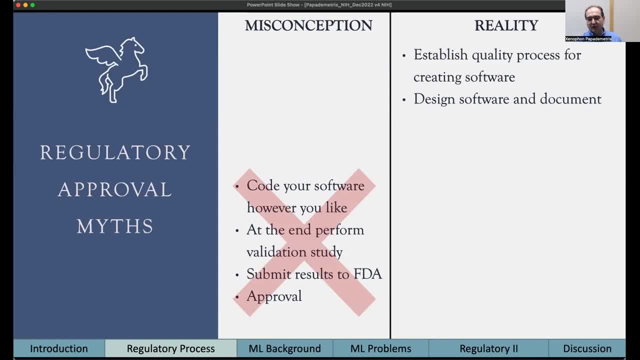 do we go about committing code etc. we design our software and document it. we perform risk analysis to think and figure out what could go wrong. the fda will optionally review your plans ahead of time. you implement your software and document. you perform a pre-specified validation study. 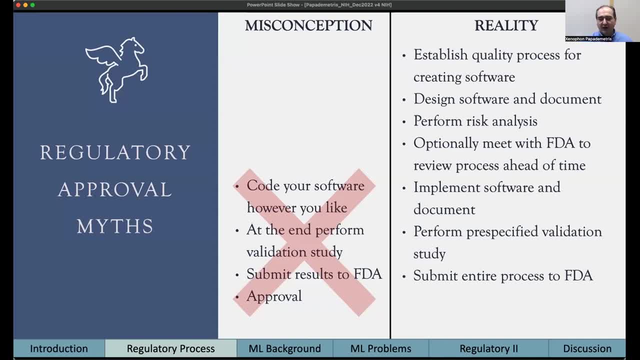 you submit the entire process to the fda. the testing is part one part of it. you get approval or clearances or technical terms- we're going to get into them now- and you're still responsible for monitoring how the whole thing works after you've sold your. 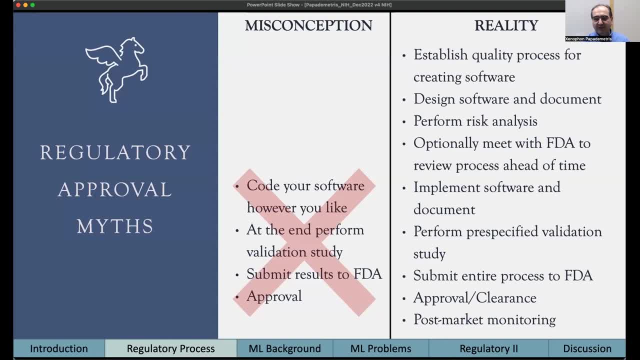 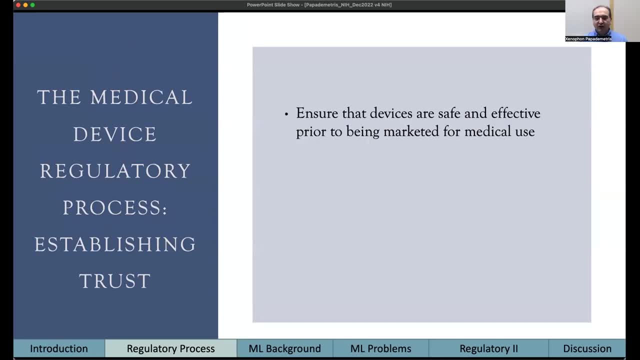 product. so it's a much more involved process, and the first step is this thing called the quality process. so the medical software process is all about establishing trust, and we want to ensure that devices are safe and effective prior to being marketed for medical use. if we're thinking about 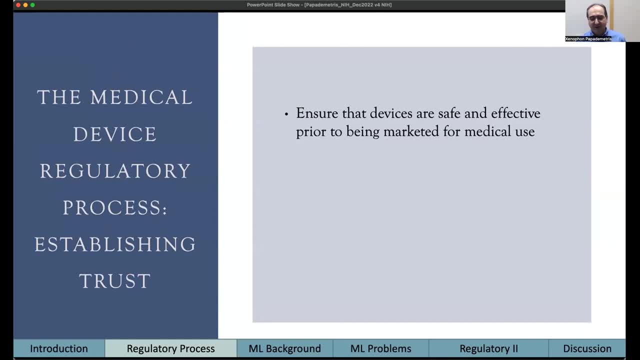 medical image analysis research. we want to ensure that our algorithms are safe and effective for using them. for there was a paradigm shift in industry- maybe sort of this taste about world war ii- and this is the shift from quality by testing to quality by design, and this is sort of 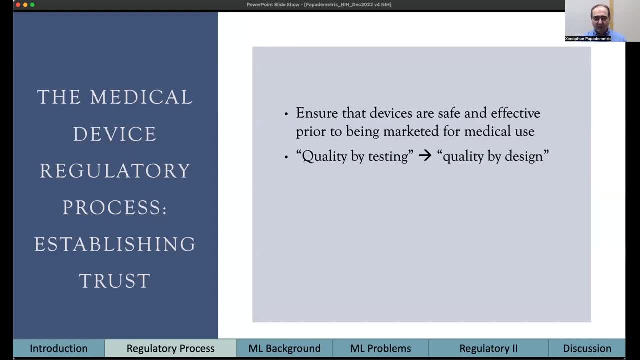 we build it, however we build it and we'll make sure it works at the end. to having processes that make that, ensure that what comes out at the end is good every time. and this ideas came to full development in post-world war ii japan during the process of reconstruction, and they were important. 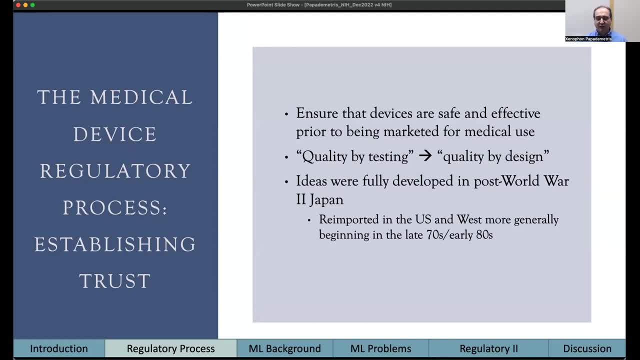 in the states and the west more generally in the late 70s, early 80s. you've heard of things like total quality management, the toyota way. all of that is the sort of core of what quality systems are, and this led to the creation of. 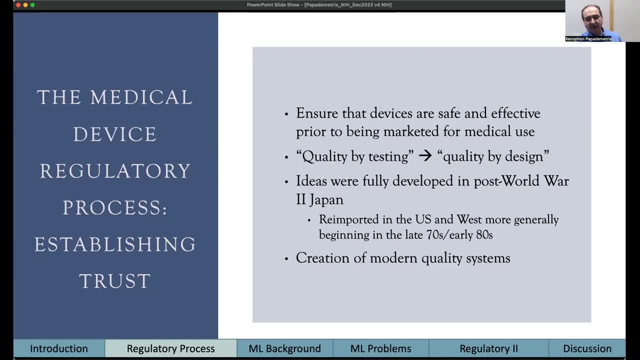 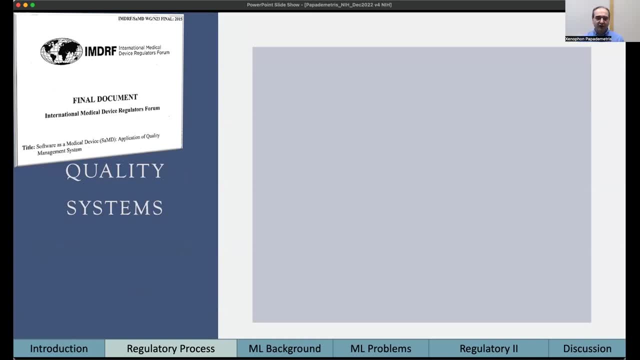 modern quality systems, which is now embedded in the medical device regulations, beginning in the 90s probably. so what? what do these things include? this is one of the regulatory guidance documents from one of international organizations, international medical device regulators forum. again, the goals of quality by design. 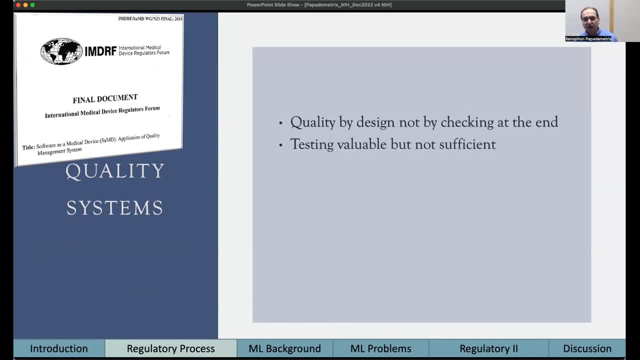 design, not just by checking at the end. and it comes out of recognition that testing, while valuable, is not sufficient. okay, you can't just test quality into something. we cannot trust the results unless we have a good process in place. maybe we got this due to pure luck, maybe a rat. 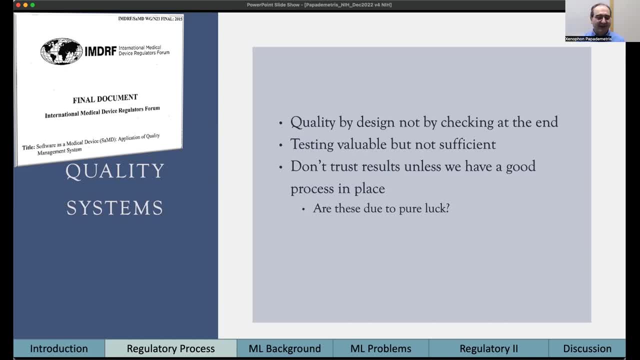 can work really well, because we found images from patients that were really not particularly variable and more likely. there are explicit procedures on how key things are done, and this includes- and this again another lesson for our research population- training for personnel. you can't just have somebody in a lab. 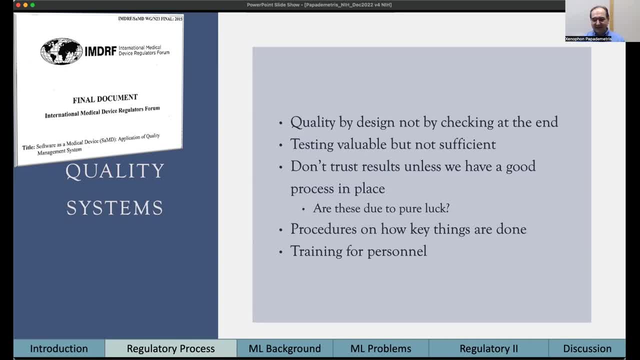 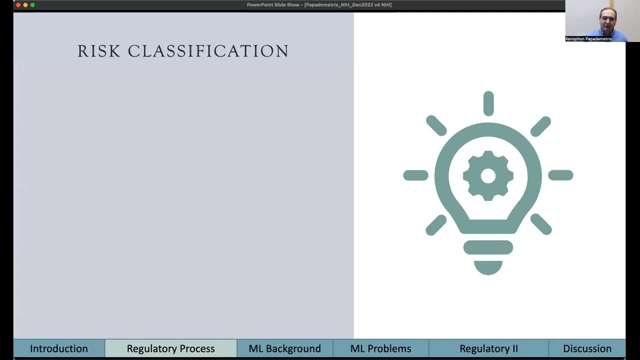 barely knows what they're doing. download some code, download some data and come up with results and you feel like, yeah, that was good results that are published. people need to be trained to be qualified to do the work they're doing, otherwise we risk getting random results. sometimes they work. the other thing- and if you remember one thing from the talk- is probably this: 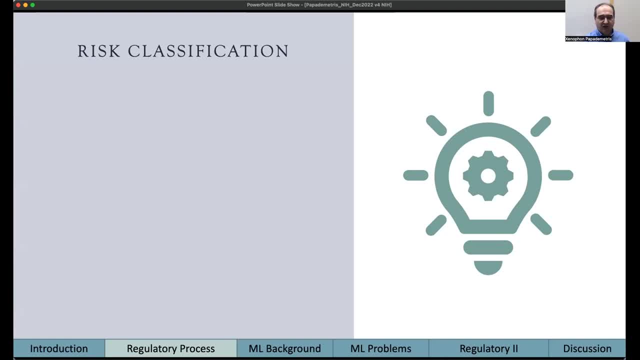 slide. there's a concept in the regulatory process of risk classification, so the focus is on what the risk is going to be used for, not on what it does, and these are the so-called use cases. so once you know what the software is going to be used for, we estimate the risk involved. 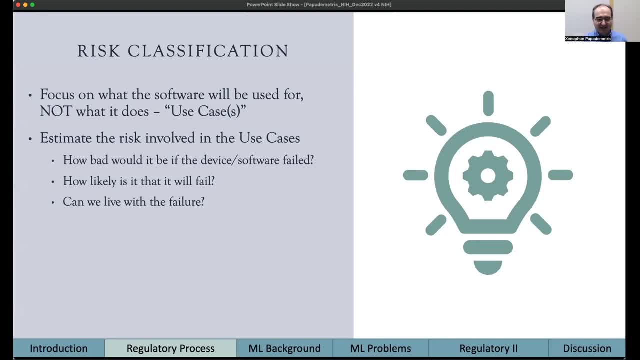 how bad would it be if the software device failed? how likely they will fail? can we live with the failure? and, based on the use case and the risk involved, we end up with the risk classification, something like low, medium, high. there's a million of these schemes. they're all slightly different. 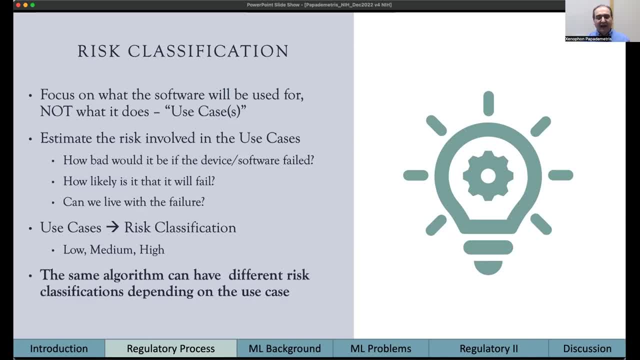 but they all boil down to something like this: and the same algorithm can have different risk classifications depending on the use case. so it's not what the algorithm does, it's not what the tool does, but how it will be used that drives your risk classification. so let's look at some practical 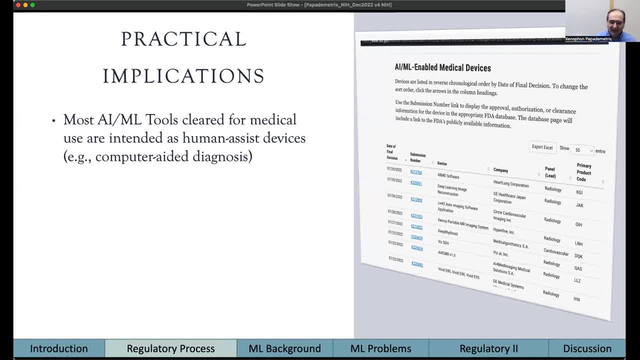 applications. on the right, you'll see a table of ai enabled medical devices comes from the fda's own web pages, and most of these tools that are cleared for human use are intended as human assist devices, for example, computer-aided diagnosis, and the reason for this is that it lowers the risk level. 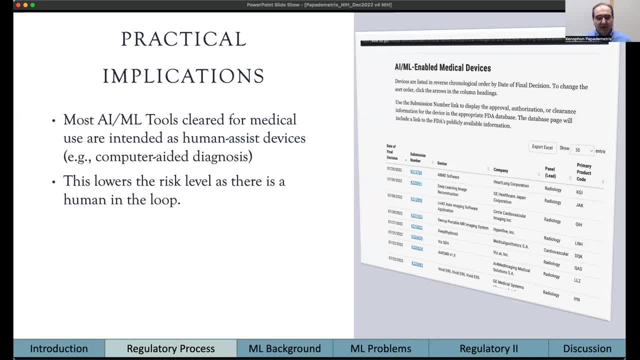 because there's a human in the loop. if you're just doing dealing with non-fully automated things, the risk is lower because the idea is that a human can catch the arrow algorithmically. these are identical often to what could automate the diagnosis tools. you could use the same tool for human assist or completely automatic diagnosis, but the risk 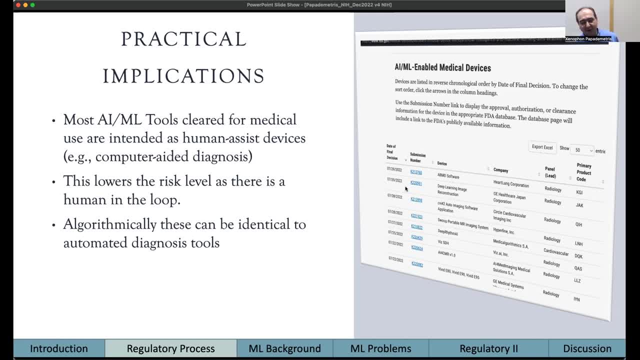 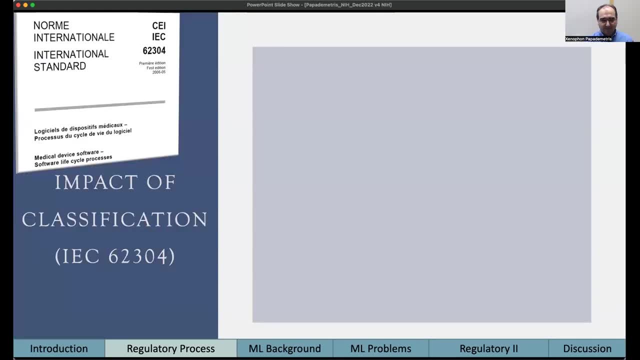 profile is very different, because you say, well, we have an expert that's going to look at the results of a lower risk tool and that's why, actually, most of these tools tend to be, you know, designed this way. what is the practical impact of the classification on the nitty-gritty of creating software ai tools as part of that, if you have higher risk, 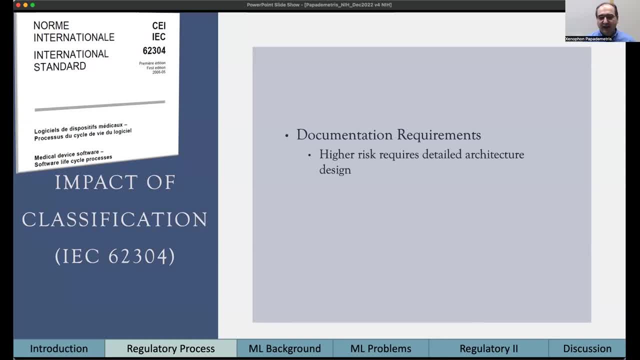 you require more detailed documentation when you submit to the fda, for example, a detailed software architecture design. and on the testing side, if you have higher risk, you require, for example, unit testing and more detailed testing, more detailed clinical testing. so the scrutiny goes up as the risk level goes up, and that is the principle of the thing here. what are the? 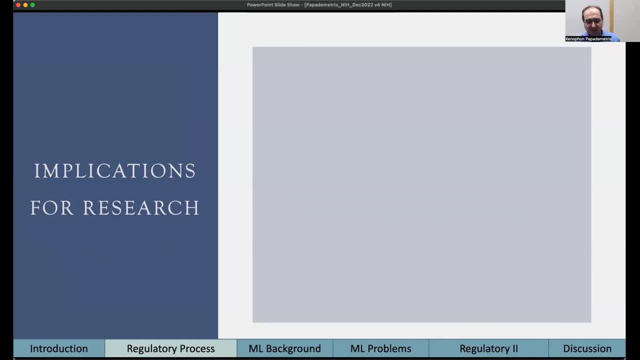 implications for some of our own research. what are the implications for some of our own research outside of the medical device process? we should expose things that are more impactful, that make more impactful claims, to high scrutiny. you know, if this is a claim that this is going to massively affect everybody and it's a high impact. 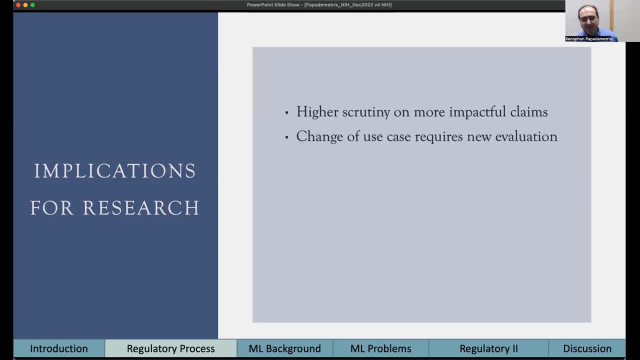 paper. we should put high scrutiny on it and we should always keep in mind again- and you'll see examples of failure later in this talk- well, that the change of use case of research requires a new evaluation. here's an obvious example. we do not use lab studies to get drugs approved, they do clinical. 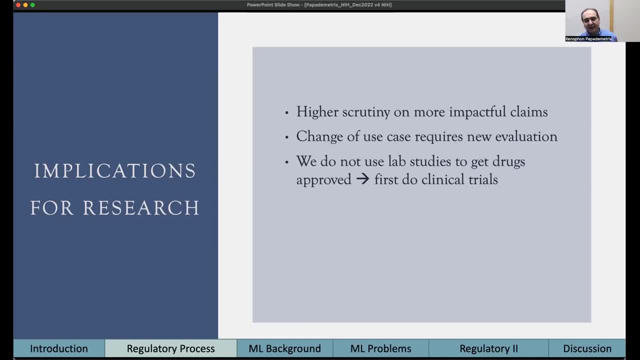 tests, even though theoretically it's the same process, it's the same drug, the lab paper, the research from the university. they use cases to demonstrate, you know, initial feasibility. you cannot use that to get clear and approval for testing for putting a drug into the population at large and i would argue that we should not rely on ai or other software driven results from pages. 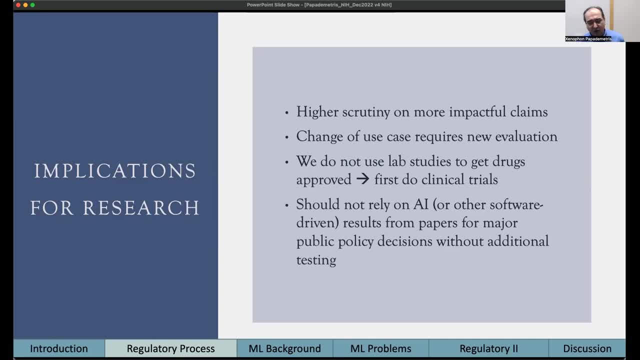 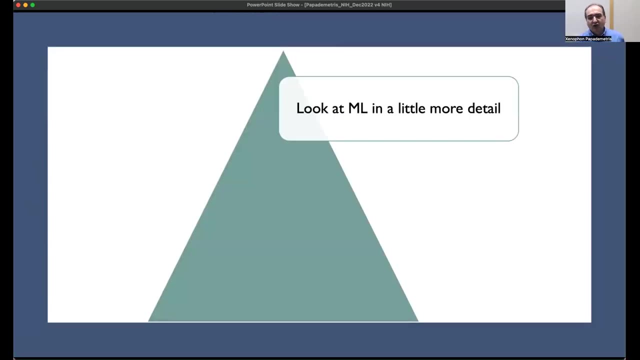 for papers for major public policy decisions without additional testing. and we saw that during the pandemic, all these models that were published and then people were using them to make the decisions, were those subjected to the level of scrutiny that you would have taken for that use. so we'll come back to that at the end. so with that out of the way, we'll look at machine learning. 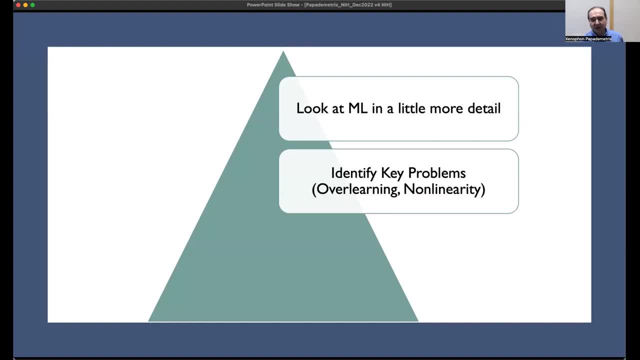 in a little more detail to establish some common ground for everybody. we'll identify the two key problems in my mind: the possibility of over learning and the issue of non-linearity, and this undergird a lot of what you will see: domain shift and other terms that you will have heard. 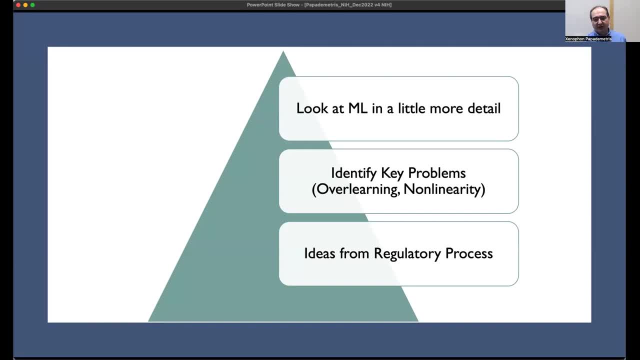 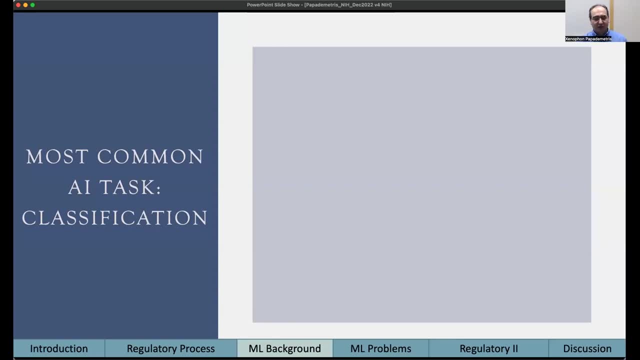 and we're going to look again at ideas from the regular term process for how to address a little bit of those as well. so the most common ai task is probably classification- is labeling something as good or bad as healthier disease? what have you? and the typical process goes: given some measurements, descriptors or features, we assign a label to these. 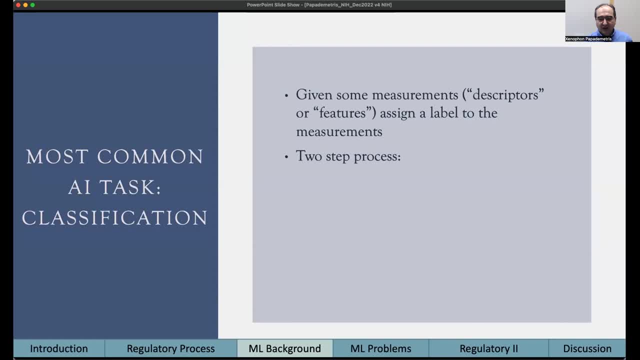 measurements and this is often a two-step process. given a thing, a human being- maybe you might be into measurements of features. we call this representation, perhaps so a person could become the two numbers height and weight, and given these measurements, the features we classify. so, given the weight and 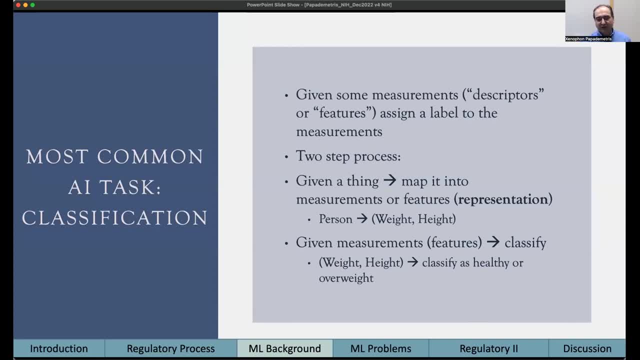 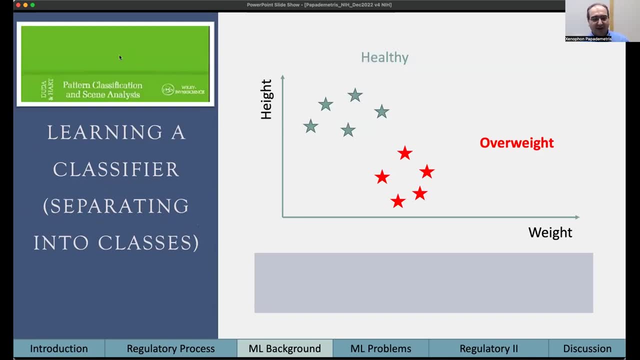 the height we classify as healthier or overweight or high risk for diabetes or what have you. so the process may look like this: this goes all the way back to the classic text by duda and hart, this back in 1973. and here may be our data: the healthy are the green, the overweight are the red. 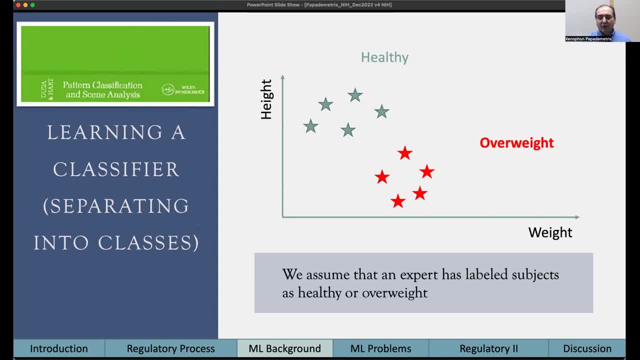 they're higher on the weight load on the high scale and we assume that some expert has labeled the substance as healthy or, where we have some clinical diagnosis, there's a reason why that is and based on that we may learn a line- the line shown that separates the state. that is the 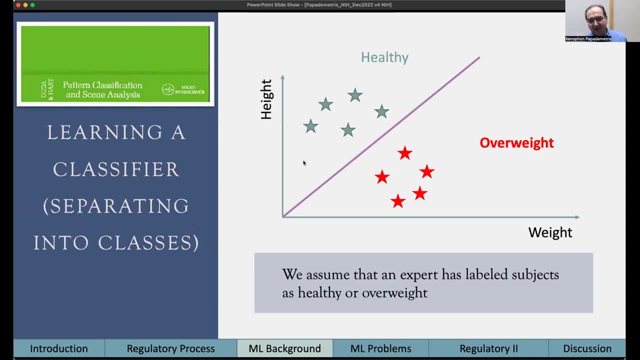 classifier and we get a new measurement. if it's above the line, we say okay, that's healthy. if it's below the line, you say that's high risk, or other way. that is the most fundamental part of this process. now, this is one way to do it. another algorithm that again dates back to that era is: 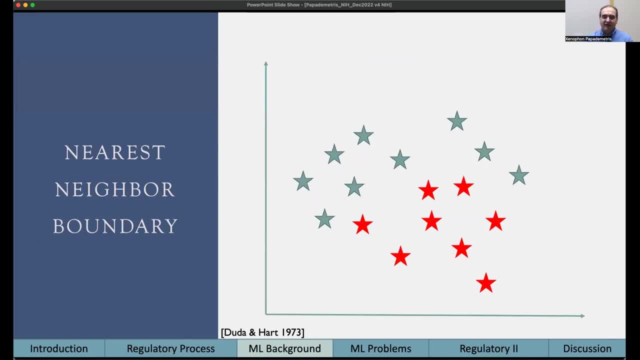 the nearest neighbor algorithm, and here we memorize all our examples. so this is the old saying in ai, and when we get a new example, we classify based on what is nearest neighbor or neighbors where. so if you do that, you get an implicit boundary that looks like this: below the curve, you're in the red. 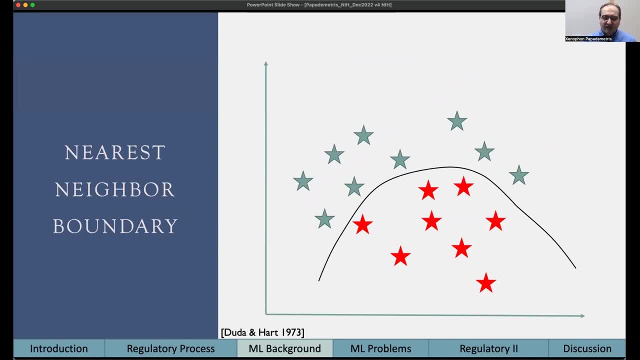 category. above the curve you're in the green category and that's just driven by how close you are to an existing sample. if we were to get one more sample up there, maybe now we have a three part partition: top and bottom of high risk, middle is no risk and this is either the nearest neighbor. 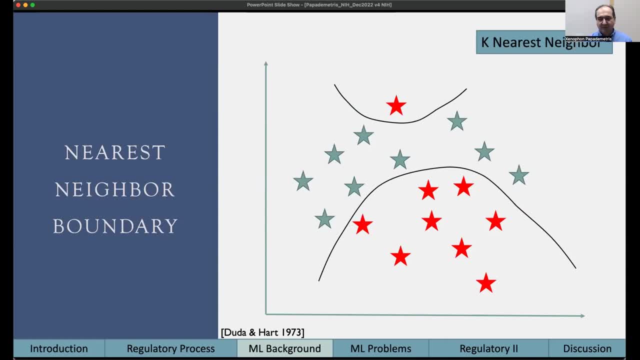 or we have k nearest neighbor. okay, can be five, seven, nine, depending on your application. let's continue the story. you could have a situation that looks like this and now maybe get another example. and now we have an island in the middle, so this little spot here with the red star is in the middle of the grids. now inside the island, you're high risk below your. 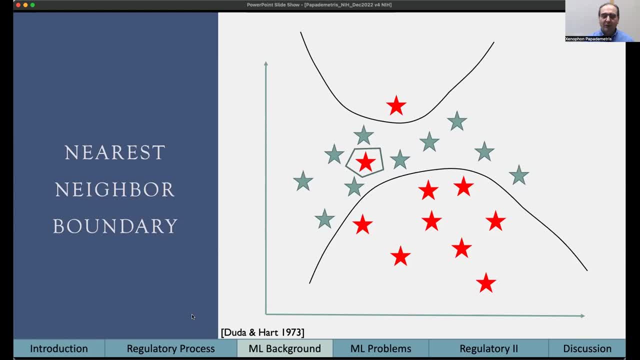 high risk, above your high risk, and this type of structure is more common. when you look at deep neural networks, you have a lot of islands. really you don't have a clean separation. what happens at those points labeled with question marks that are far away? what happens if a doctor 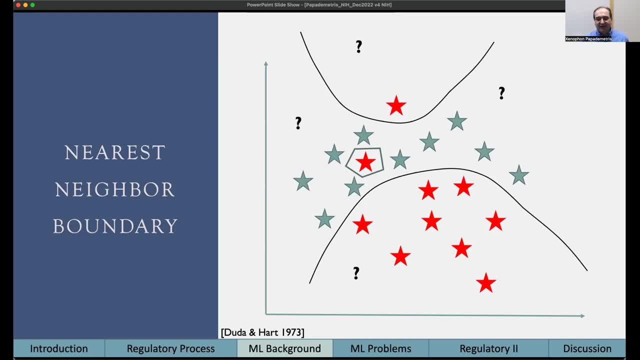 sees a patient that's unlike anybody they've seen before, the answer is that their experience is going to help them. same happens to classifiers, and coverage is critical. okay, we're unlikely to get good results if we're far away from training samples, if our patient doesn't look like any. 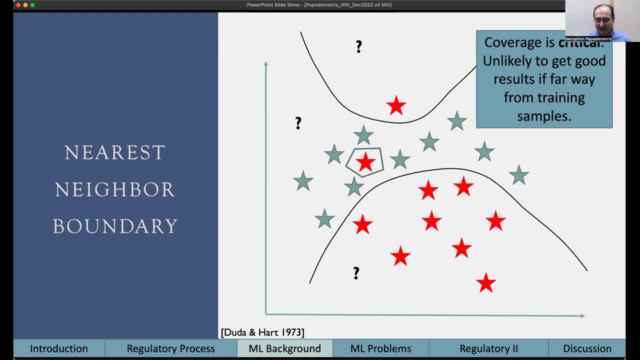 patient we've seen before. whether visually, we have a patient of a different skin color on our database or the presentation of the disease is very different, we're unlikely to get a good result, and that is the fundamental limit of all machine learning deep learning. we need a lot of samples. 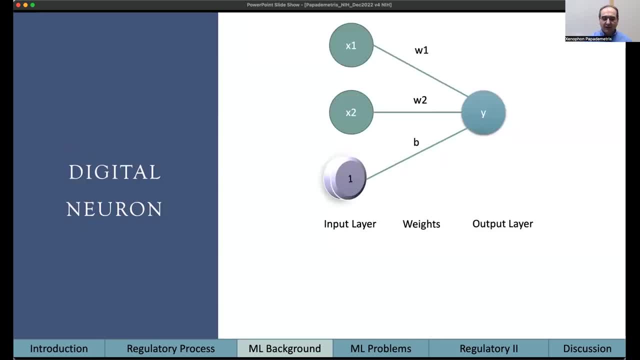 and we need good coverage and we'll come back to that again. here is what a digital neuron looks like. this is the building block for a neural network. we have an input layer. this number is x1, x2 and 1, so the inputs, we have some weights, w's and the b here, and we have an output, y, and this is the y is the. 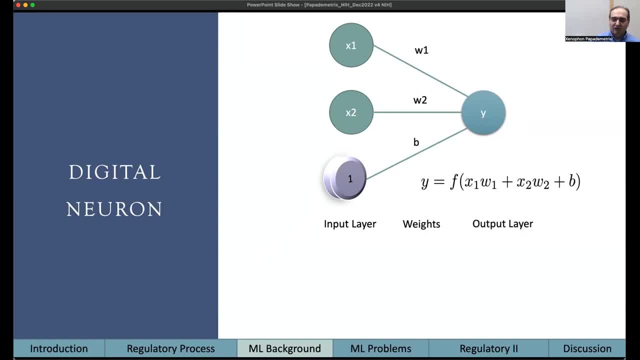 simple neuron and the neuron could have an output like a function, that's sort of the function of the weighted sum of the input. so x1 times w, 1 plus x2 times w, 2 plus u, we have the input layer. this is what we feed into the, your network: the weights and the. 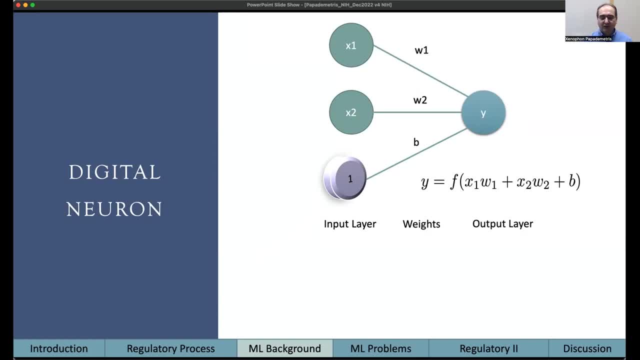 output. and then in practice, what happens? you give it lots of examples of xs. we know what the ys are to be and we tweak the weights to get the right answer, and that is how you trained the cell. the function f may be something like a threshold potential leaf a, then what goes into f is greater. 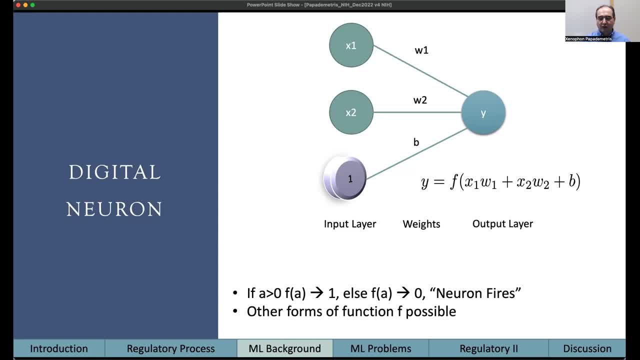 than zero. you can output one hours zero and we say the neuron fires by the biological analogy. there are other forms of ANDS asking in addition to layman's corner or between species and you, of function available or values, sigmas, what have you? 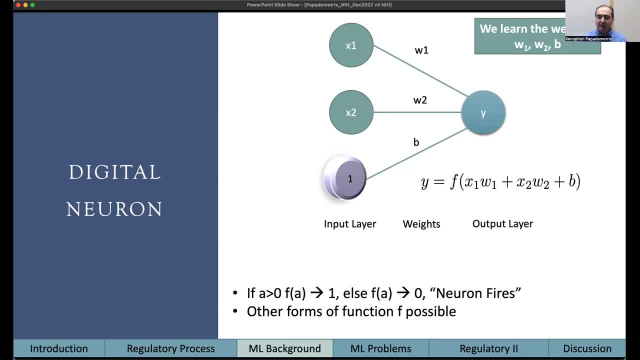 And again, just to reemphasize, we learn here the weights w and w to b from example data and then we use or apply them to a new input. Now, if you take lots and lots of these things, oh, just a final point here before I move to the next slide. 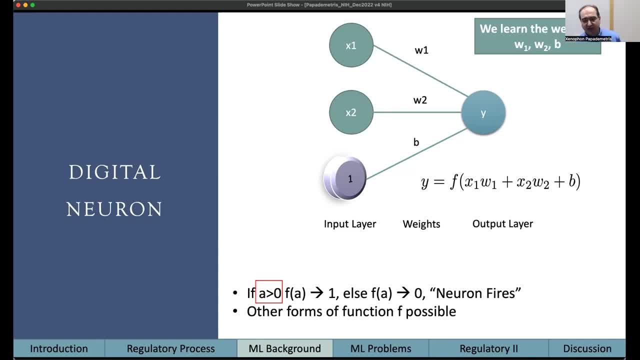 just want to highlight that thresholding process. if a is greater than zero, What do we have here as an example of a nonlinearity? If we go from a minus 0.001, we get a zero, to a 0.001, we get a one right. 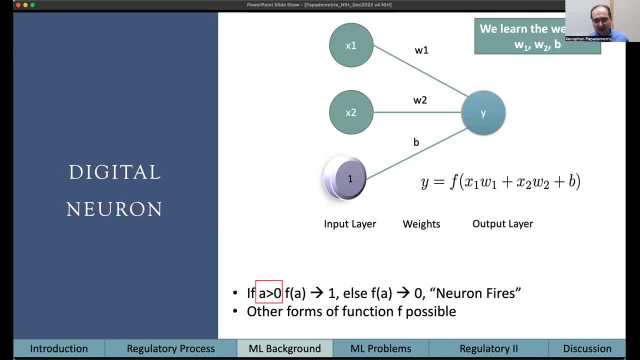 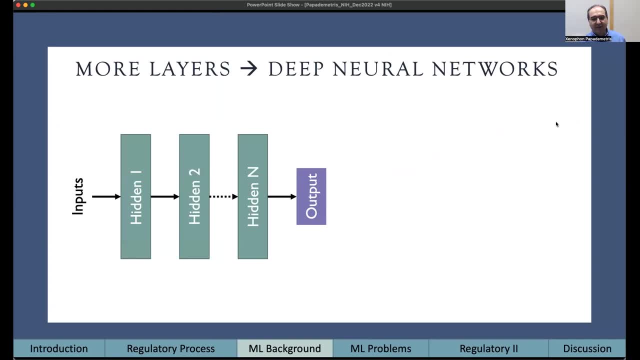 So a small change in the input and a large change in the output, and we'll come back to that. So if you take a lot of these neurons and we clone them together in parallel to create layers, and we have lots of layers, one after the other. 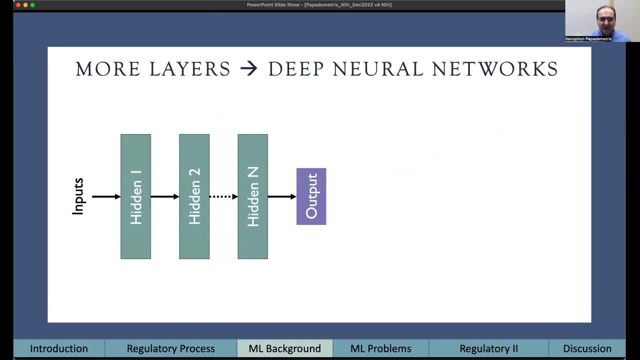 we have neural networks and if we have a large number of layers we get deep neural networks. That's really all it means. It means you have a lot of layers. To train this, we need lots of examples. We guess the initial weights and adjust them. 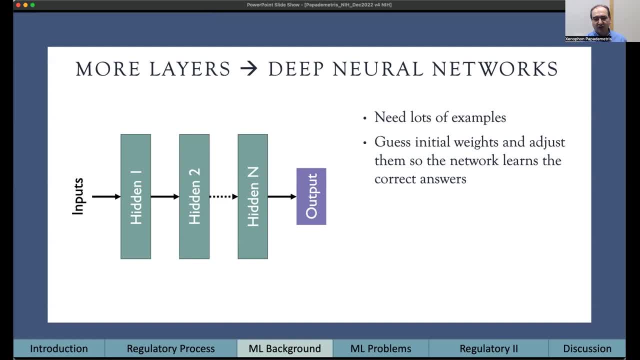 so the network learns the correct answers. There's a process known as back propagation: more neural networks. It turns out in imaging- not by design, but that's how life works- that the first few layers learn features. they learn a representation. 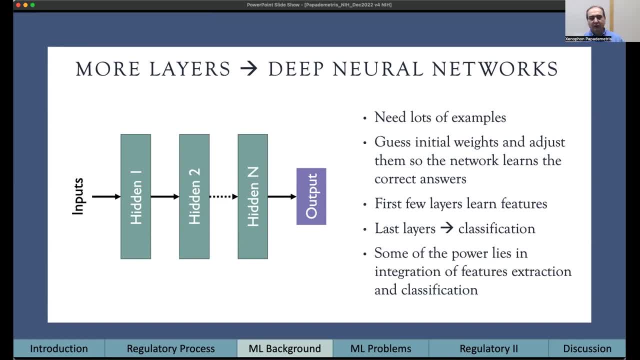 and the last few layers learn a classification. Really the power of deep neural networks and why we get such good results is this integration of feature extraction and classification. So instead of trying to figure out by hand what the features ought to be, the weight and the height. 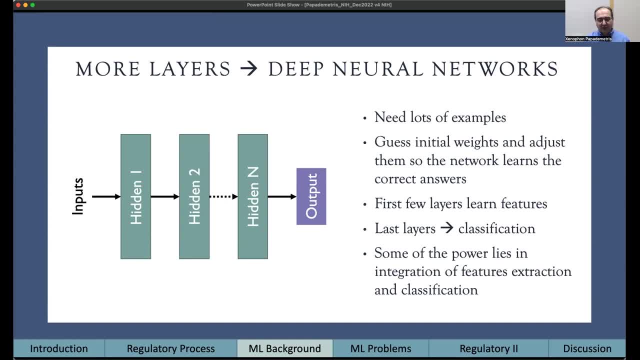 we give it as much as possible the raw data, the images, and it figures out what the right features are and then uses those to do classification, And so you can get features that are optimal for separating classes as opposed to features that are optimal for something else. 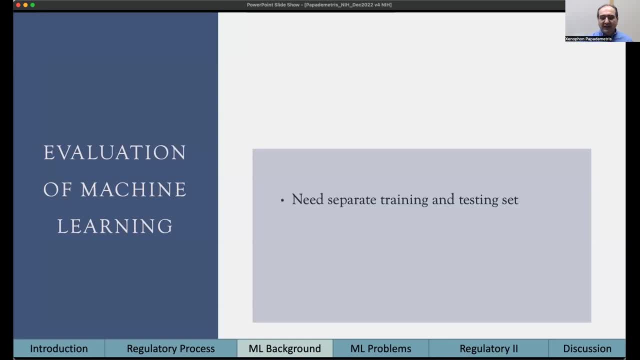 How do we evaluate this thing? So here is the typical process. We need a separate training and testing set. That's probably the single most important thing. That flow chart above shows the process. We have some training data. We use it to train a model. 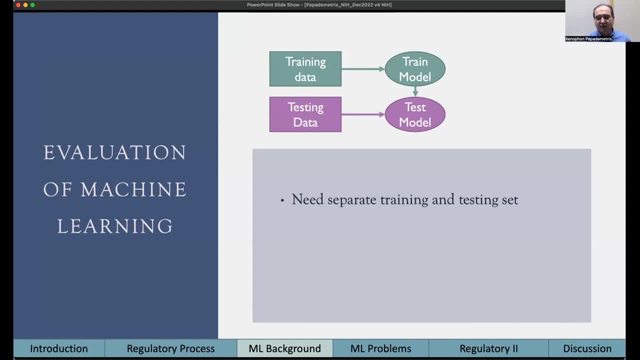 We have a separate set of testing data and we use it to test the model, And the reason for it is especially when it comes to deep learning. these are so powerful that they can memorize the training data. So we only really are interested is 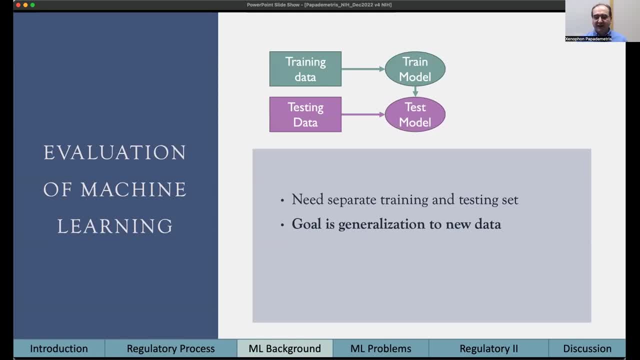 how well does this model generalize, how it well performs on data that it was not trained on. Otherwise we can just memorize the data. Ideally, we should use a completely separate testing set In practice most applications, because we don't have as much data. 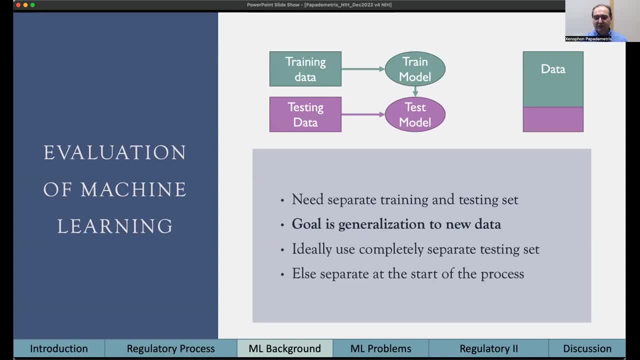 we separate at the start of the process. We take our data, we split it off into testing and training, We do the training and the testing And you can do permutations. You can do permutations of that. Post-validation would have you in some cases. 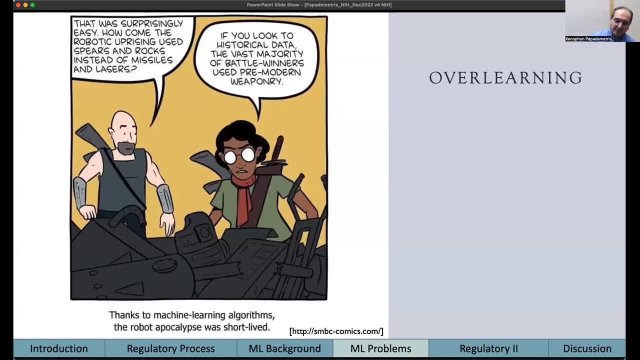 but we'll leave that for later. The fundamental problem, as I alluded to before, is over learning. It's a great cartoon that illustrates the case, So let's just walk through it. The title says below: thanks to machine learning algorithms. 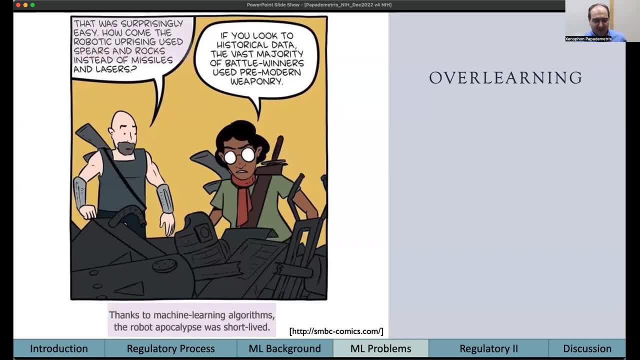 the robot apocalypse was short-lived, So soldier1 asks: this was surprisingly easy. How come the robotic uprising used spears and rocks instead of missiles and lasers? And here comes the answer. If you look at historical data, the vast majority of battle winners. 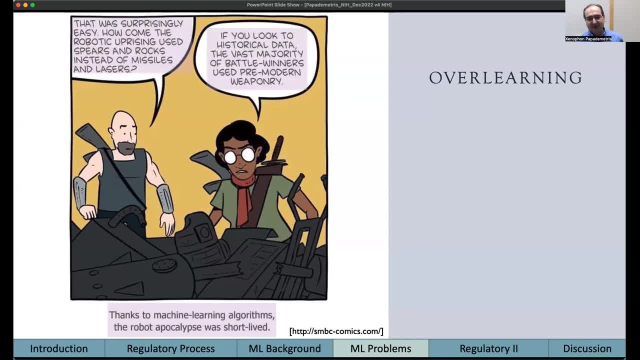 use pre-modern weaponry right. History goes back thousands of years And most of those battles were fought with stick and stones. To me, if you want to put some math on it, the statement a measurement like what happened in the battle. 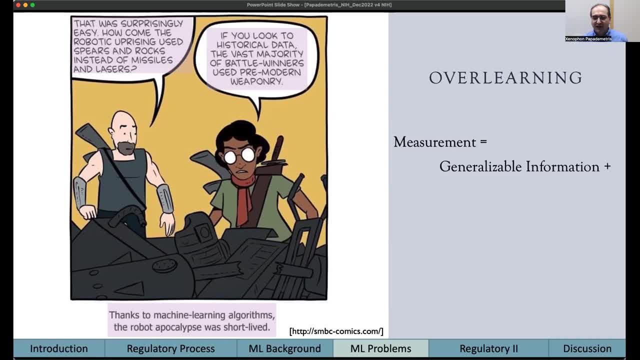 consists of perhaps the generalizable information which you should take away from it. Larger armies tend to win, Something that was idiosyncratic, that just happened to happen at that event, but doesn't really something you want to carry away. You know, if you're tired in the morning, you tend to win. 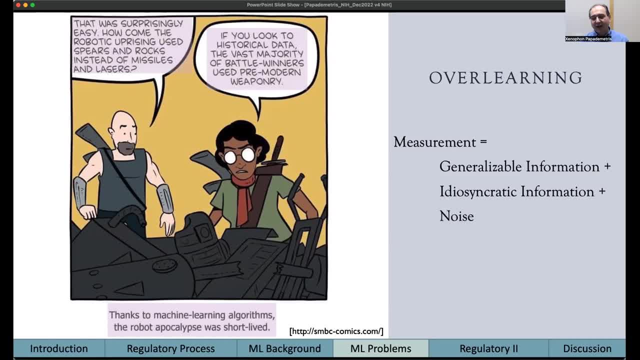 Maybe, maybe not, but it may have happened a few times and you learn it. And, of course, noise. the report we have of the battle may not be exactly what happened. It may have been altered to protect the reputation of winning generals and powers, et cetera. 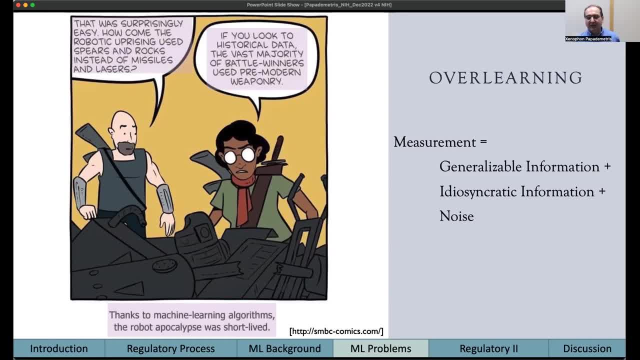 The goal of machine learning is, out of our measurements, to learn something that reflects the generalizable information and hopefully filter out the rest. Easier said than done, but in general the general information is the most stable. So if we don't try to overlearn from our data, 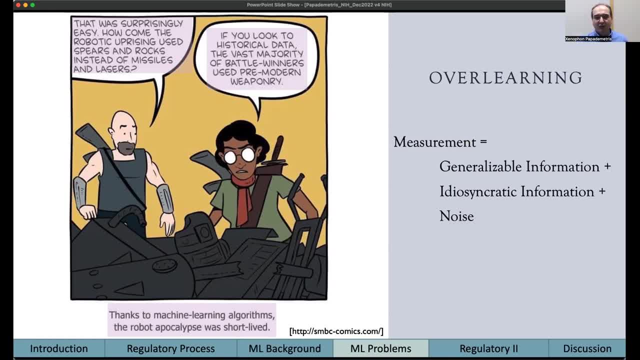 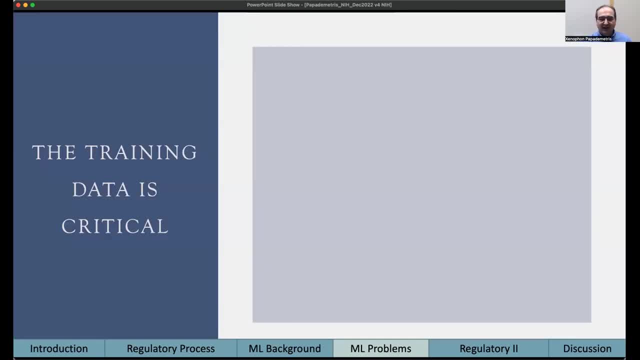 to not overfeed our data. we'll extract that, And as you try to squeeze more out of your data, you end up in the second or third category. The training data is critical. So the last military adage of the day. this quote is attributed to many people. 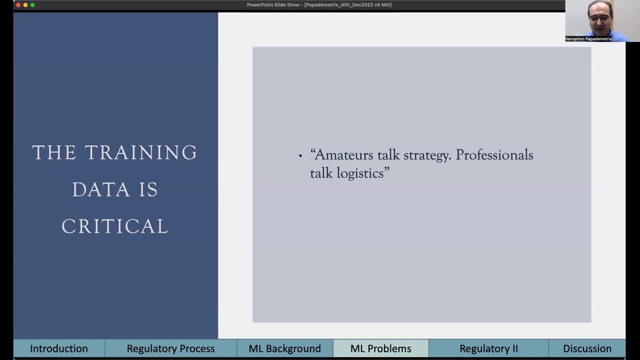 so I can't claim to figure out who it is, but it says: amateurs talk strategy, professionals talk logistics. I would say, in machine learning, amateurs talk networks or structures, professionals talk training data. Not that the networks are important, strategy is important too. 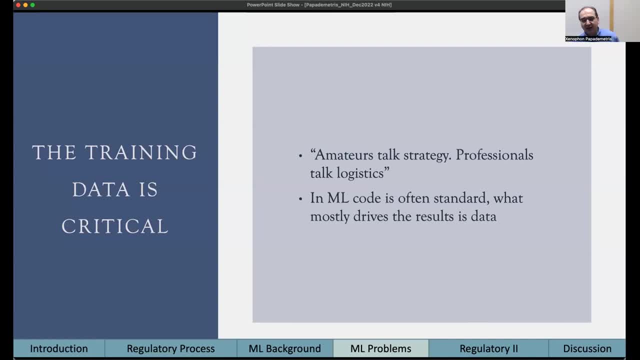 but training data is often more important In machine learning. the code is often standards over the same networks. The unit is the most common image analysis network. It's fairly commonly used. What often drives the results is the data, not the code. 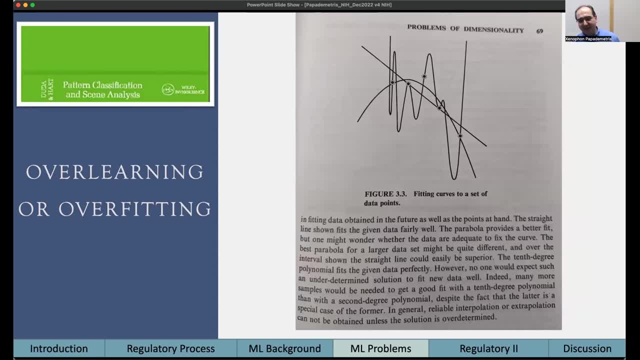 If you think about overlearning or overfitting back to Dudenhardt, back to 50 years ago, here's an example from the book that it's the same problem that we're still dealing with 50 years later. We have some measurements. 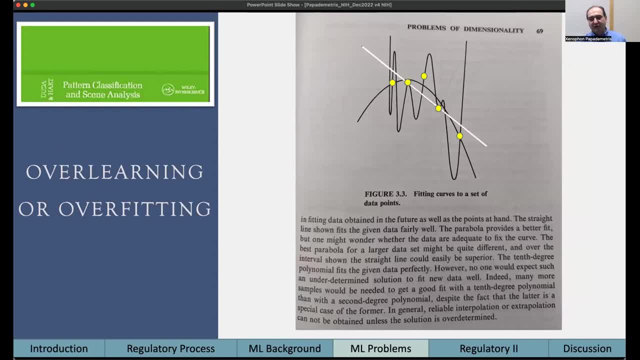 Those are maybe at yellow dots. We try to extract some patterns So maybe we fit a line. a linear regression has that sort of thing And we have learned something about the data. Maybe we think there's a little bit more we can squeeze out. 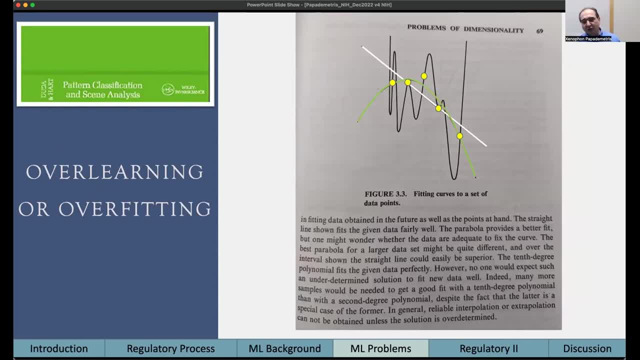 Maybe we fit that parabola, this green curve, So it goes up and down. So, who knows, maybe there's a better fit. If you go to extreme, you can fit a super highly nonlinear polynomial, And this fits our training data exactly. 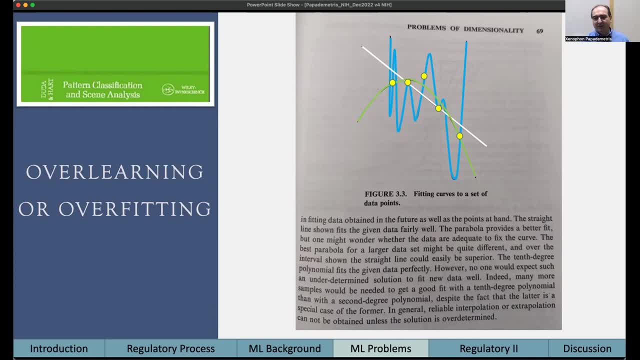 But the question, of course, isn't how well you fit your training data, these measurements, but what happens when you get another measurement there where the blue point is, So the prediction error? it may be vastly different between the three And, in general, if you overfit the data. 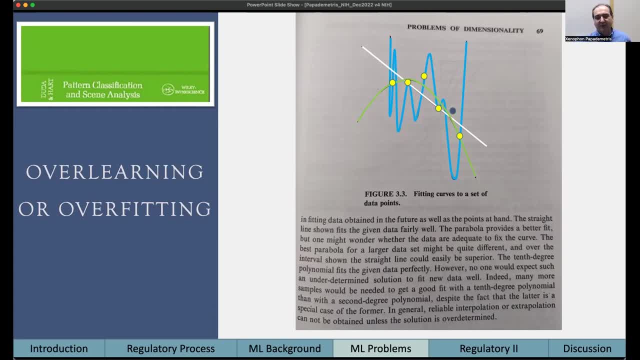 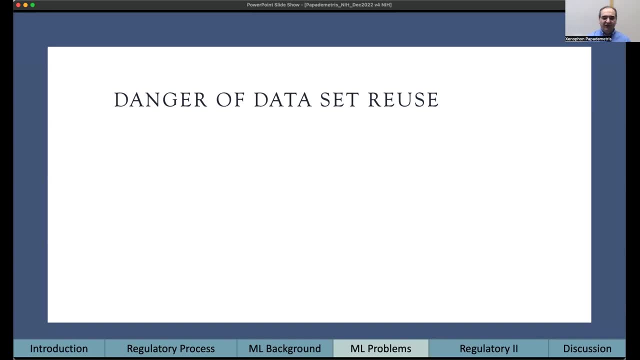 you get large generalization errors compared to fitting errors at the beginning. So keep that picture in mind. We'll come back to that as well. So as an aside, just from a research perspective, there's also here the danger of reusing your data. 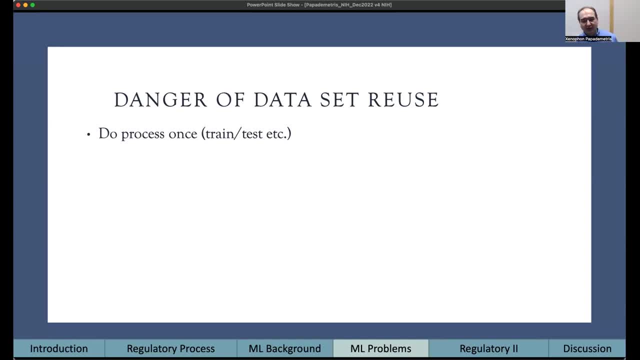 since too many times. So what I said, we do, we train, and we do the first ones. We train our neural network. We tested on the data We did once. so far, so good. Everything is clean. The results are not good enough. 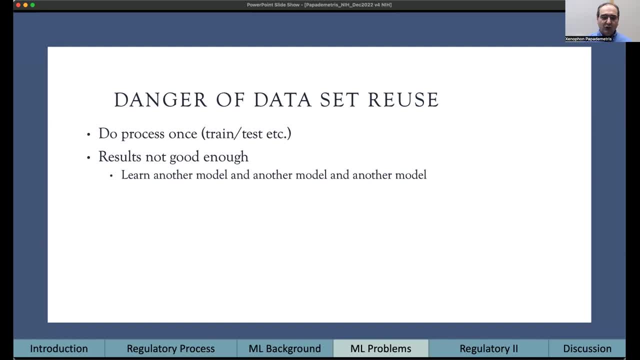 So we learn another model and another model and another model. And even though we don't mix training and testing data implicitly, we are. we get feedback from the testing data into our training set And training. multiple models can lead to overlearning from the data. 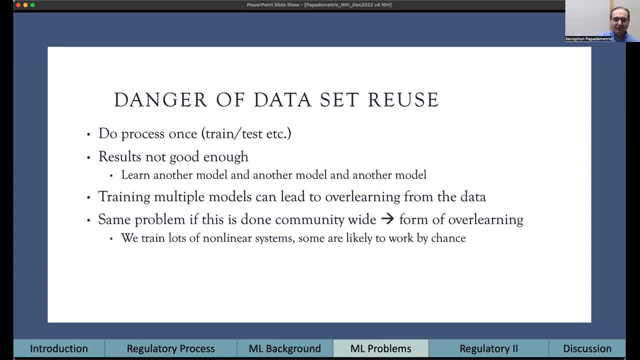 And this is the same problem. if we do this community-wide, it's a form of overlearning. We train lots of nonlinear systems, some of which are likely to work by chance. So back to my nonlinear case. if 50 labs train a nonlinear, 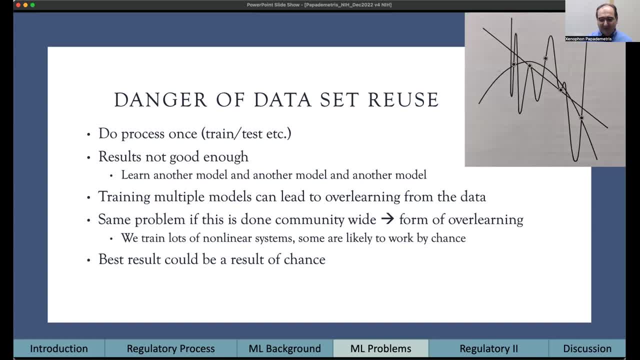 system of this data and we have 50 high order polynomials. by chance, one of them will generalize. But are we learning something about the data or did we just get lucky? Did we do? And in the social sciences, this form of training? 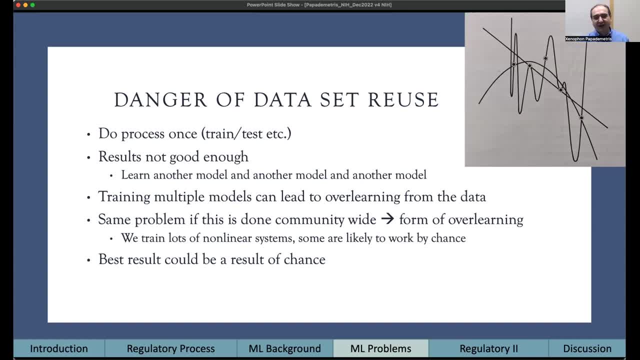 lots of models on the data and not doing public comparison. correction led to a crisis called pea hacking And I wonder if, in the machine learning, we're going to end up in a community while pea hacking, Are we really learning something? Or if 100 groups train on the same data? 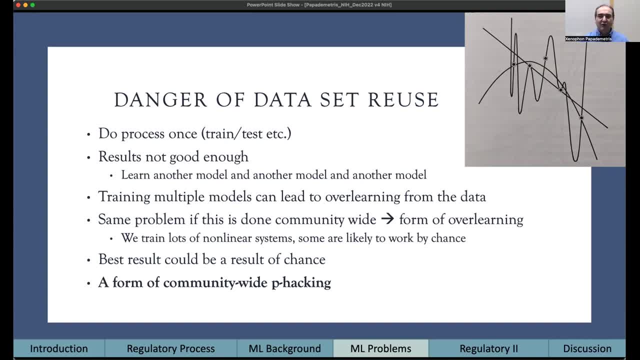 one of them just gets lucky. And as an aside to that, this is where we get into trouble with constant reuse of the same data sets. By the time, the 5,000 paper or the 10,000 paper is published on a data set, 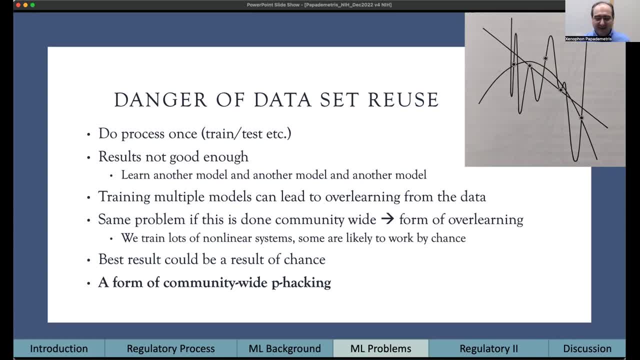 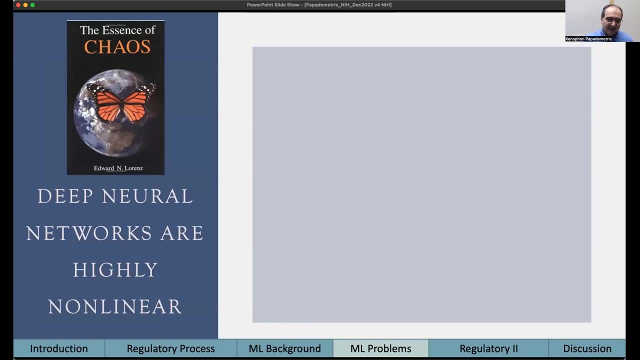 whether it's the Human Connection Project or ADNI or ABIDE or all of those things. are we studying the brain at this point, or are we studying the data set? So something to keep in mind- And we'll close that parenthesis here- Related to the problem of learning, is the fact that deep neural networks are highly nonlinear. 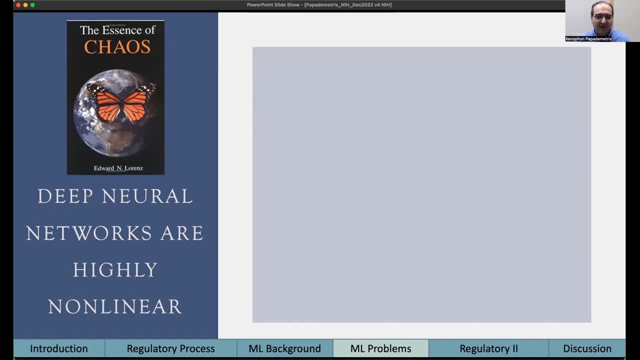 The picture you see on the left is the cover of this book by Edward Lorenz, The Essence of Chaos. Lorenz is sort of the father of chaos theory, And the summary of nonlinear systems is that small changes in the input can lead to large changes in the outputs. 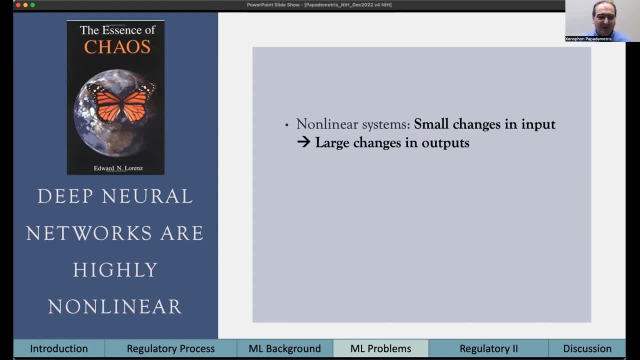 Back to the cover is the famous butterfly. A butterfly flapping its wings in the Amazon can lead to a tornado in Texas. This is sort of the summary of highly nonlinear systems. If you look at deep neural networks, each layer has activation functions which are nonlinear. 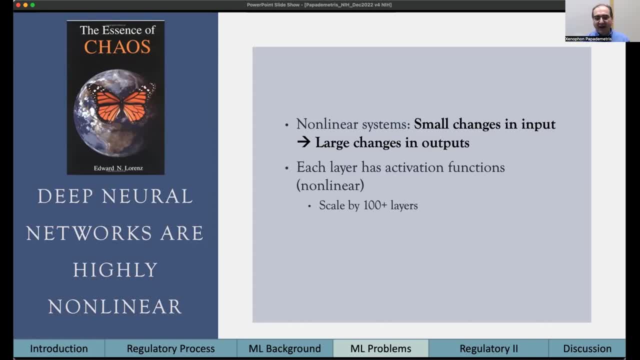 There's a threshold, a ReLU, what have you, And we may have a hundred layers. There's a ton of linearities joined one after the other, And the expectation, if we knew nothing else, is that these networks are going to be sensitive to small changes in the input. 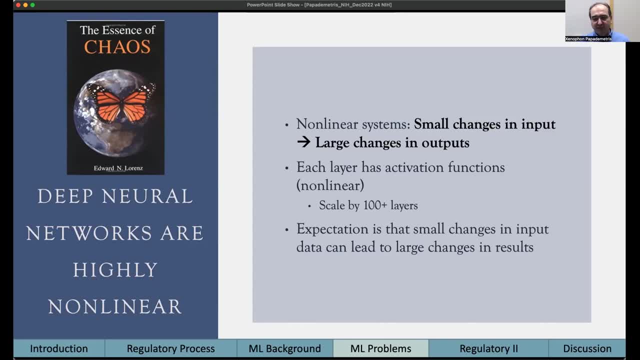 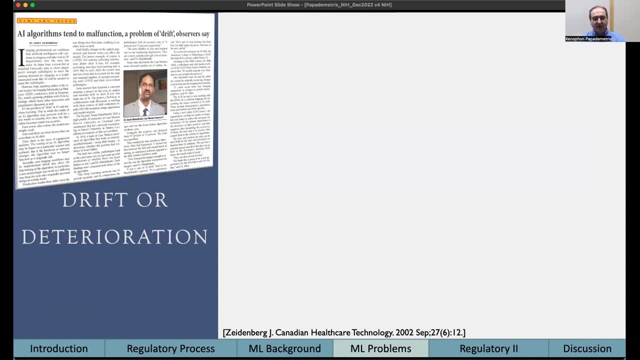 Small changes in the input data will lead to large changes in the results, And we're going to be in this domain. Do we see that? And the answer, of course, is yes, And I'm going to show you some examples. Here's a first example. 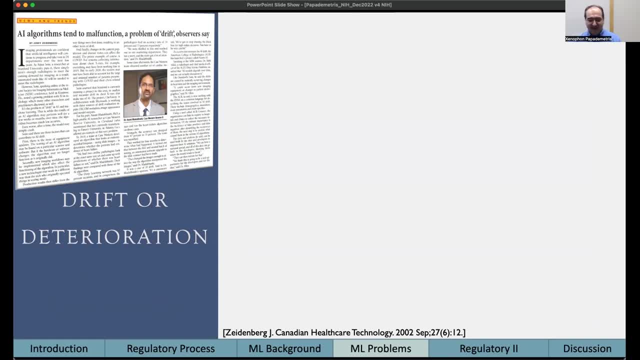 This is from an interview published in the Canadian Health and Technology Journal earlier this year And I'm going to quote from some of the from Dr Nath Madabushi, one of the well-respected colleagues at Georgia Tech. at the time he was at Case Western. 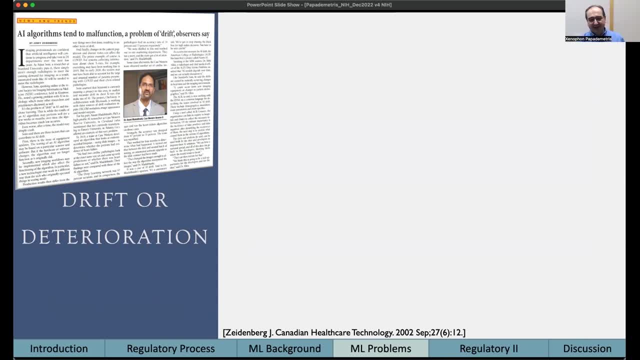 This work was done. I actually heard this story from him personally when he visited Yale. about the time this happened. He said in 2018, a team at Case Western, where he used to be, developed an algorithm that looks at endomyocardial biopsies using slide images to determine. 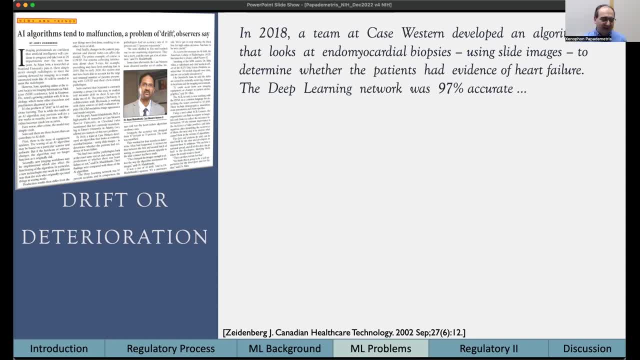 whether patients had evidence of heart failure And they trained a deep learning network and it was 97% accurate. It was significantly higher than the humans they had at the time, So they got really excited. Sometime afterwards they obtained another set of cardiac images. 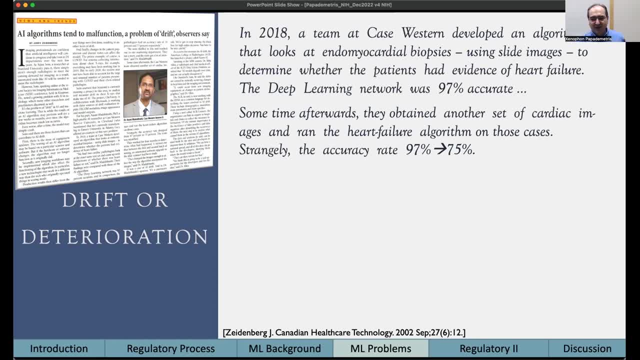 and they ran the same algorithm And, strangely, they got an accuracy all the way now down to 75%. So what happened? It turned out that between the first and second batch of testing there was an automated software upgrade to the slide scanner and that changed the images enough to affect the way. 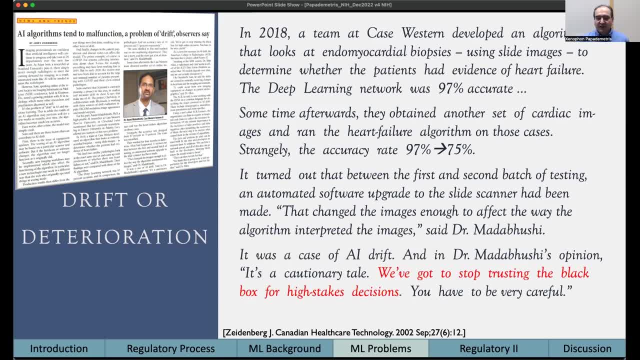 the algorithm interpreted the images And this is his conclusion. It was a case of AI drift, small changes in the input, small changes in the data And, in Dr Madabushi's opinion, it was a cautionary tale. You have to stop trusting the black box with high-stake decisions. You have to be careful. 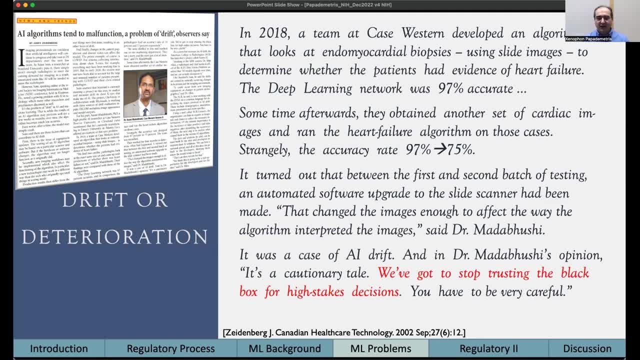 So here's a case where the only thing that happened was a minor upgrade to the scanner. It was enough to destroy this algorithm, And that's because, probably in the training they learn not only how the disease appears, but how it appears in the specific configuration. 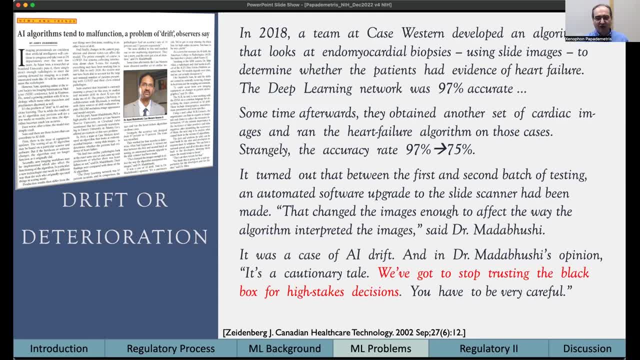 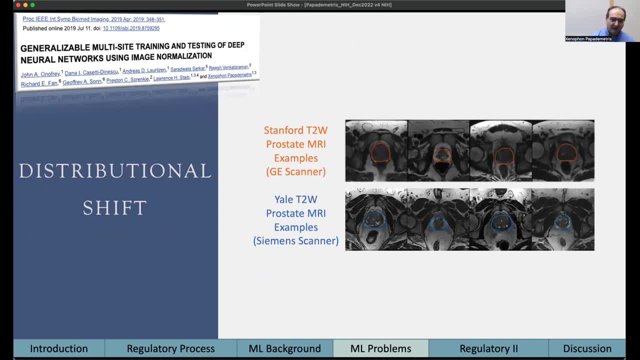 the specific software, the specific scanner. We made a small change of that and the overwhelming came through and that's what they call drift. Here's another example from our own work. We're trying to segment prostate MRI data. The top is a set of data we got from our colleagues at Stanford. 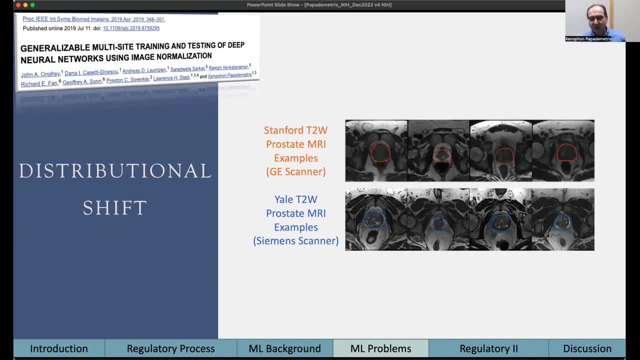 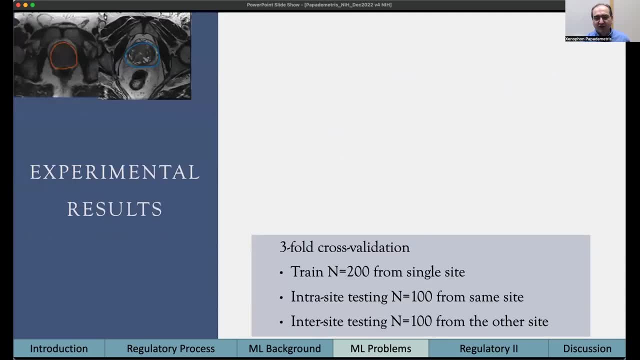 The more important part is from a GE scanner. The bottom is some sort of prostate data we got from our own data set at Yale- This is on a Siemens machine- And we trained a neural network to do this segmentation and we followed the right things. 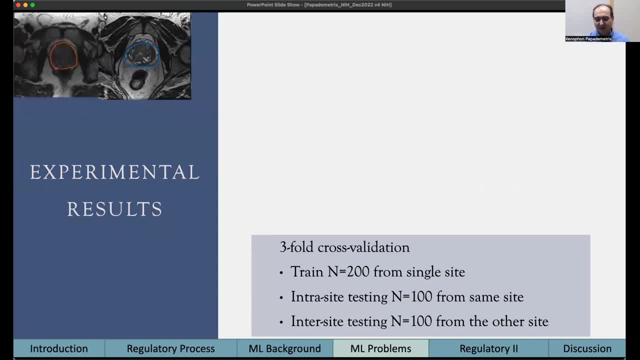 We did 3-fold cross-validation. We trained from a single site and we did testing either from the same site or another site. So if you trained on Stanford data, tested on Stanford data, trained on Yale data, tested on Yale data. 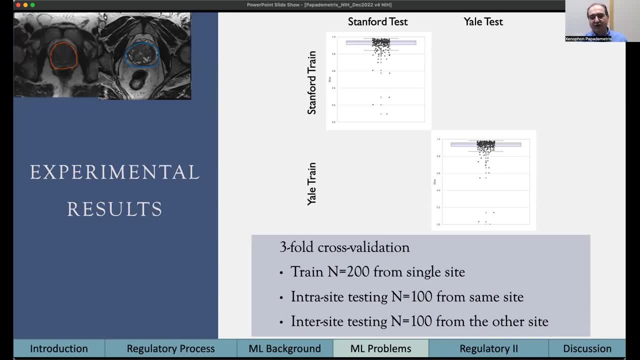 got really good results. accuracy: the median accuracy in the high 90s If you trained on Yale data tested on Stanford. we have some deterioration but you know still pretty good results. But the kicker was this final one: When we train on Stanford: data tested on Yale data. 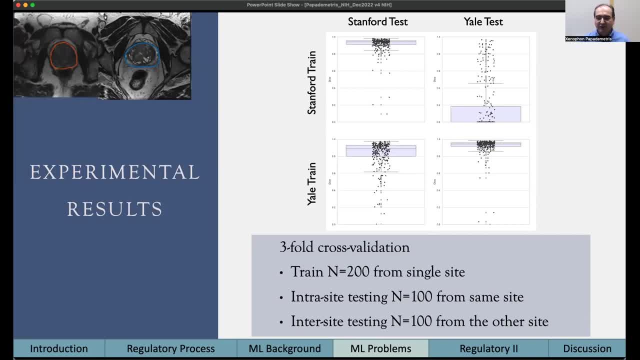 most of the subjects failed. The median accuracy was close to zero And again this was a case of the images were different enough from the two scanners that we failed to see that, And the lesson I took from this is that you can't really see anything reliable if all your data is from a single source. 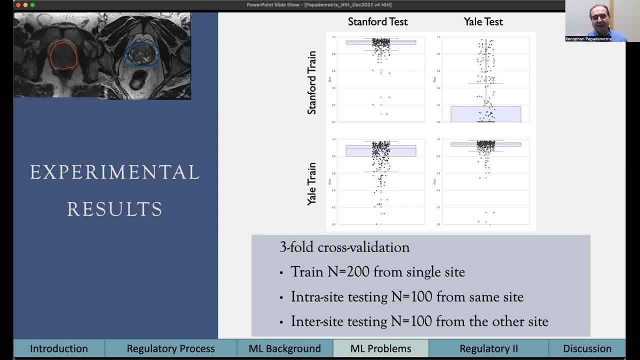 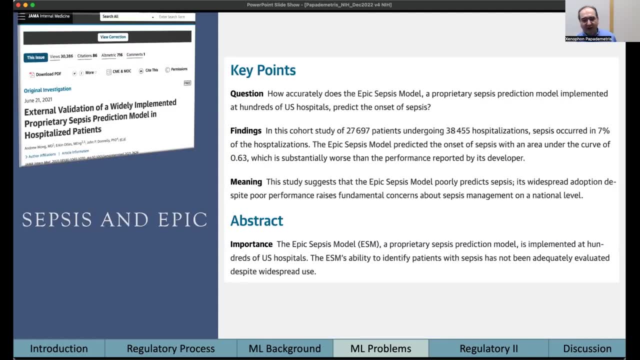 You have to do more sources. We were able to correct this by doing intentional normalization. It's a fairly easy problem as things go because of obvious failure, but keep that in mind. Let me give you another example From outside the imaging world, and this is the sepsis algorithm that's part of EPIC. 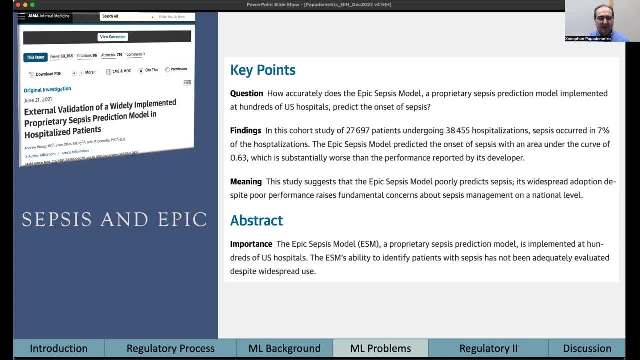 the electronic health record database and this was their proprietary sepsis prediction model. This is one of the major issues in hospitals: predicting which of the patients are at risk for sepsis and taking measures. So a set of researchers at the University of Michigan- you can see a team of Wong Ottles and Donnelly. 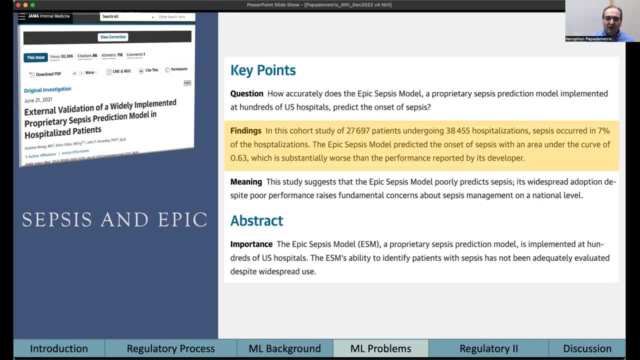 repeated the study with their own data And in a cohort of 27,000 patients undergoing about 39,000 socializations. they had 7% of carotid cancer, So they were able to predict the onset of sepsis. 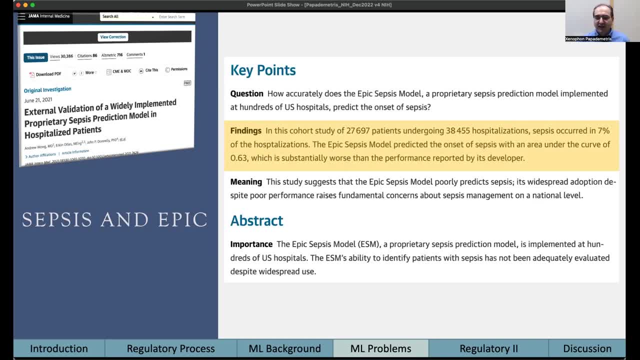 The EPIC sepsis model predicted the onset of sepsis with an area under the curve of 0.63,, which is substantially worse than the performance reported by its developer. The study suggests that this model poorly predicts sepsis and it was widely used at the time, despite performance. 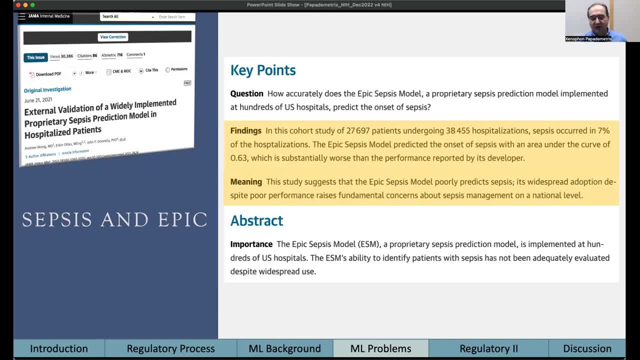 and raises fundamental concerns about sepsis management on a national level. They had to recall this model and retrain it. In the original work, the area under the curve was on the order of 0.8.. They got about 0.63.. 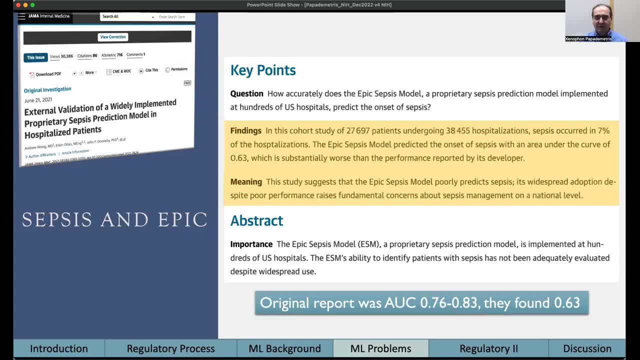 For those of you who don't think in area under the curves, at a very hand-wave approximation, an area under the curve of about 0.8 is the equivalent of a sensitivity and specificity of about 0.8.. 0.6, you can get that with a sensitivity and specificity of 0.6.. 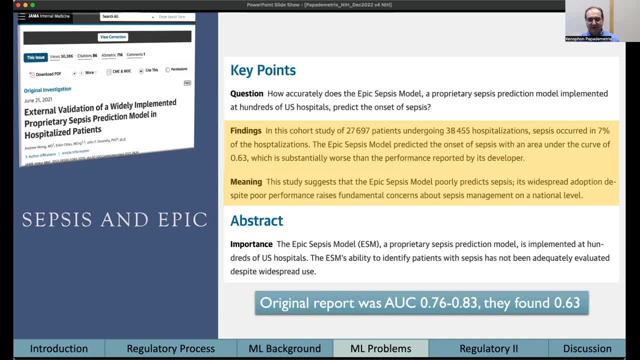 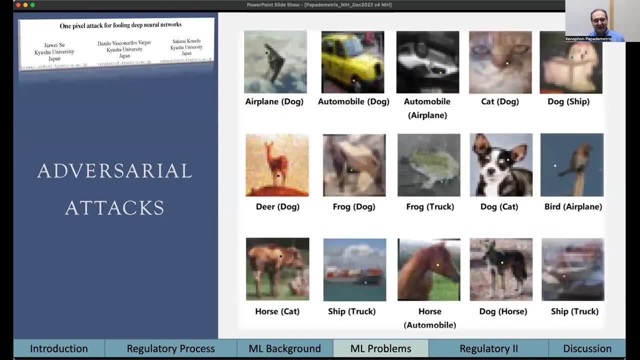 There are other ways to get the same area under the curve, But think about it: it's a 20% reduction in both sensitivity and specificity. So it's pretty dramatic. One One additional example that's kind of interesting. this is work from Sue Rackers and Grischi from the computer vision world. 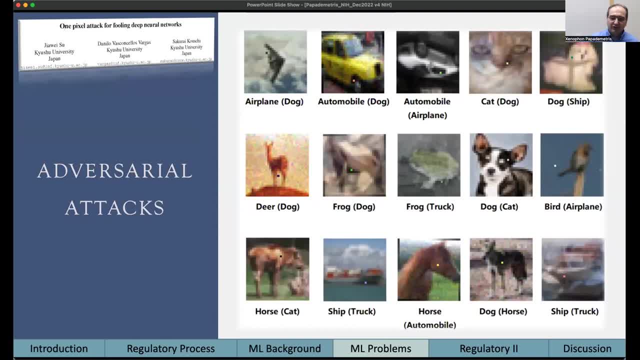 This is the one pixel attack work for fully neural networks. What you see here are images, And these were trained on a classifier and they were getting the correct levels, And then what they went ahead and did is that they changed a single pixel in this image. 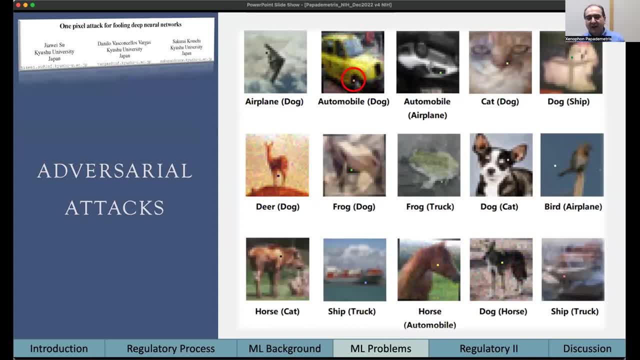 For example, in the image- the second on the top- they added that orange pixel on top of the tire And that was enough to fool a pre-trained classifier to report that this was a dog instead of a car. And they were able to do it with any pair of images: to get any label to any label by just changing one pixel. 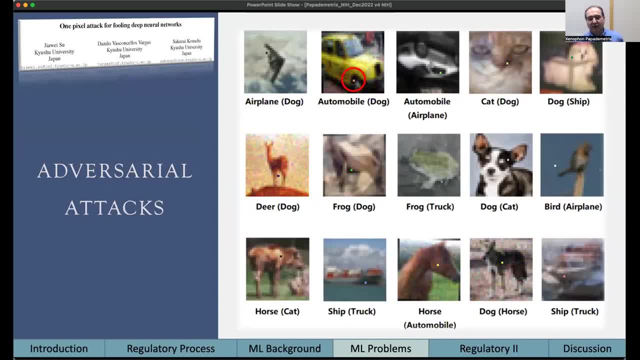 And this again is a case of a high non-linearity in these networks- Highly non-linear networks, susceptible to changes in the input- And they were able to demonstrate that it was a single pixel attack on all these things. One final example before we try to make sense of it. 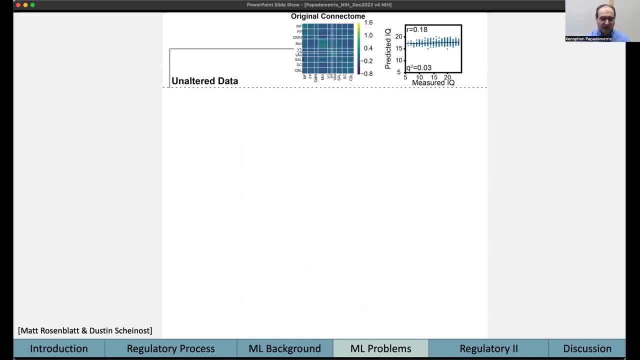 And this comes from functional magnetic resonance imaging, some published work from my colleagues at Yale. What you see above at the top is a connector. This is data derived from fMRI by averaging in the parcellation of the brain, And then they use this to predict behavioral measures outside the scanner. 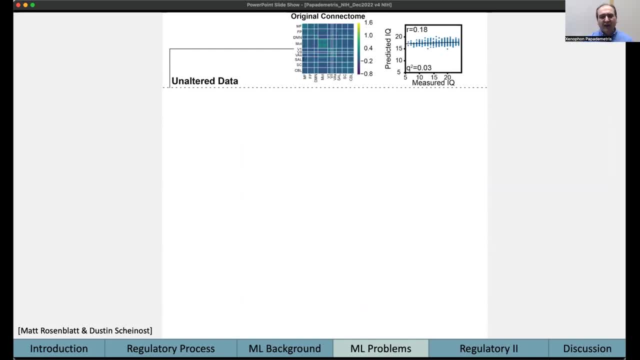 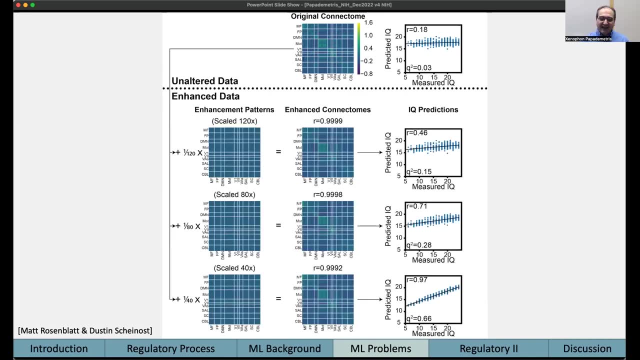 So can you predict IQ from fMRI against measured IQ? And you can see, in this particular data set the prediction was not that great. there Correlation was about 0.18.. They went ahead and they added a little bit of enhancement patterns. 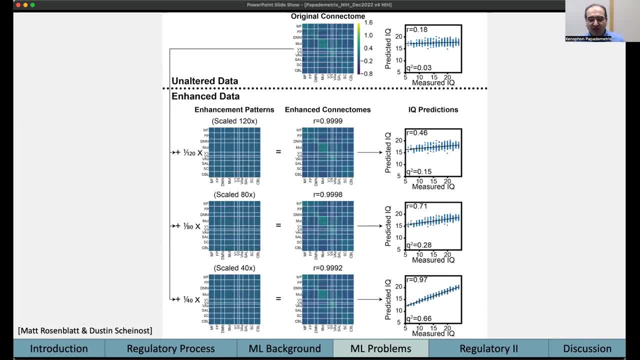 targeted enhancement patterns to the data. These are very small compared to the original data. You can see the correlations. those 0.99s It's how similar the corrupted data were to the original data. But that small data you can think of it as almost fraud, right. 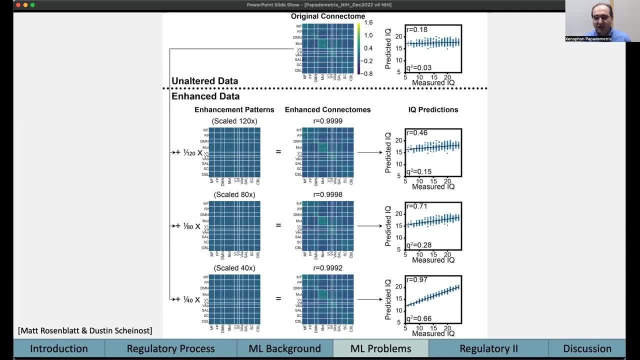 They're just showing how sensitive these algorithms are. Raised the IQ prediction from 0.18 to 0.46, all the way to 0.97.. This is a tiny change And, again, this is not a deep neural network. 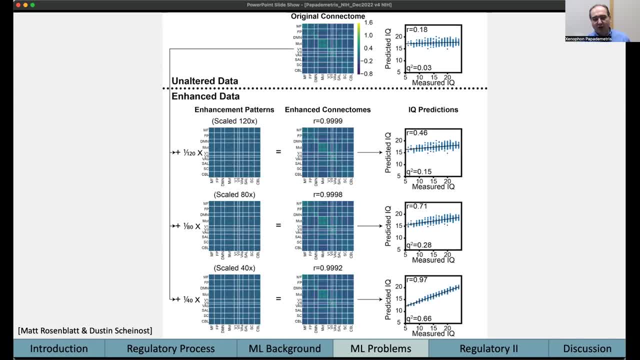 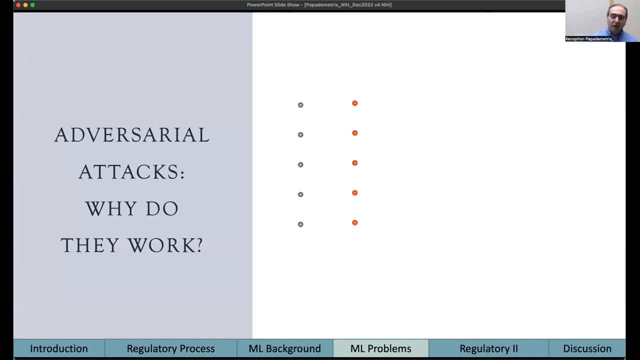 but it involves a significant number of non-linearities stacked together: Small changes in the input, Large changes in the output. Why do these things work? Why do adversarial attacks work? If you train a neural network, perhaps those are your data. 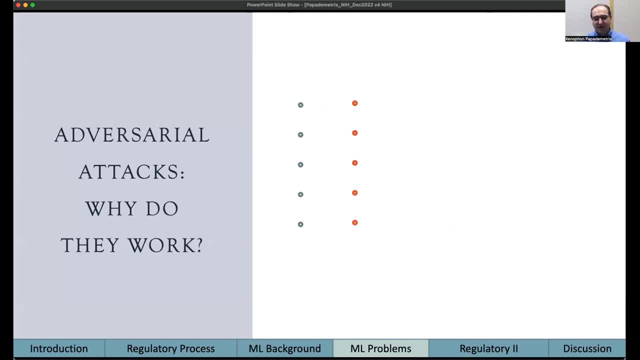 The green dots are your healthy controls. The orange dots are your patients. The problem is that, in the big empty space of all possibilities, all we know is the truth at the location of those points. So yeah, we think we may get a result like this. 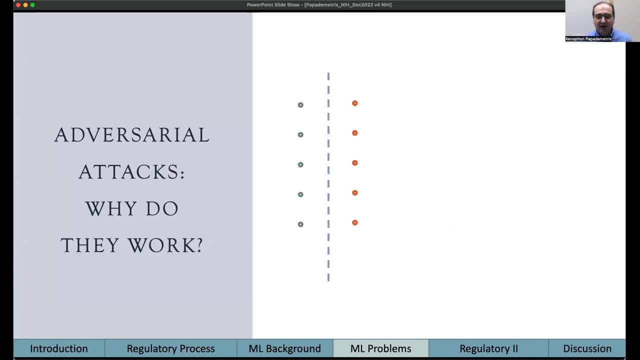 nicely far away from everything, And that's what happens when you run a linear classifier. You can specify how far away you can get from data, And so you're somewhat robust, But with a deep neural network, you may well end up with a classifier like this: 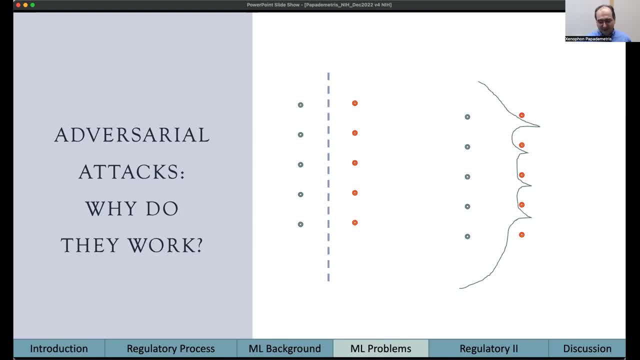 This has equivalent truth value than the other one. right, All the patients are on one side, All the controls are on the other side. The problem with the second classifier is it takes very little movement of the arrow at the top to shift it from one side of the classifier to the other. 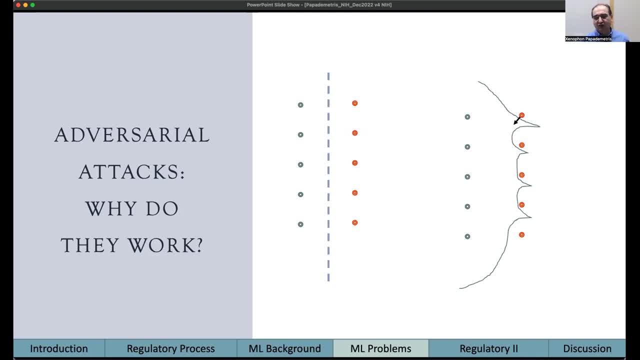 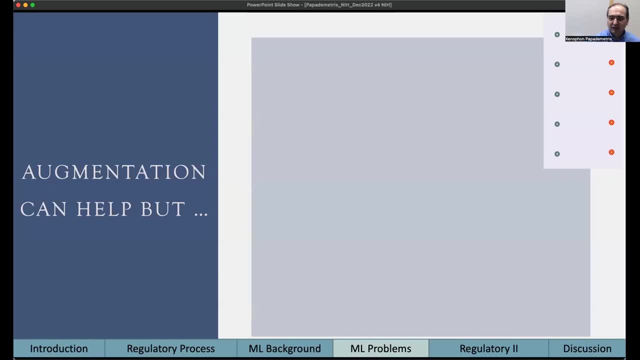 and to get an adversarial attack or to get an error. And again, this is a function of the non-linearity. you see, One solution to this problem is augmentation. So you take your initial data points, you see them on the right. 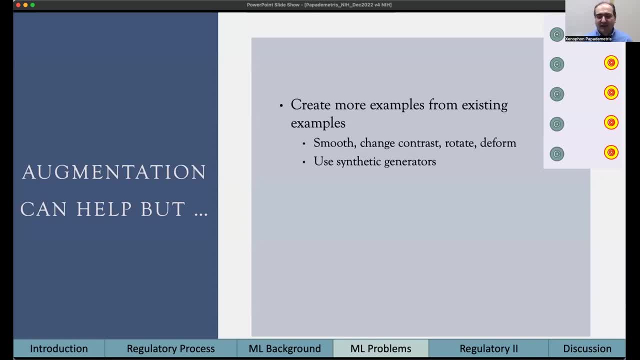 and you make them fatter by creating more examples from the existing samples. right, You smooth, you change the contrast, we rotate, we deform the images, we generate more examples. we can use synthetic generators And you know just at a high level. think of it as taking little dots. 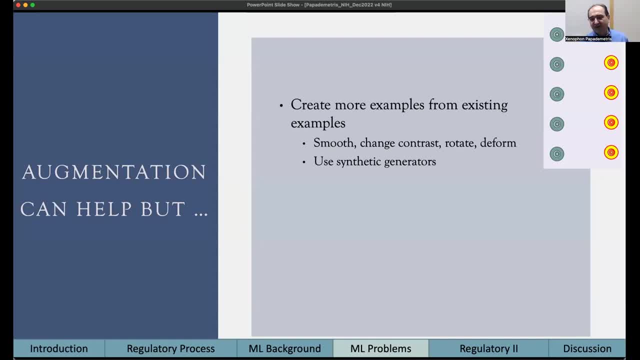 and making them fatter, and this gives you more points. So this kind of stability- and it actually in fact does work quite nicely, but I will assure that the creator who created synthetic samples maintained the same level. Did the change actually make it more like the other class? 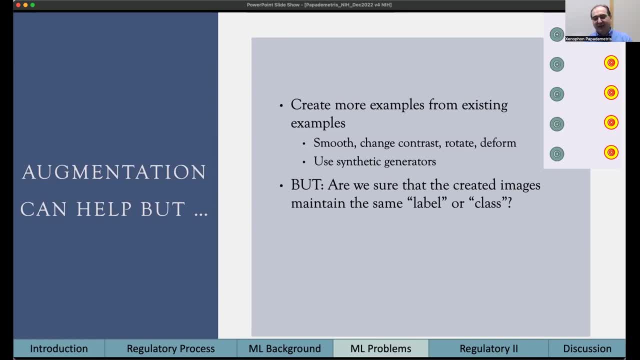 If you take a healthy subject and change its image, is it more like a patient now or is it still a healthy subject? Just to give you a couple of examples of what happens. we all learn deep learning on the digit data set, the digital recognition. 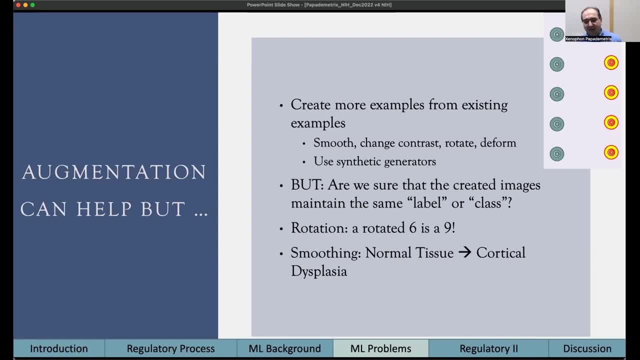 If you rotate a six, you get a nine, so you change a class. A more sophisticated example: perhaps let's take smoothing, If you look at epilepsy on the gray-white boundary. one of the structural abnormalities of epilepsy is cortical dysplasia and this manifests sometimes. 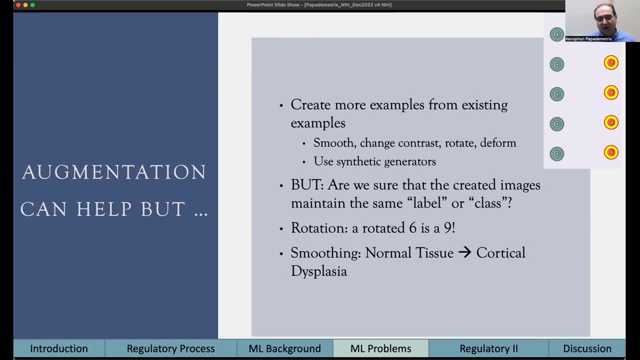 as a blurry, gray-white boundary. So if you smooth normal tissue, you actually get something that looks like a cortical dysplasia. So augmentation is helpful, but it's not perfect and we need to be careful about that as well. So we've seen some of the issues. 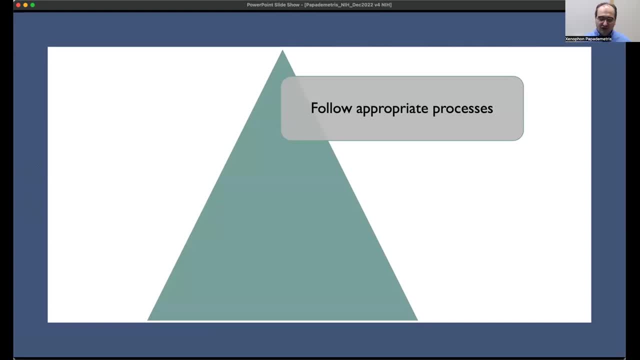 We know that we need to follow appropriate processes and the risk classification and all of that. but let's look at a couple more things from the regulatory process. This is the last major chunk of the talk. We'll talk about how to evaluate, to establish trust. 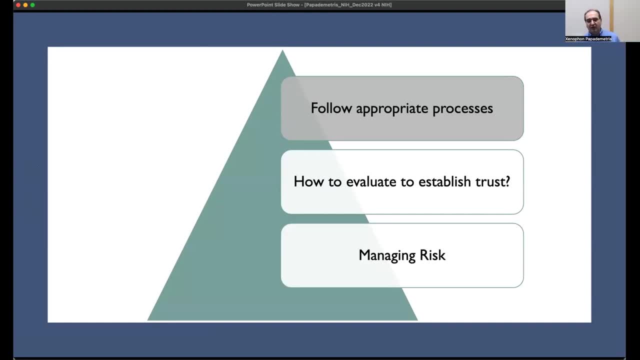 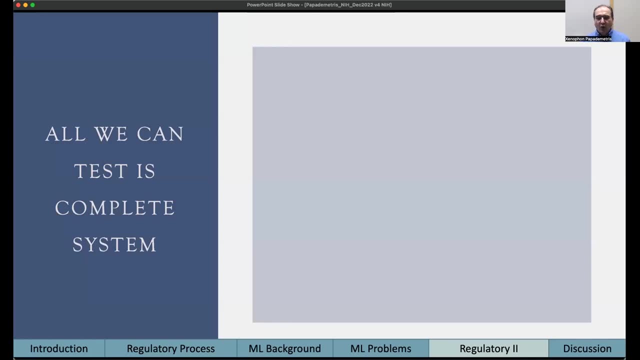 and we'll talk a little bit about managing the risk. You know, can we live with the mistakes? Maybe we can in some cases, and sometimes it's the easiest thing to do. One of the issues with machine learning systems is: all we can really test is a complete system. 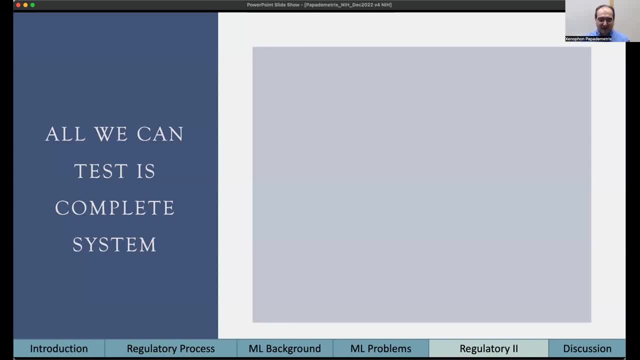 Unlike regular software, we can check all the components and test function by function and make sure every function works and then put them together In deep learning. all we have is like the black box input output. So given the series of those, 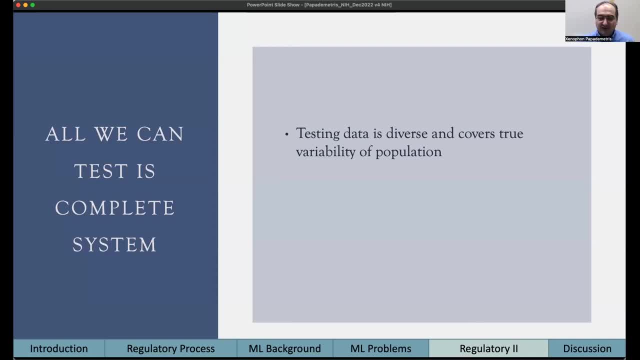 we really need to make sure that our testing data is diverse and covers the true variability of the population. We don't just test on the subset of the population, The old story about drag studies only being done on college undergraduates and not working on older people. 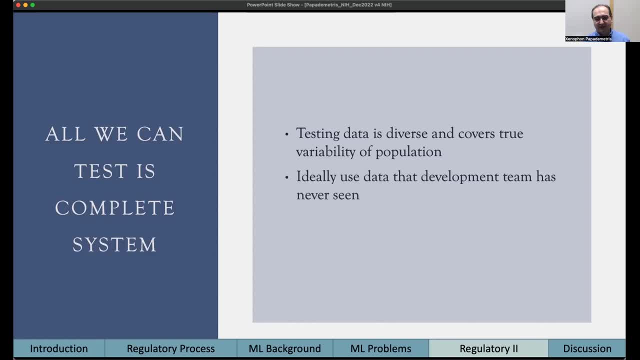 applies twice as hard here because of the non-linearity. Ideally we want to use data to test that the development has never seen. If it's a serious high-risk operation, maybe this case for prospective data or separately data from another location, And this is hard for us. 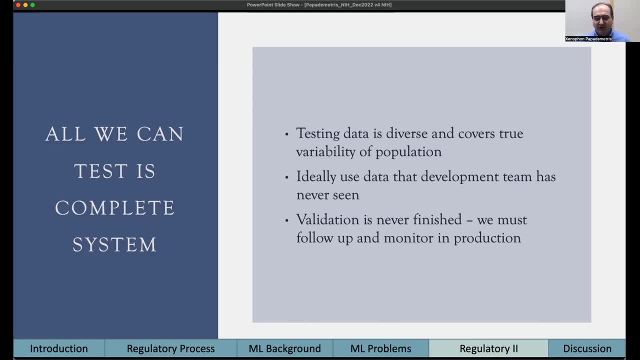 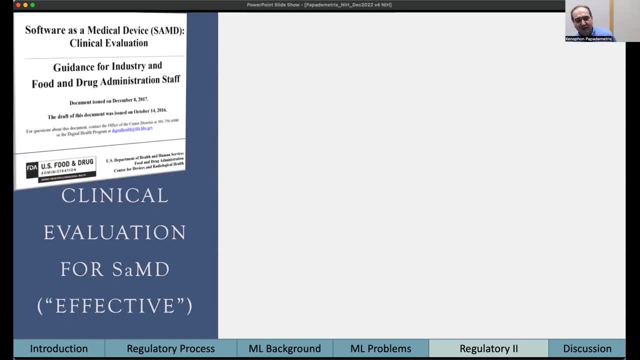 It's in research, but we have to realize that the validation is almost never finished. We need to follow up and monitor in production And you can see some of the echoes of the regulatory process there. One of the documents the FDA has this now dates six, seven years. 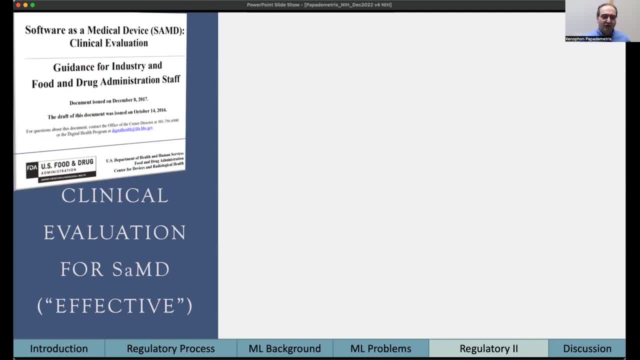 depending on when you count the drafts. This is one of the evaluation documents for software as a medical device. This precedes the deep learning era, but the ideas are still valuable. So they want to see three things as part of your evaluation. The first one is to establish what's called 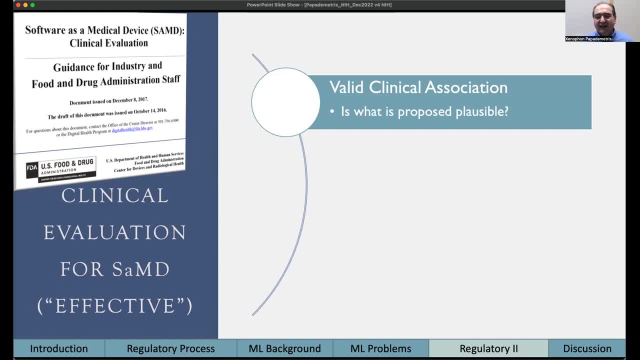 valid clinical association And so crudely spoken. is what you're proposing plausible? Are you measuring something that's somewhat hopeful for this disease? We'll get an example in a minute. Is what you're measuring accurate? This is the analytical validation. 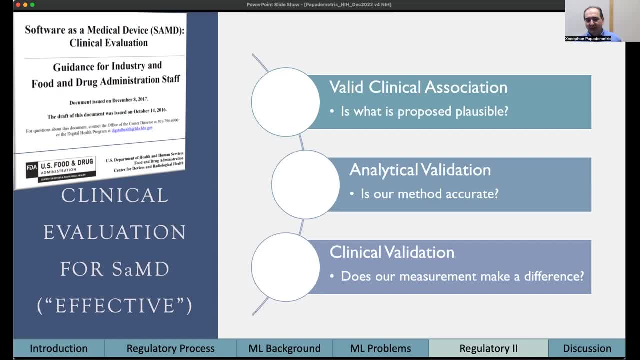 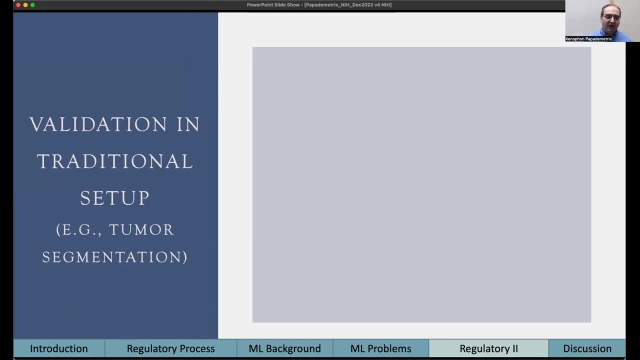 And then the third component of that is the clinical validation. Does your measure make a difference? So, is it plausible? Is it accurate? Does it make a difference? So let's look at an example. Let's take again a traditional algorithm. We're doing tumor segmentation. 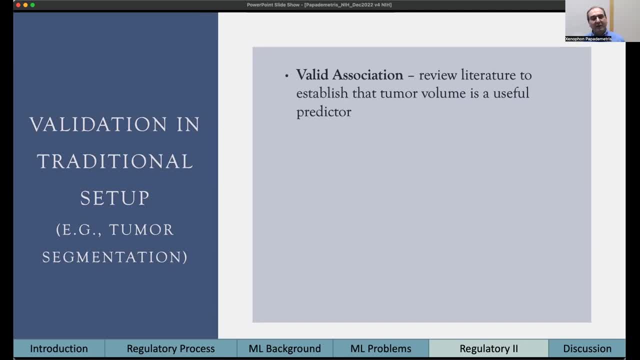 So what do these things look like? Well, the valid association may simply be a literature review to establish that tumor volume is a useful predictor in managing the disease: Small tumors manageable. large tumors highly risky, et cetera. That type of thing. 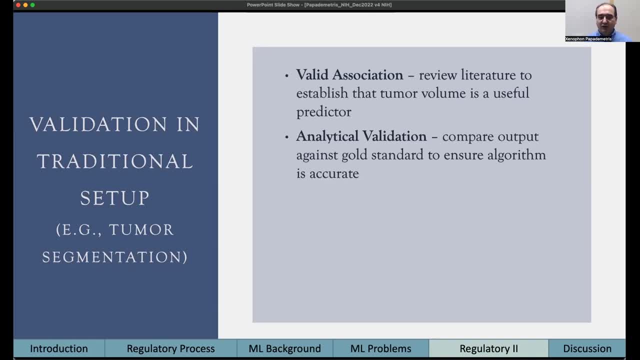 Your analytical validation may involve comparing the output against some gold standard to ensure that your outcome is accurate, that your segmentation result is correct, And your clinical validation may mean apply this method to a new data and see if this measurement is helpful in stratifying patients. 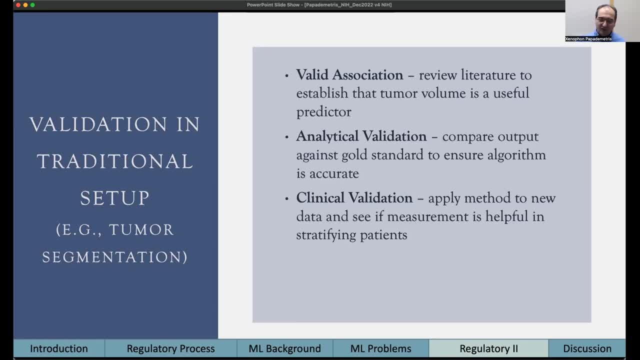 Just because you can get it accurate accurately and just because you measure something that's relevant doesn't mean it's actually useful in a clinical sense. Finally, if we get out of this document and go back to the rest of the guidance, we have to worry about safety. 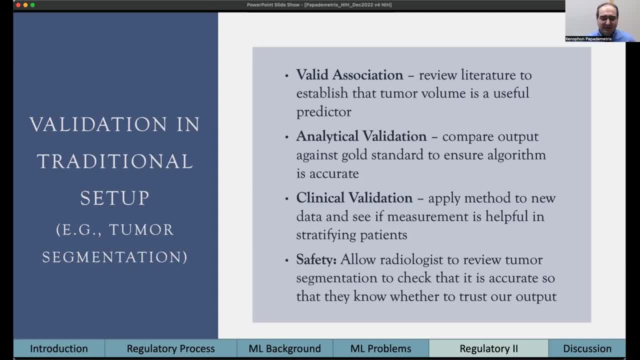 Safety means in software mostly usability, that we don't cause the doctor to make a mistake. So perhaps in this case we would allow the radiologist to look at our overlay of the tumor on top of the image and check that these are accurate. 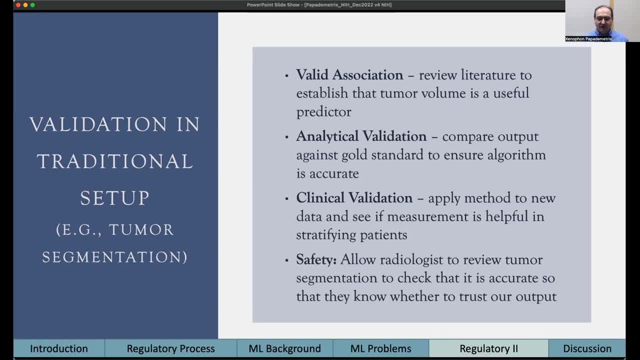 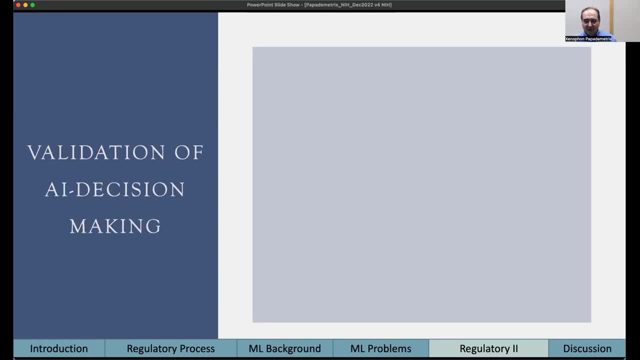 so they know whether to trust it or not. So this is what we think the tumor is. This is the image. You look at them together, You can say: yes, it didn't work, nor did everyone. Now let's look at this one step up now. 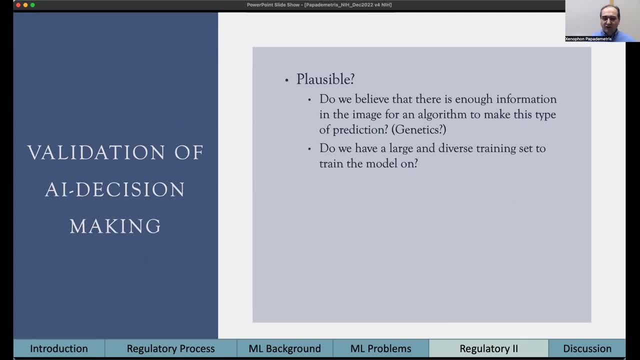 in the context of AI decision-making. Is it plausible Now? do we believe that there's enough information in the image for an outcome to make this kind of decision? Is appearance from the image enough? Maybe the same thing could be very different depending on the underlying genetics. 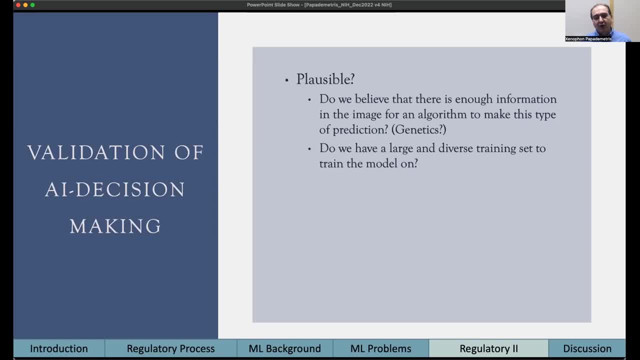 So it may not be plausible or not, but we're trying to squeeze in more. Do we have a large and diverse training data set to train this model? And if we don't now, can we really predict disease outcome from 20 patients? 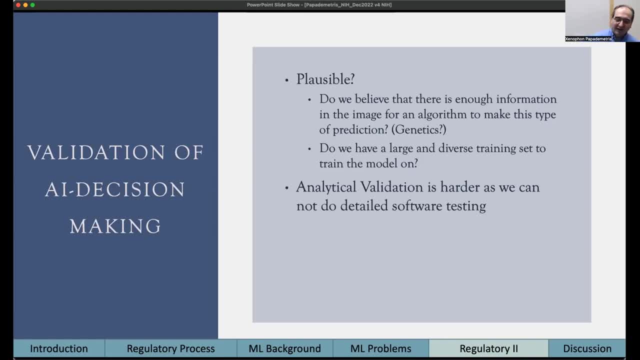 That's questionable. Analytical validation is harder because we cannot do the detailed testing. We can check only the final results. so we're a little bit more limited here. The clinical evaluation is the same as before, but even the relative lack of analytical evaluation. 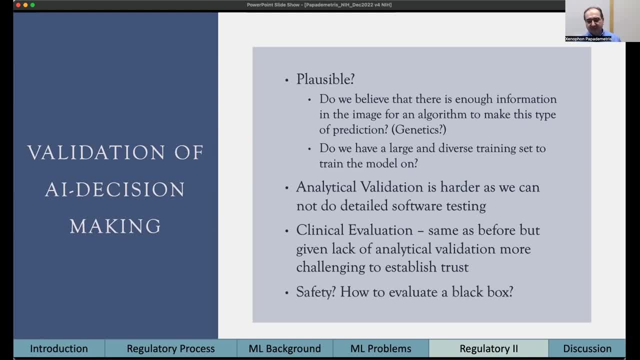 it's more challenging to establish trust here And safety. how do we evaluate a black box? The algorithm tells you that this patient is at high risk of getting Alzheimer's Deep down. this came out of a black box, unable to examine what it did. 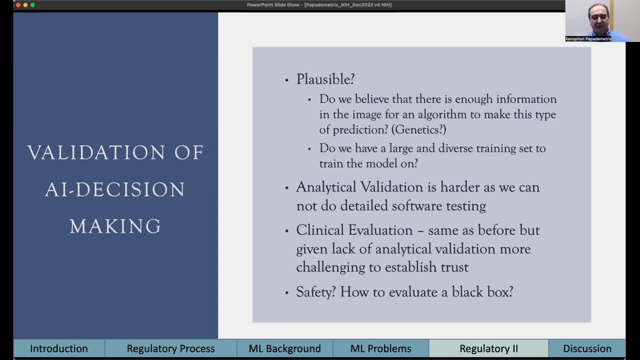 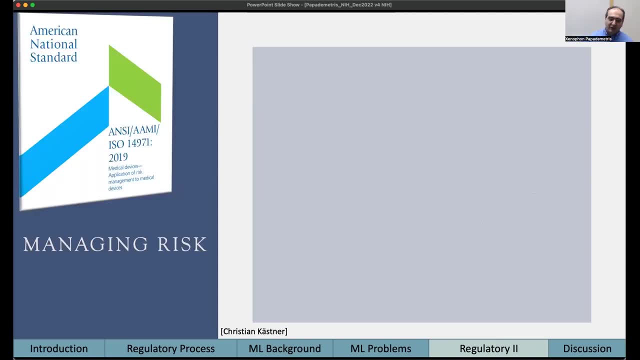 but not in the same way as something has. well, we tell you: the tumor is here and it's here, right? No human knows how to do that. The final part of this talk. before we get into discussion, we'll talk a little bit about the risk management process. 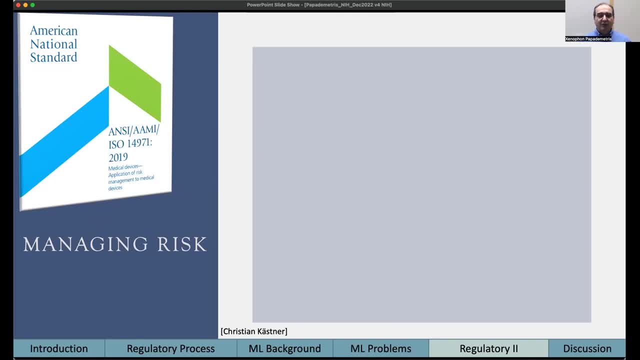 and how we manage risk. Risk is something that goes bad- and how to control it, how to make sure that, if a bad thing happens, it doesn't have downstream effects on our patients. In machine learning, we can do this at three levels. 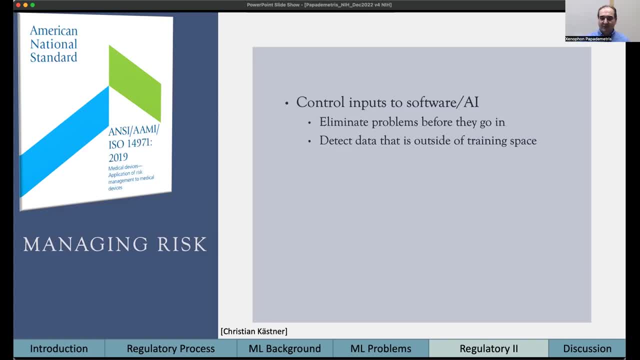 We can control the inputs of software, AI, we can eliminate problems before they go in. Perhaps we realize that this image is not like any other image we've trained in, so we can just issue a warning right. Our outcome is unlikely to work here. 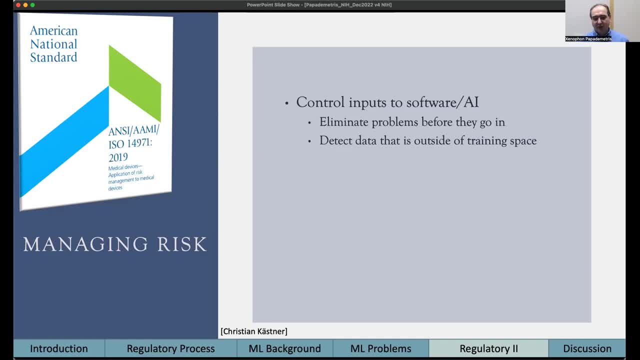 It's from the wrong scanner, the wrong resolution, the wrong contrast. what have you? You can do things to make the system, the deep learning neural network, less sensitive. There are training methods. I think that's less hopeful, and you can provide checks. 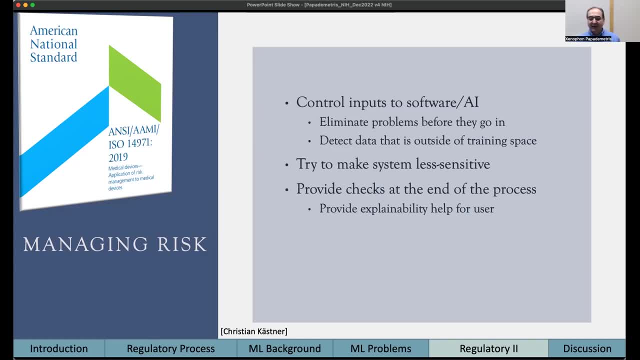 at the end of the process, And this comes under the rubric of explainability, And we provide some explanation to our user as to what the network did so they can evaluate the results. My colleague Christian Kastner, Carnegie Mellon always talks about. 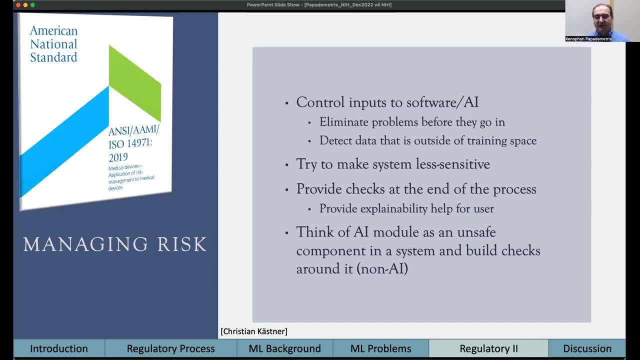 one should think about AI modules as unsafe components in a system and build checks around it, And these checks have to be almost non-AI things that we can fully trust So we can manage the process. we can build checks and balances outside the neural network. 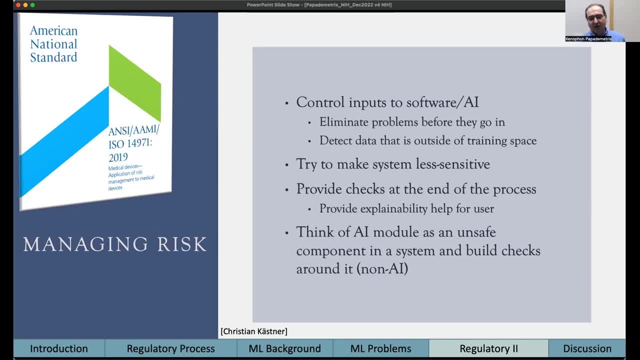 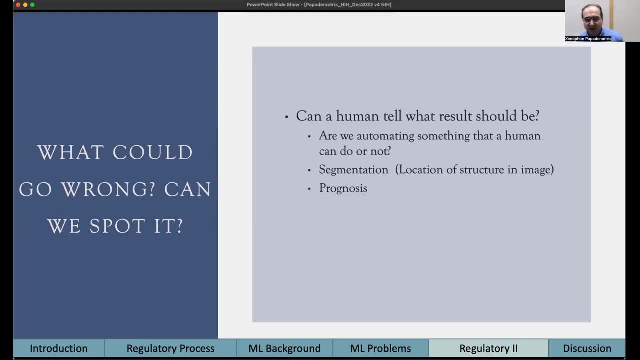 to detect if something is going wrong and solve for some warnings. What could go wrong? Can we spot it? The biggest challenge: if we're relying on humans as a risk management strategy- human in the loop type approaches- can a human even tell? 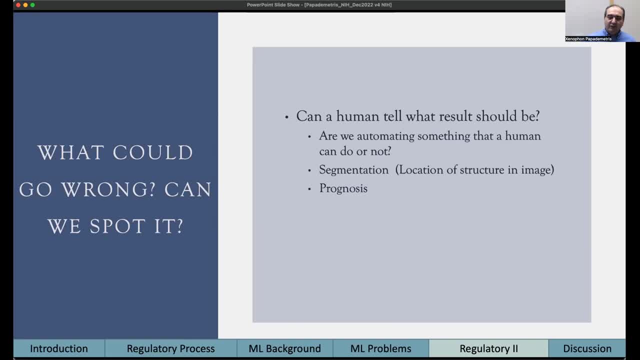 what the results should be. And this is easier when we're automating something. a human can do something like segmentation. So this is where you know a particular part of the structure of the brain is in the image. This is where the tumor is in the image. 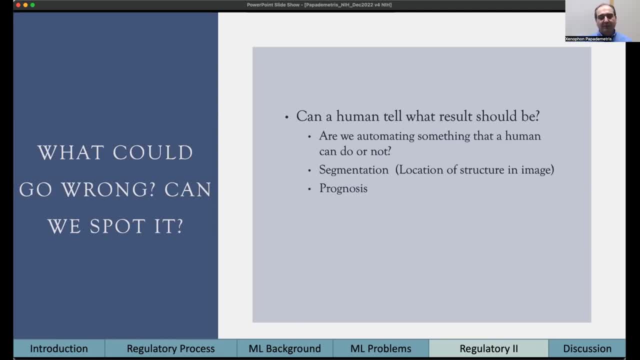 because a human could theoretically do that. It would be slower, it would be perhaps less accurate, but they can certainly check. If we're doing something like prognosis for future outcome of a disease, there's a much harder problem because humans already can't do that. 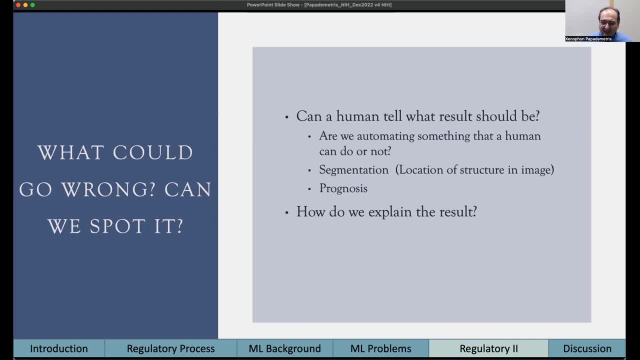 So that's a harder thing to do. Can we explain the result Now? given this super highly non-linear neural network, can we really come up with a number that helps you see what it did? That's a questionable thing, And in the literature, 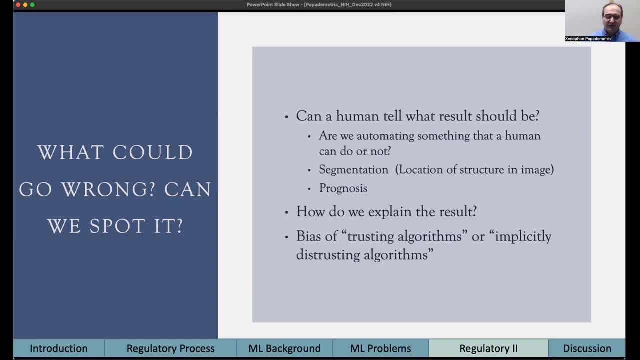 there's a whole debate about the bias of trusting algorithms or distrusting algorithms. Some people believe computers more. If a computer came up with the results, they believe it more. Others implicitly distrust computers if the result came from a computer And the literature is a little. 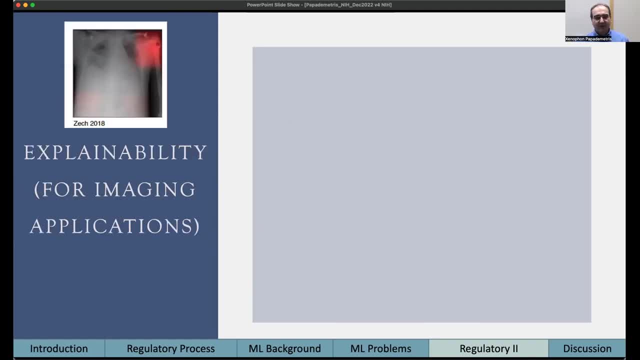 conflicted here, but it's an open problem, as you can tell. So let's look at one example of explainability for imaging applications. This is an example of a neural network that was trained to detect some particular kind of lung disease, And you can interrogate the network. 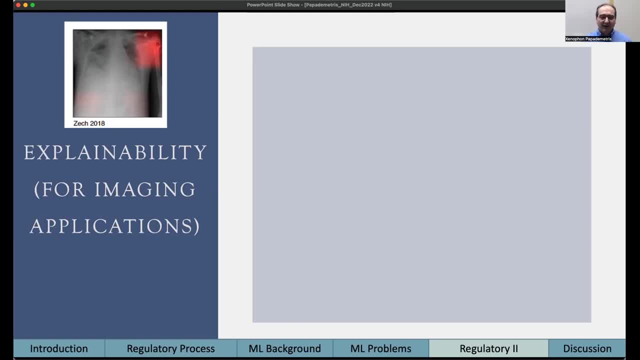 to see what parts of the image play the most role in its decision. In this particular case, it was looking on the shoulder, So that's in case of this is what's known as a heat map or a salience map, And you can tell by looking at this. 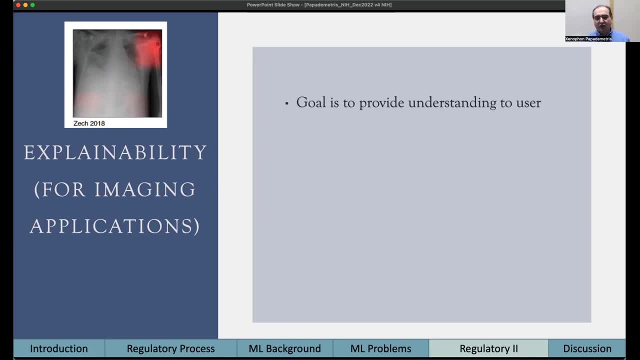 that the neural network is looking at the wrong place and probably shouldn't trust it. So the goal is to provide understanding to the user, And sometimes it's very useful. So in the case on the left, even though the algorithm is looking at the shoulder, 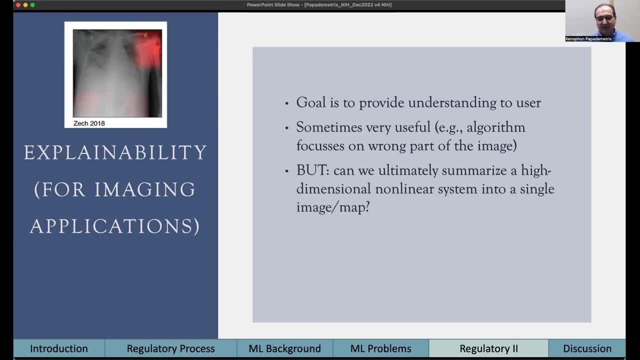 and not on the lung. probably shouldn't trust it for the diagnosis of lung disease, But can really summarize a high dimension non-linear system with millions of parameters into a single image map. Sometimes we can and sometimes we can't. And the other problem. 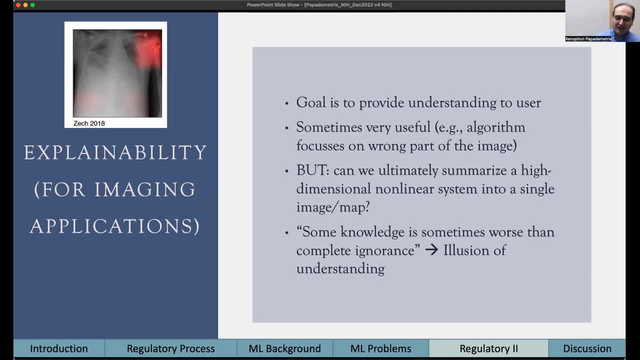 that comes up with explainability is this sort of Alforez, and Grieg is very famous. Some knowledge is sometimes worse than complete ignorance, And this is the illusion of understanding. So what if our algorithm showed that it was looking at the lung? 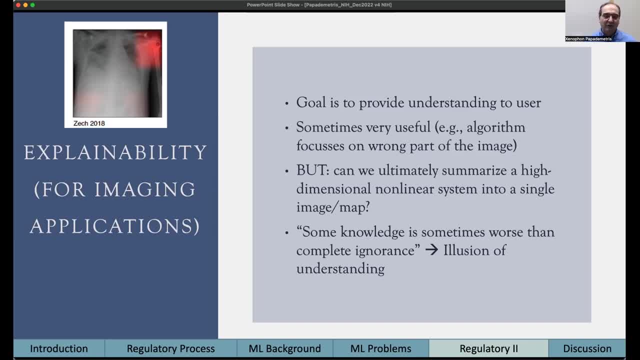 It doesn't really mean that it interpreted the image correctly. It means it was only looking at the right place. So if you had the explainability and it told you it was looking at the right place, maybe you're more inclined to believe it. 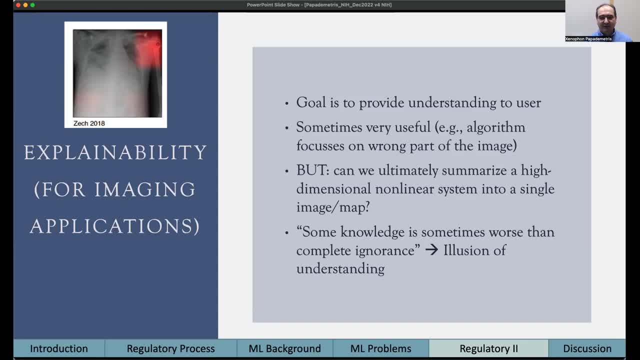 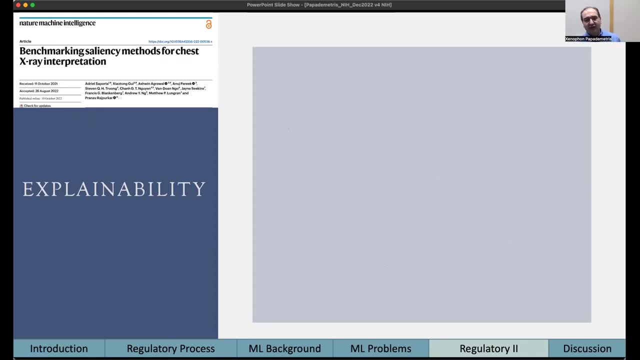 but for no good reason sometimes. So these are some of the challenges of explainability, So I don't think that's going to be the panacea at the end of the road here. Just to say one more slide on explainability. There was a recent study. 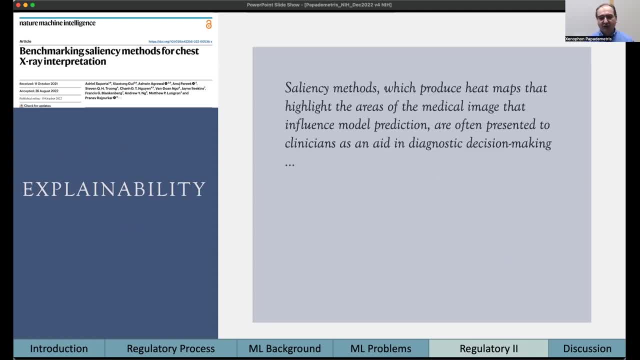 where they did benchmarking of methods for chest x-ray interpretation- And this is from their abstract Saliency methods- produce heat maps that highlight the areas of the medical image that influence model prediction are often presented to clinicians as an aid in diagnostic decision making. 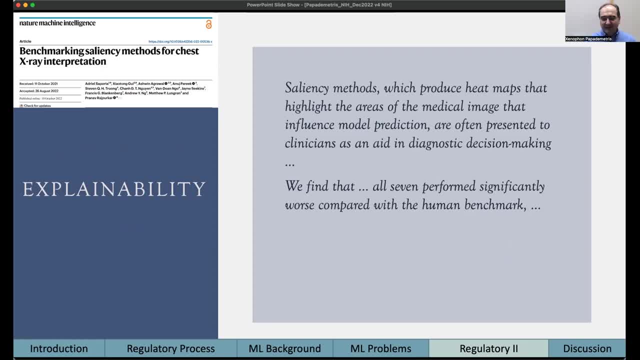 These people tested seven methods And while one did better than the others- for our purpose at least- all seven performed significantly worse compared to the human benchmark And their work demonstrates- and it's a very interesting paper- that several important limitations of saliency methods. 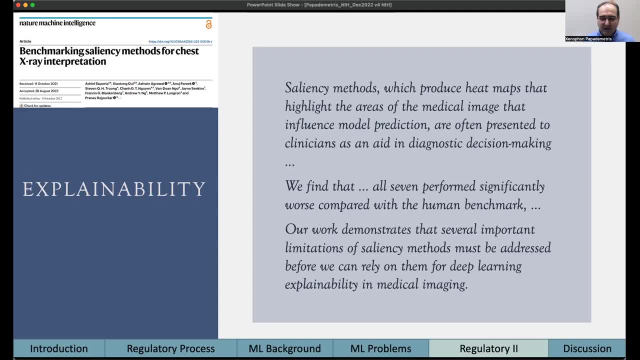 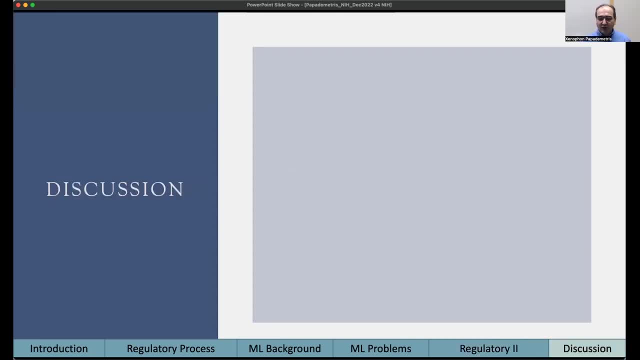 must be addressed before we can rely on them for deep learning. explainability of medical imaging. So explainability is important when it works, but we can't trust that either. So just to wrap up the talk, I have four more slides. I think we're okay. 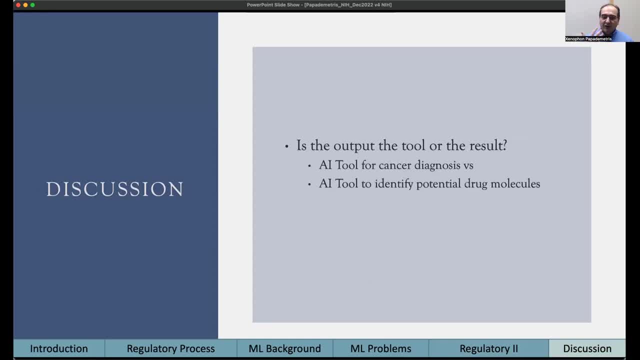 time-wise here. The first question sometimes to ask when you say, can we trust this thing? is whether the output is the tool or the result. If we're doing, we have a tool that helps you diagnose cancer or Alzheimer's from an image. 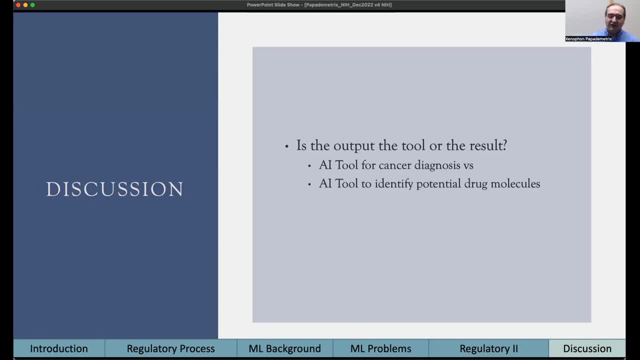 here the tool is the result. So we have to learn to trust the tool. and it's a more difficult process If the tool is used to give you a lead into something else, to identify potential drug molecules or some interesting work in that area, which you then test separately. 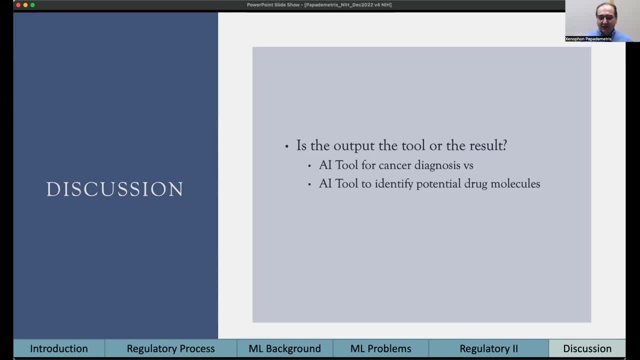 then maybe trusting the tool is less important, because the actual outcome isn't the tool, but the tool gives you some input into some other process. Can we afford to be wrong? What if we got it wrong? Can we mitigate or manage the risk? 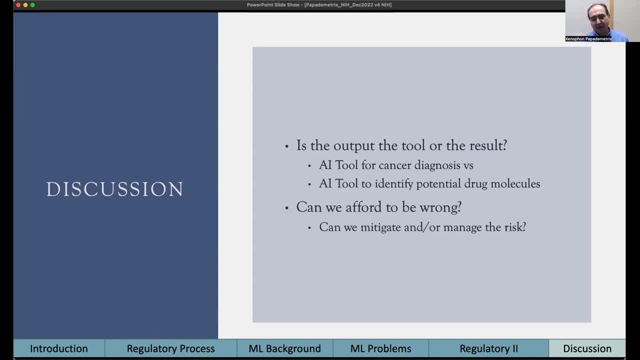 In some cases we can, in some cases we can't, and that will determine what happens. Back to my sort of take-home slide. it's not what the tool does, but what it will be used for. So let me give you three examples. 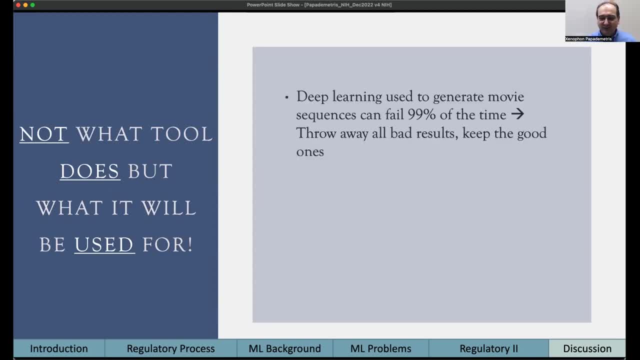 Those of you who are Star Wars fans may have heard that they use deep learning to generate some deep fakes for one of the recent Star Wars movies. Deep learning used to generate movie sequences can fail 99% of the time. That's not a problem. 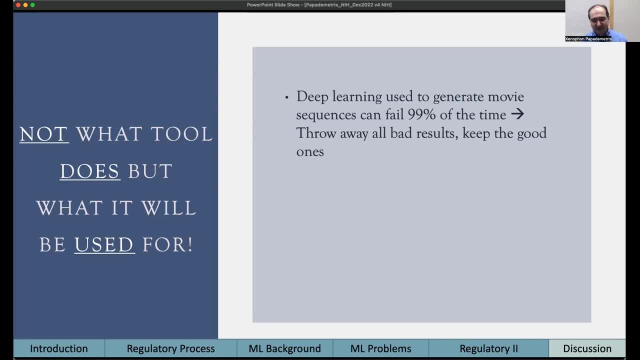 You throw away all the bad results, you keep the good ones and so long as you did it in a reasonable amount of time, you can use it and you're happy. Perhaps closer to medical if you have thousands of images for a clinical trial. 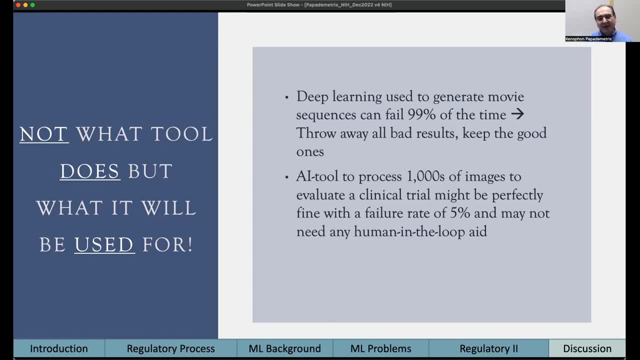 or a giant study and use an AI tool to process them, you might be fine with a decent failure rate and not require a human to check it, because maybe the error average is out, so long as the tool is mostly accurate. So, on the other hand, 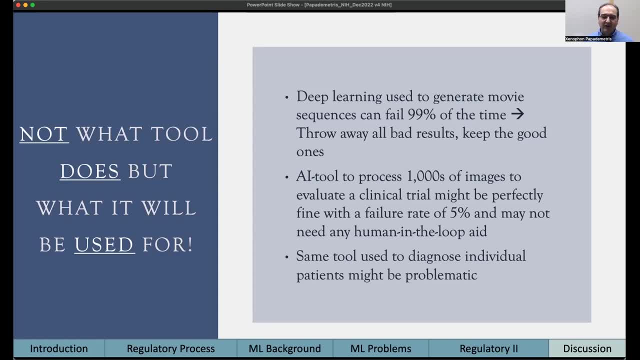 if you're using the same tool to diagnose individual patients, you may have a problem right? So it's what you will use it for. It may be the second algorithm that does two and three above the clinical trial of the individual patient. You trust it for one. 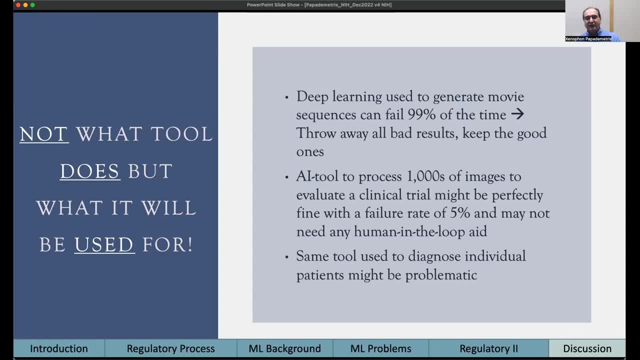 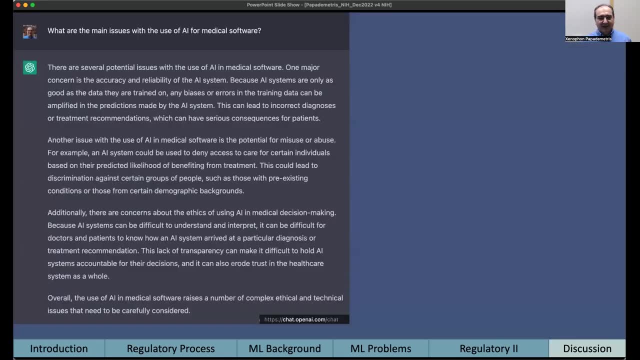 you don't trust it for the other. So it's not a question of can we trust AI, It's when can we trust it and when can we not. That is the question to keep in mind. So you've seen all these AI chart things. 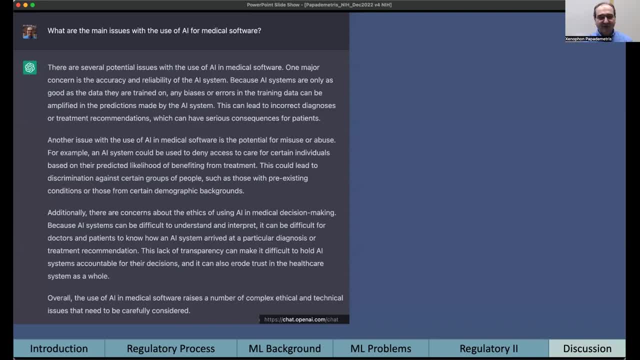 This is from ChartGPT, So I went ahead and asked what are the main issues of the use of AI for medical software, And it gives a very good answer. If my students gave me this, I might actually believe them. So that's now. I'm scared. 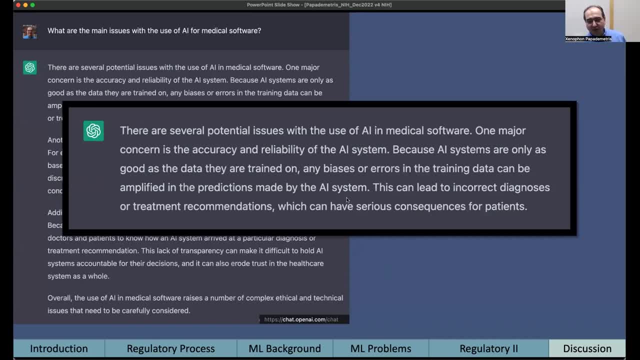 when it comes to teaching next semester. But what I want you to focus on is the statement here, Because AI systems are only as good as the data they're trained on. any biases or errors in the training data can be amplified in the prediction made by the AI system. 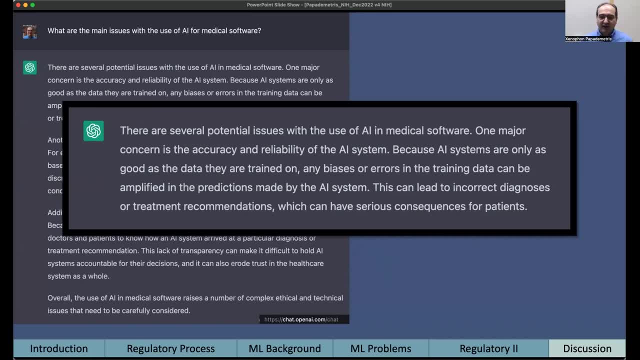 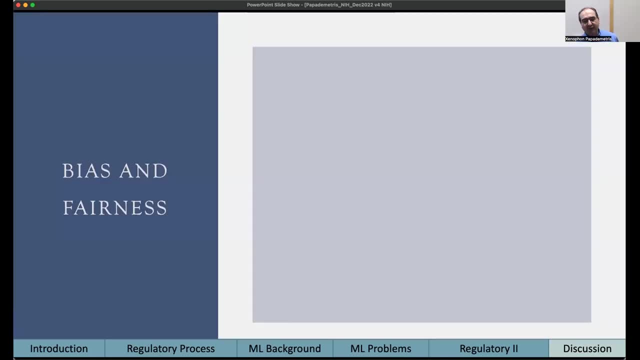 This can lead to incorrect diagnosis. Treatment recommendations can have serious consequences for patients, And this includes fundamental issues like bias, And so let's just touch on that briefly I, as I alluded to earlier in the talk. but let's just talk. 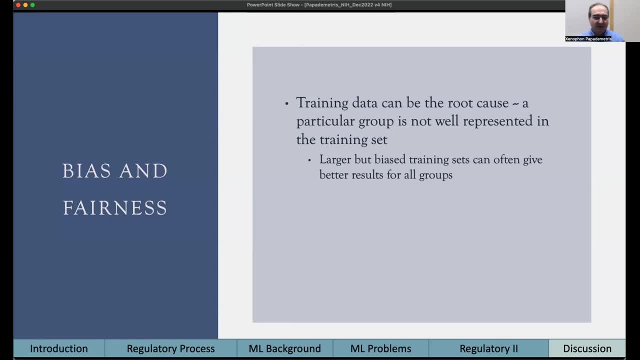 about it quickly. The training data can be the root cause for bias. A particular group may not be very well represented in the training set, So you get less accurate results there. This is not always the case. Sometimes a larger, but a biased training set. 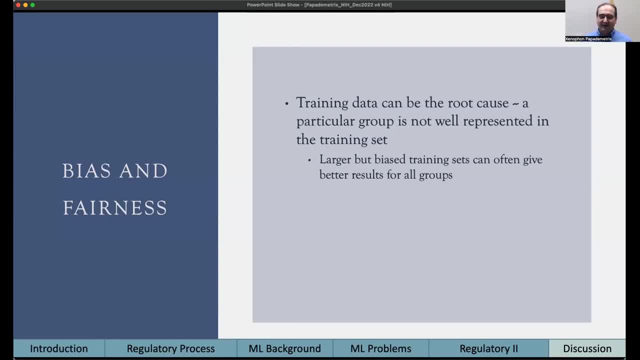 can give you better results for all groups than a more balanced training set, but that's smaller, So there is shared variance across groups And so sometimes a larger bias training set may be better for everybody. So that's just something to keep in mind. 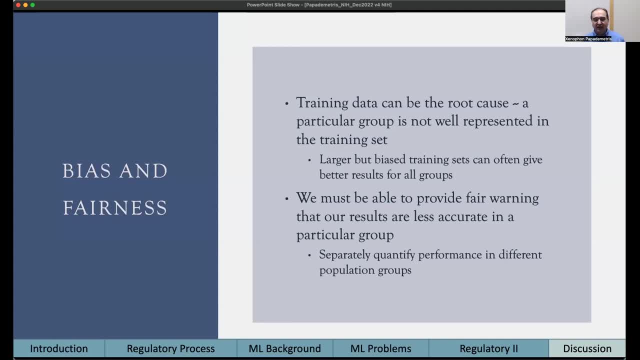 I think, to me at least, the key issue here is that we must be able to provide fair warning that our results are less accurate in a particular group, which means that we need to separately quantify performance in different population groups. We'll never be able. 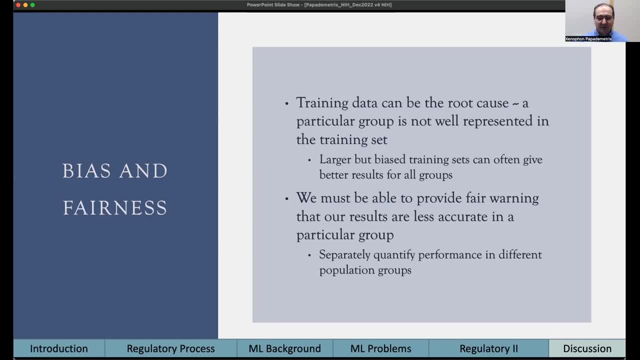 to do the same performance in everybody. Sometimes the anatomy of different people make it easier to diagnose a disease in another. skin color may make it easier to diagnose a particular skin disease in another, But at least we need to know whether this algorithm works differently in different groups. 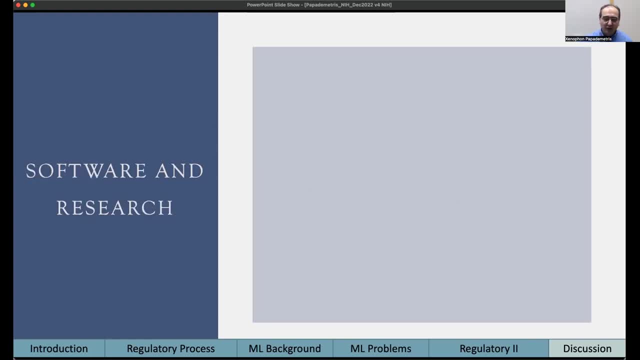 That's sort of my take here. Finally, you know we talked about AI, but let's think a little bit about software generically and research. Some of the issues involving AI apply to all software as well. AI is always really a component. 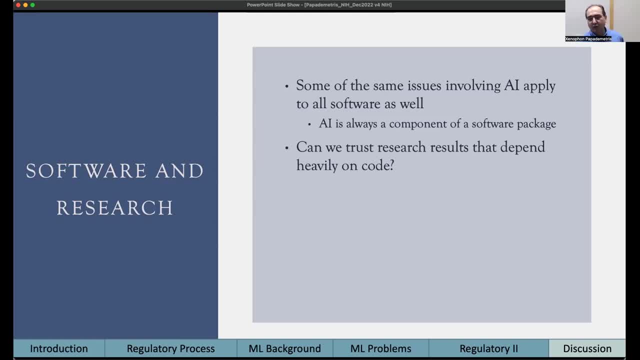 of a software package? Can we trust research results that depend heavily on code? What would you look for? So I would suggest that we don't just look at the results. We should ask questions like: who did the programming? How well trained were they? 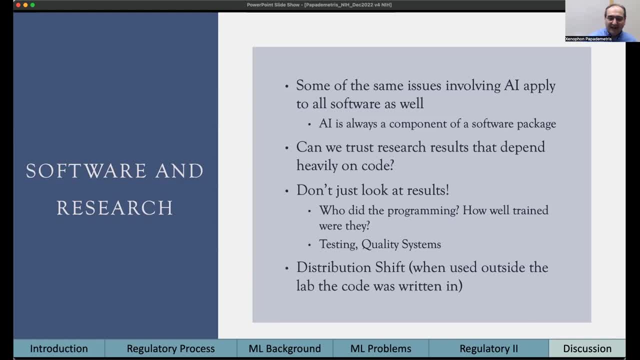 How well was the code tested? Did they have quality systems in place? Are they suffering from essentially the same thing in what we call an AI distribution shift? Did they take code from another lab? They used it on their own data and their own data. 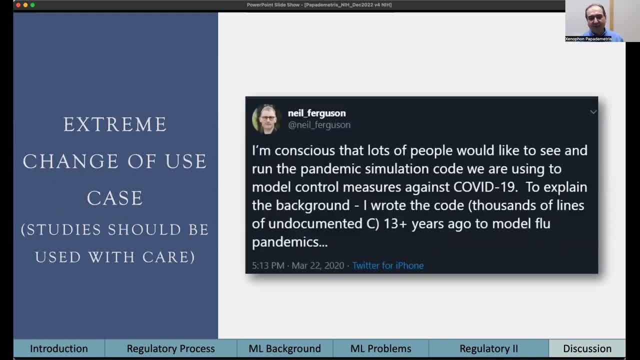 is slightly different and they trusted the results. So those are questions. So, as a final slide, just to highlight this change of use case, this is a tweet from Neil Ferguson of senior epidemiologist in London, And they were using some of his code. 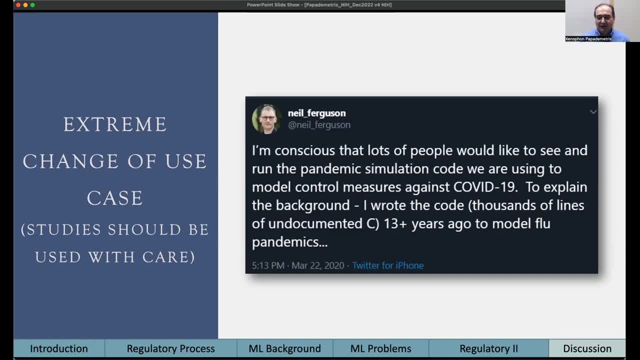 to predict how the different control measures for COVID would come out. The tweet is for March 22, 2020.. So you can tell that this is the first time that we've seen a study of COVID-19 in the US And at the time. 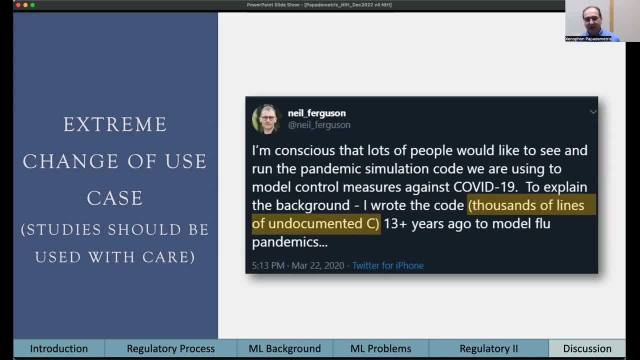 and this is in response to people wanting to look at the code that they were running- And he said: look. the reason this has been delayed is that I wrote this code and it's considered thousands of lines of undocumented sea 13 plants years ago. 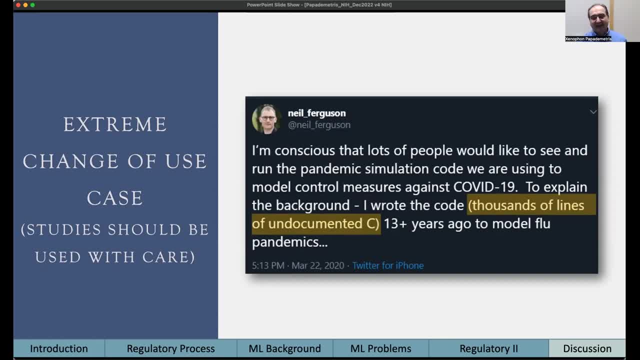 to model flu pandemic, So it's taking me a little bit more time to get it out to you Now. this code may have been perfectly fine as a modeling tool for research, but it requires more detailed documentation, So you can't just use code. 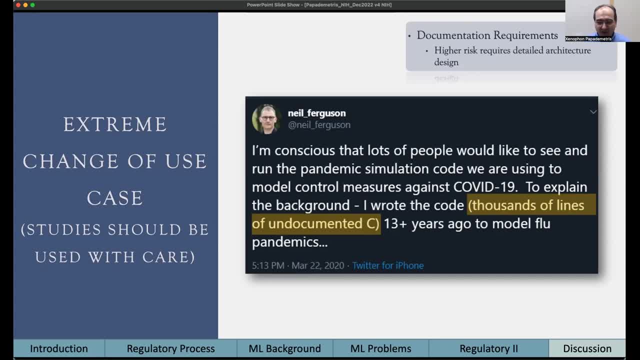 that was designed for one purpose for another purpose. It may be the same tool, It may superficially be the same purpose when modeling a pandemic, But the use of this code is very different. One is to teach, perhaps the other is to decide. 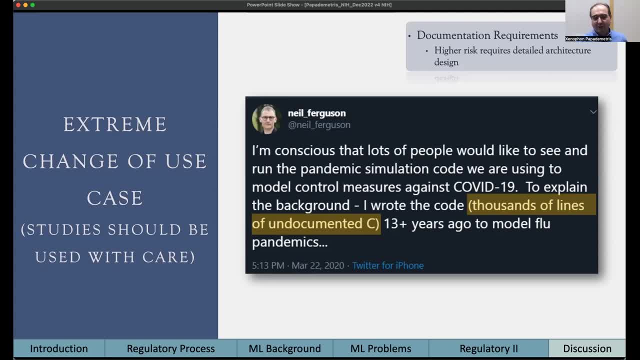 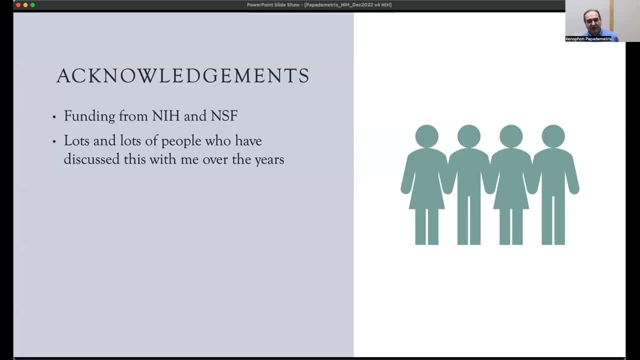 what you should do. So this was no criticism of what they did. In fact, that's not the issue of point of. With that, let me acknowledge funding here from the NIH and I'm- I'm not going to list all the people who have had many discussions. 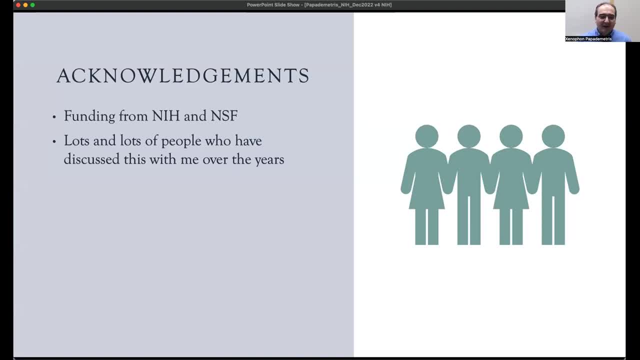 and many people. I'm worried I'm going to miss somebody and feel bad about it, But all the people who have practiced versions of this talk and these ideas for me over the years. I'd like to thank you all and we know who you are. 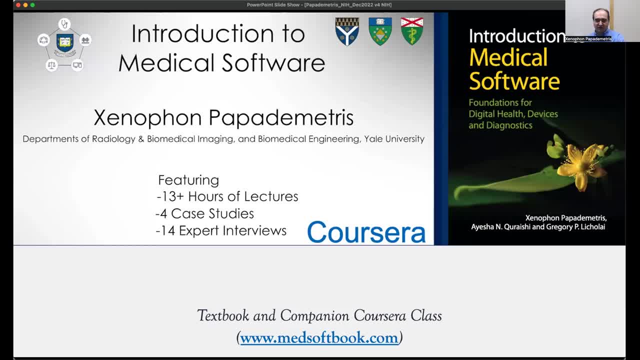 Finally, for those of you who want to know more on the medical software side of this research, there's an online Coursera class on medical software that you can take. The class is free, There's a small fee for the certificate and you can hear me talk. 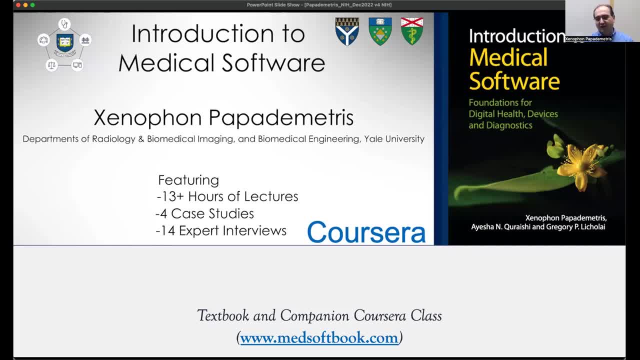 for many more hours. There's a companion textbook that I use for my own teaching. that was just made available. You can get more information at the link at the bottom: medsoftbookcom. And with that, Leonid, we'll stop here. and we'll take questions. 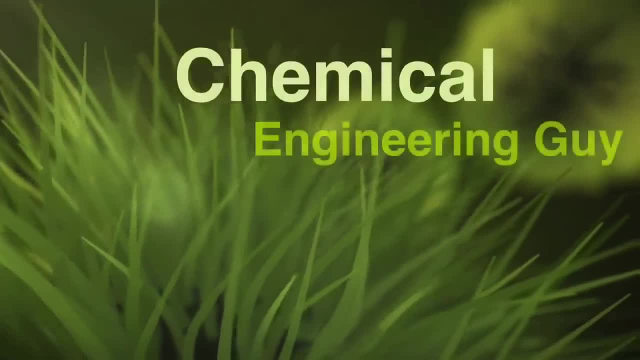 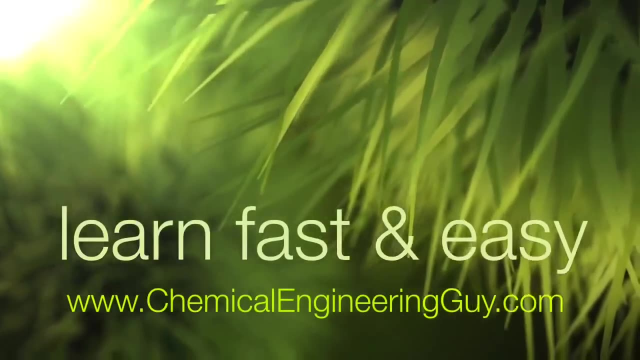 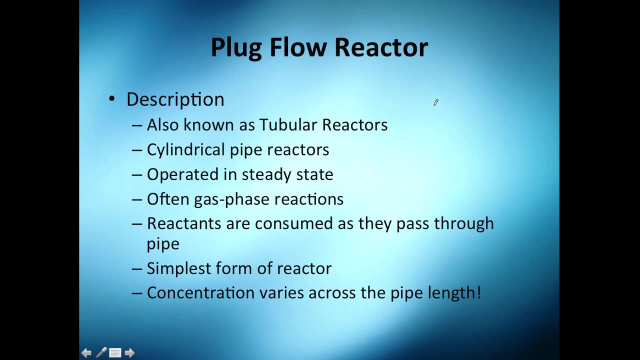 What's up, guys? now let's continue with this plug flow reactor. I'm going to give you a small description of what it is and how it's operated, and then we do a molar balance on it. So the description is essentially- you should know it also- as tubular reactors. Why tubular? 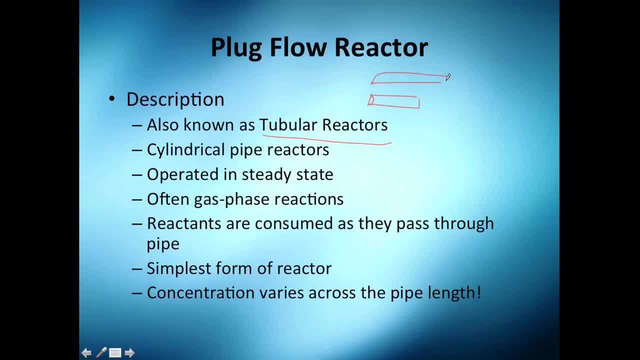 Because they are tubes or pipes. So this is the typical arrangement. they go like this. You're going to see more photos later. They are cylindrical pipe reactors. they are operated in steady state Makes sense, because you get inside stuff and you get the outlet here. It's often in. 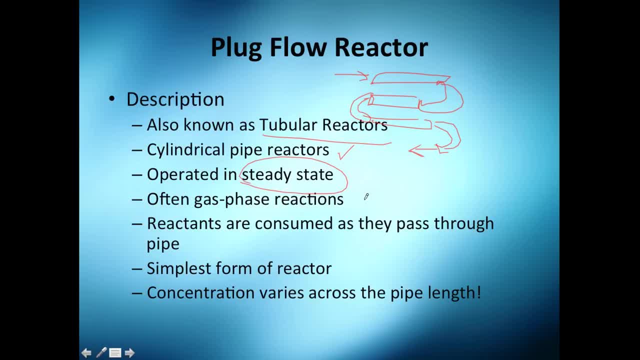 gas phase reactions, but you can do them also in liquid phase or gas-liquid. No, that's not that normal, actually just gas phase, or either gas phase or liquid phase. The reactants are consumed as they pass through. For example, you got A plus B. they start reacting. A plus B goes to C and as 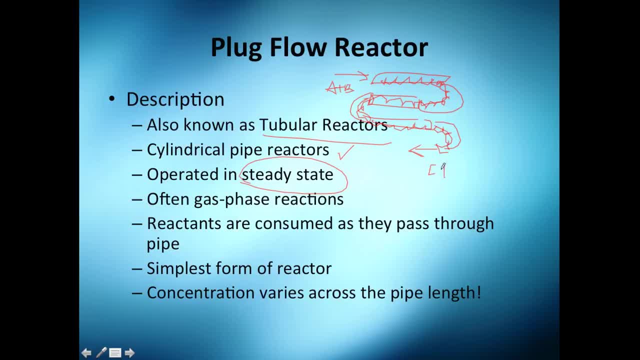 they pass through the pipe. they finish, I don't know, maybe a lot of C and not that much of A and B. The reactants are consumed. yeah, that's true, It's the simplest form of a reactor. I tell it because it's literally a pipe You don't need. 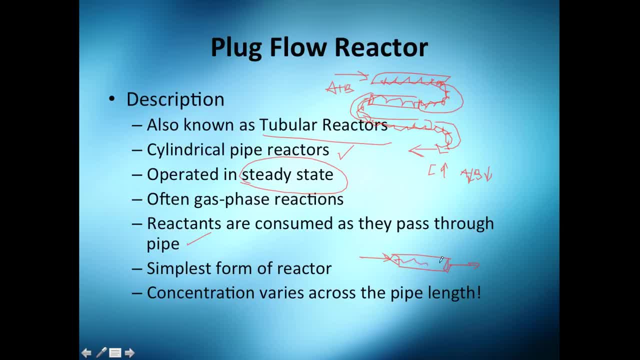 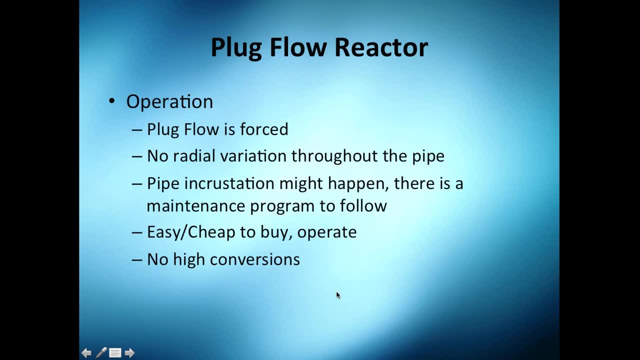 to do a tank or whatever. it's just a pipe. they mix because of the turbulence And yeah, essentially that's the thing. So let's continue how it's operated. It's operated with a plug flow. So, if you remember, plug flow means it has a lot of turbulence, A lot of turbulence.